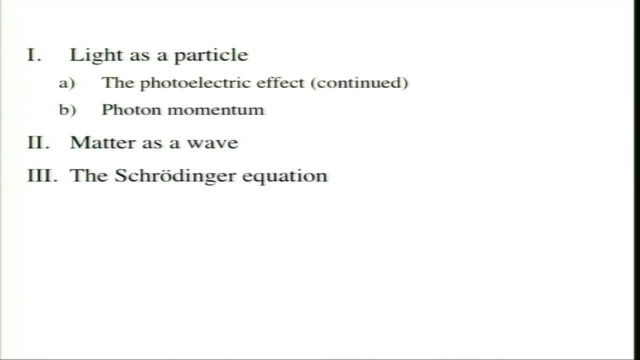 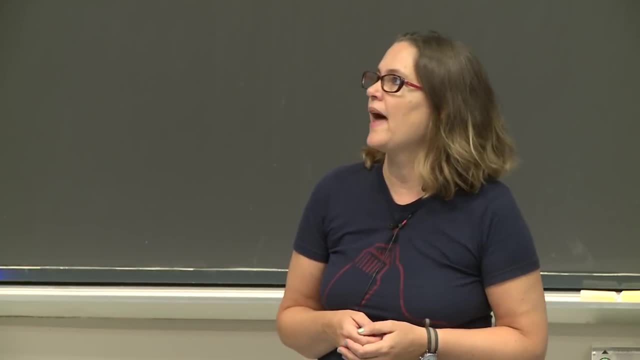 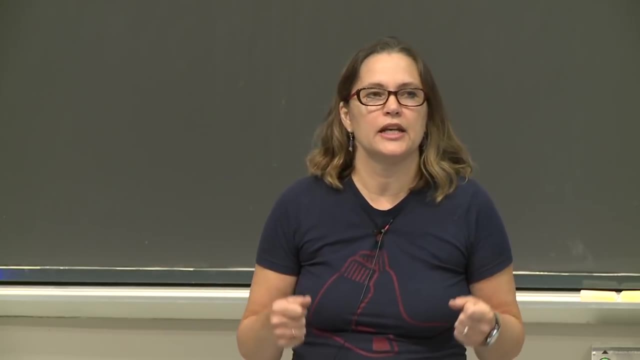 Then we're going to go on. If light is in fact quantized and you have these photons, then photons should have momentum, And so we'll talk about that. Then we've talked about light as a particle, And most of you are probably pretty OK. 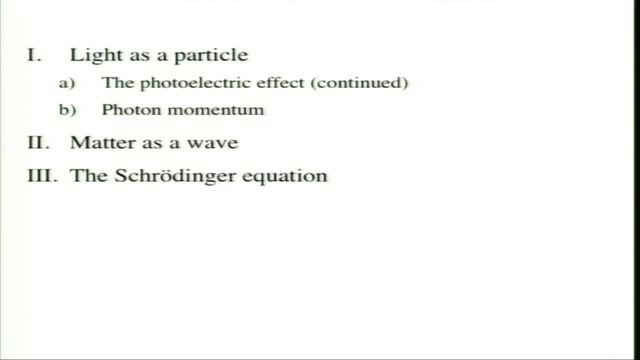 with matter being a particle, But what about matter being a wave? So we're going to talk about matter being a wave And, if we have time, At the end, we're going to start on the Schrodinger equation, which we're going to continue with on Friday. 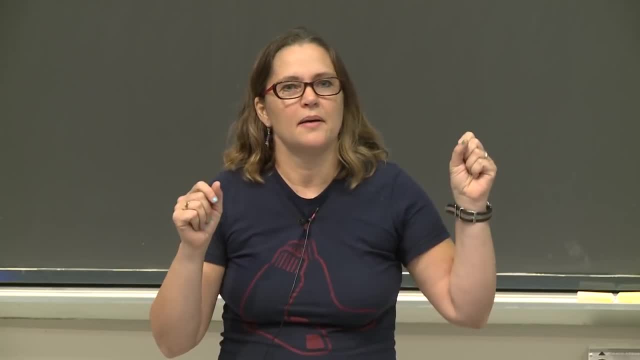 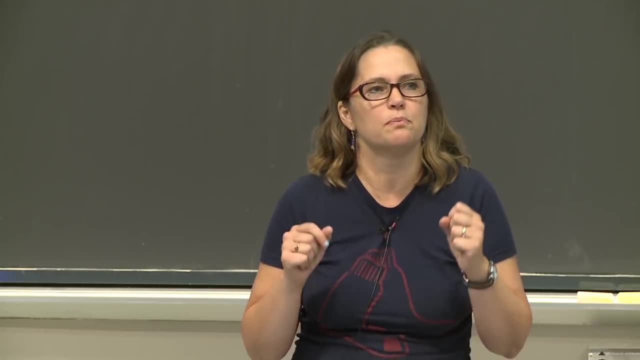 So I'll just say that sometimes I am a little overly ambitious And I put things on the handout that I'm not really sure I'm going to get to. Just because I've never gotten into it before doesn't mean that I won't get into it this time. 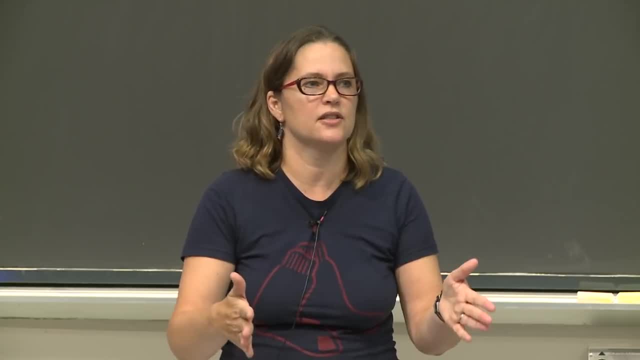 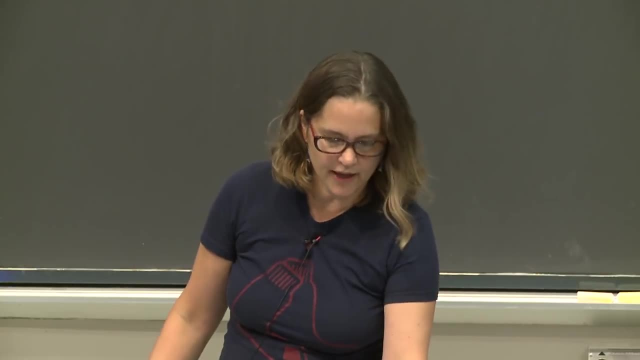 So if I don't finish everything on a handout, bring your handout to the next class And we'll just continue from there And there'll be a new handout then as well. So just a heads up on that, All right. 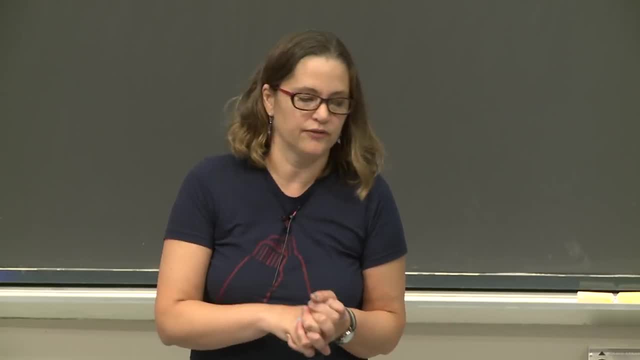 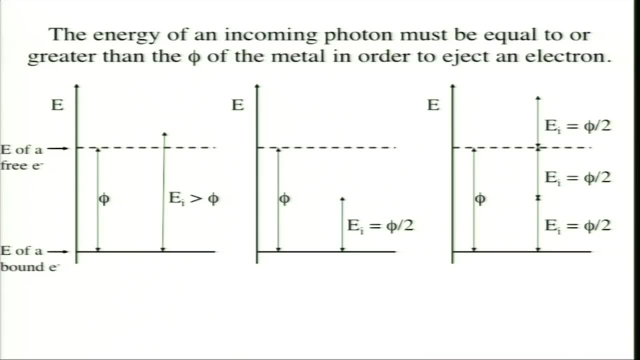 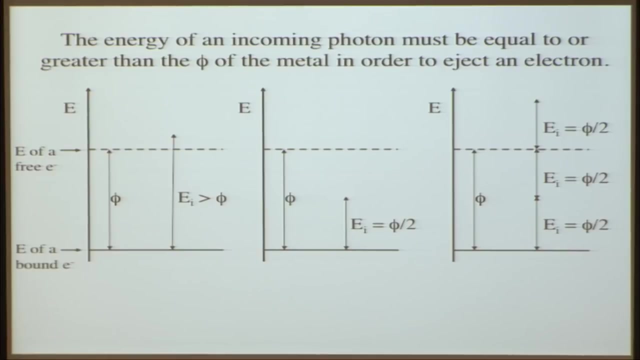 So let's continue with the photoelectric effect and get good at doing these kinds of problems. So let's look at these particular examples. We have three different examples here. We have: the energy of an incoming photon must be equal or greater to that threshold energy. 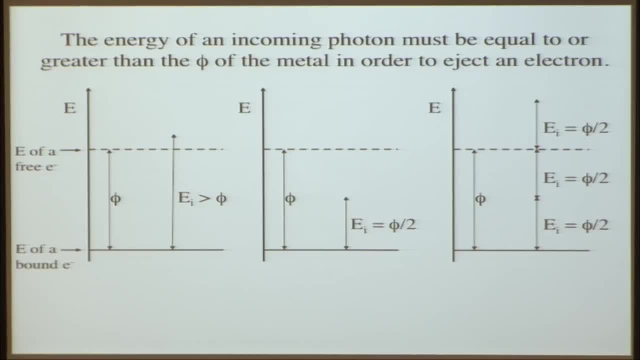 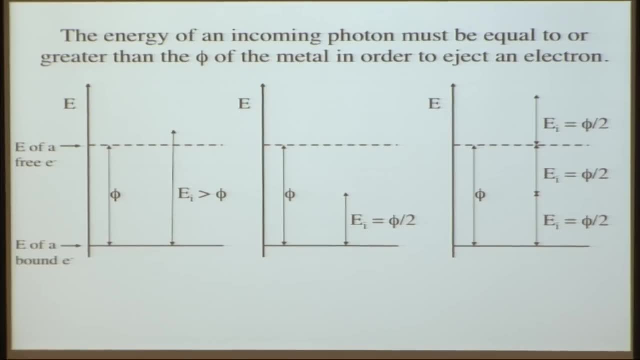 or that work function in order for an electron to be ejected. So in this case the energy is greater than the work function. So tell me whether an electron will be ejected or will not be ejected. You can just yell it out. What do you think? 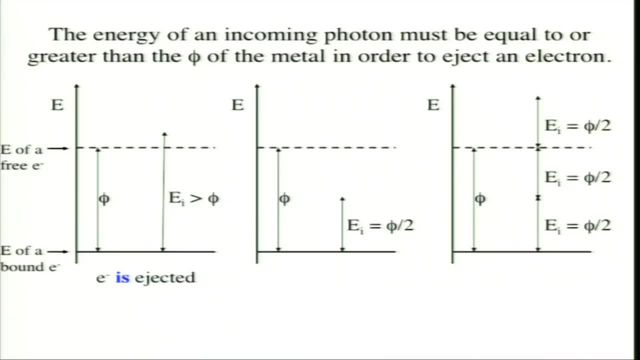 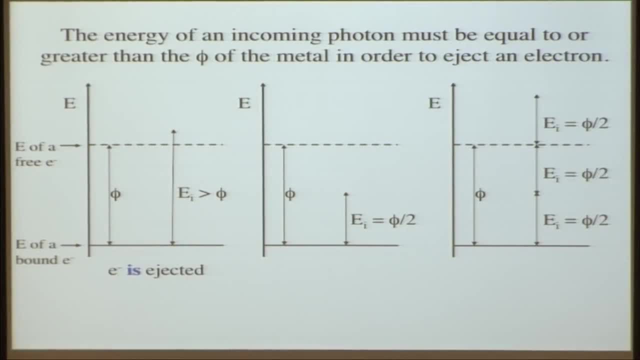 Will Yeah. So an electron is ejected, It will be ejected. What about this scenario over here, where the energy is less than that threshold? energy Is or is not ejected, Not Yes. OK, Now we have another scenario. We have three photons, each of which. 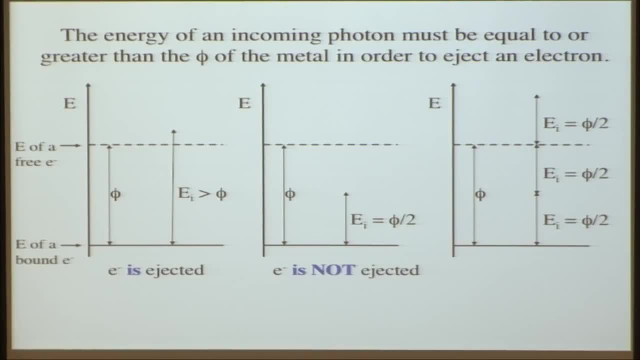 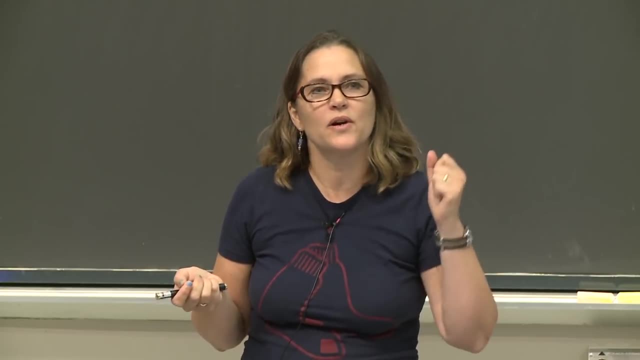 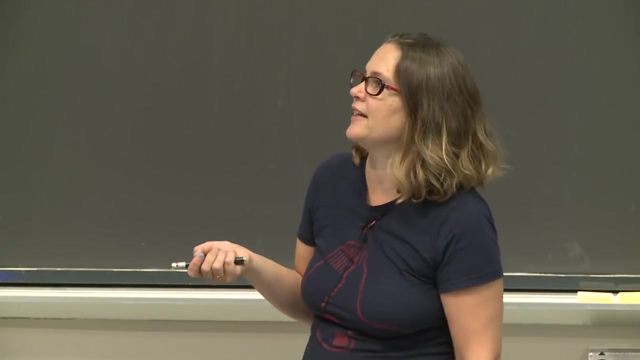 have half of the energy needed, half of that threshold energy, But you have three of them. So will an electron is or is not ejected? Not Is not OK. So three photons each that have half the energy does not add up. 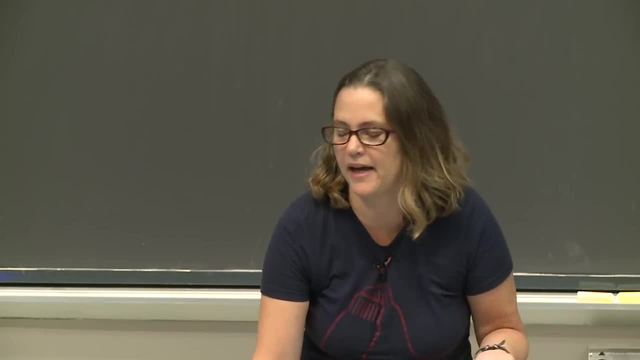 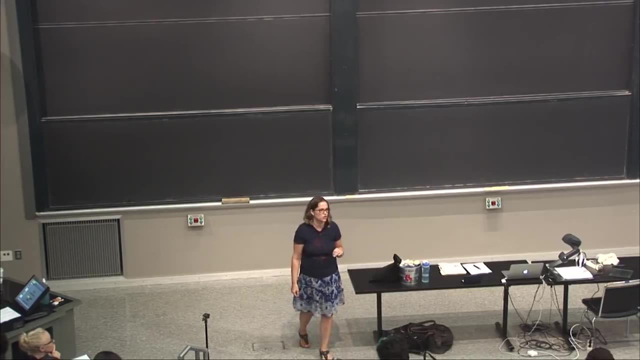 You cannot add it. It will not eject an electron. So let's just think about it for a minute. Suppose the threshold Knowledge for passing an exam is answering three specific questions correctly. Suppose over here we have the answer to one of the questions. 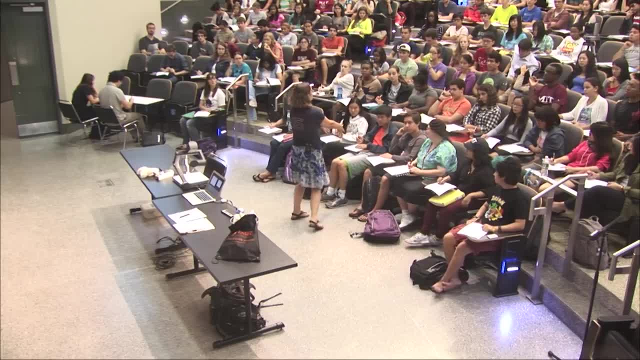 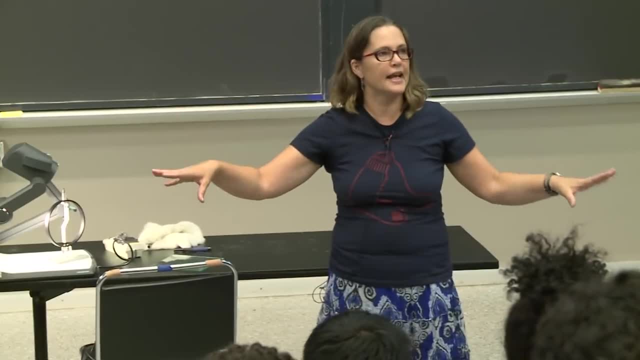 but not to the other two. Over here we have an answer to the middle one, but not the first or the second, And over here we have the answer to the third, but not the first or the second. So everyone knows the answer to a different question. 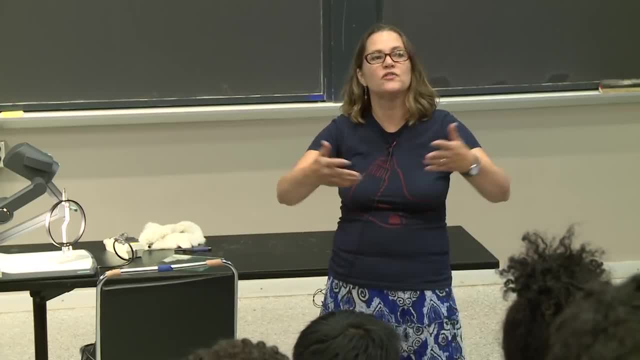 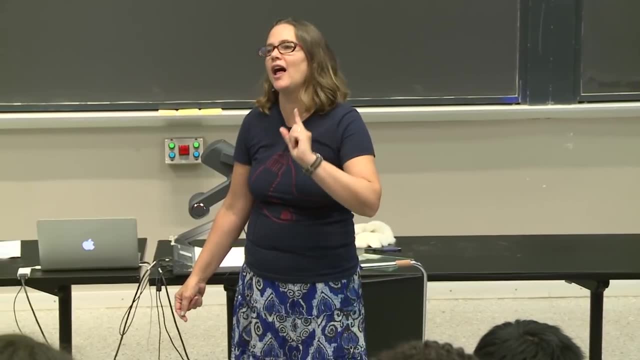 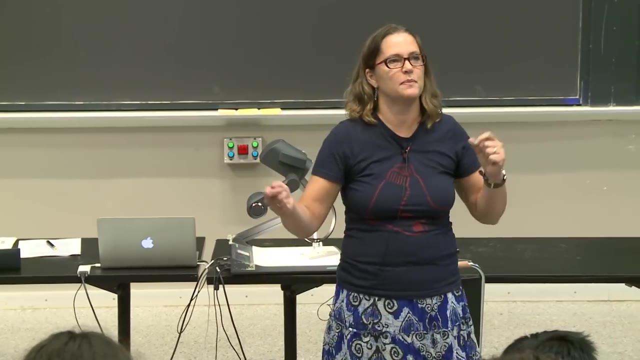 Will there be the threshold energy or threshold knowledge to pass this test? No, No, Everyone needs to have the threshold knowledge themselves to be able to pass. Everyone has to overcome that critical amount of knowledge to be able to pass the test. So that's the same thing here. 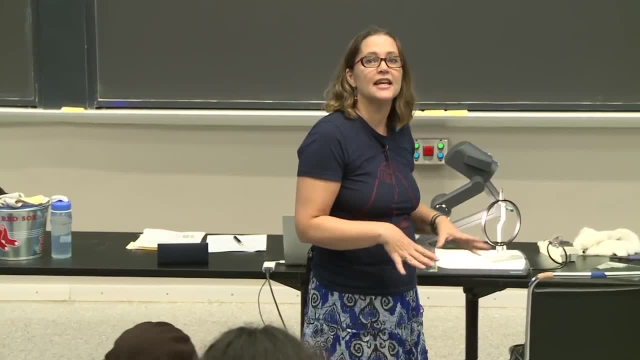 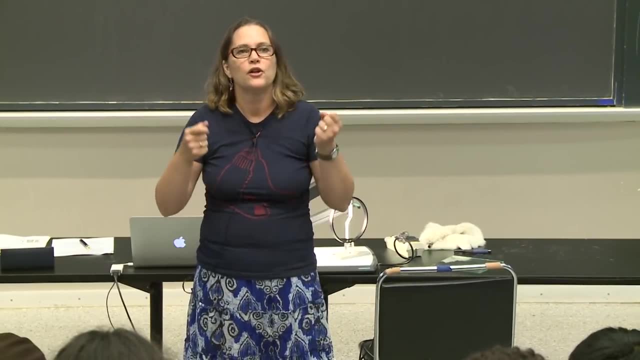 You can't add it up Now with the tests here at MIT. if everyone has that threshold knowledge and a really high level of the threshold knowledge, everyone can get an A. So the more people with the threshold knowledge, the more tests that are passed and the more the course. 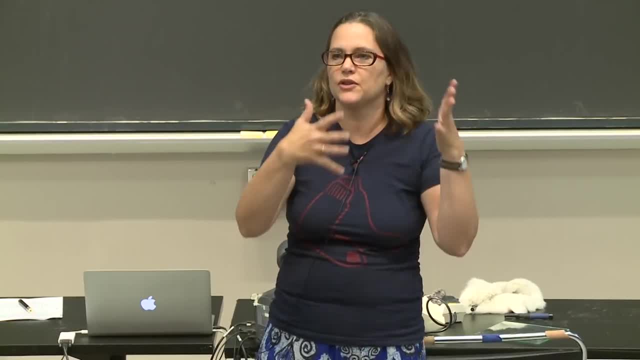 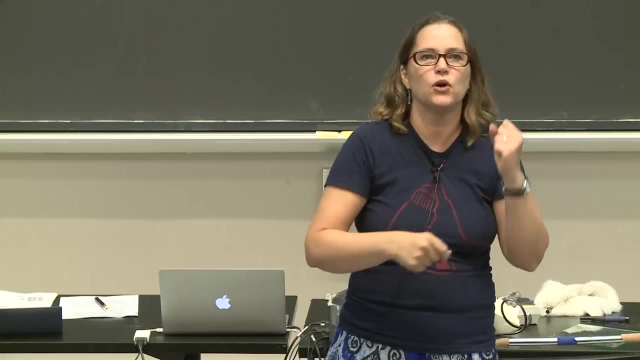 is passed by people. So the more photons coming in with that threshold energy, the more electrons being ejected. But you can't add up If you have photons that don't have enough, if they're not greater than the threshold energy, you won't eject an electron. 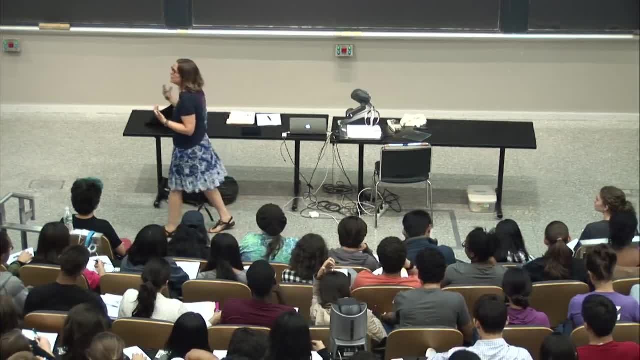 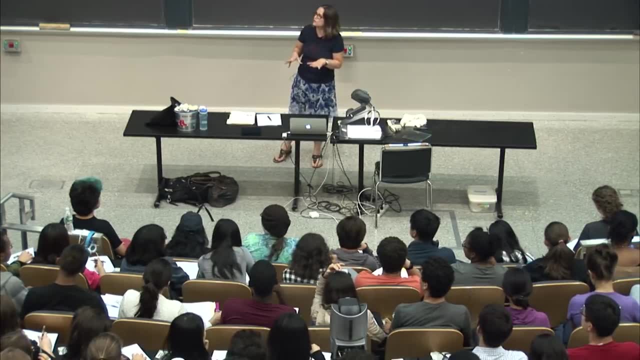 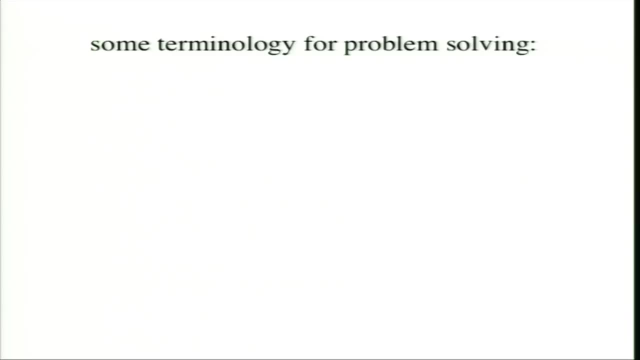 So everyone needs to meet that threshold criteria. You can't add things up, OK. So here's just some kind of useful stuff. There's useful terminology for solving problems on this problem set. and there will also be problems on problem set two related to this topic. 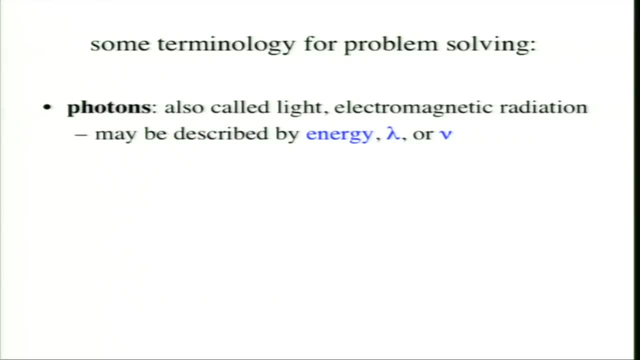 So photons, also called light, also called electromagnetic radiation, may be described by their energy, by their wavelength or by their frequency, Whereas electrons, which are sometimes also called photoelectrons, may be described by their kinetic energy, Their velocity and, as you'll see later, by their wavelength. 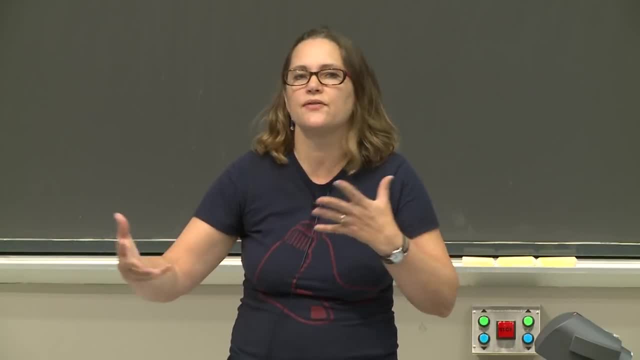 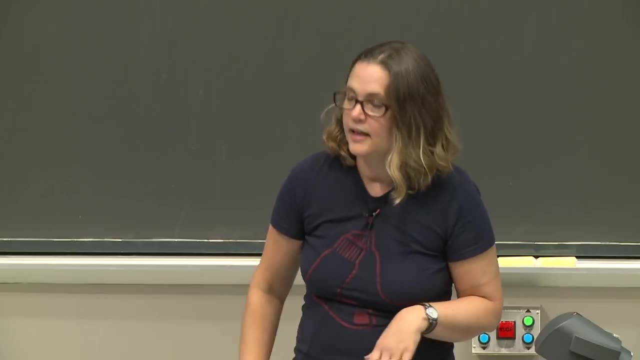 So you'll be given problems where you're given different pieces of information. You have to think about how you're going to convert it. You've got to think about: am I talking about a photon, Am I talking about an electron? And you also want to think about units. 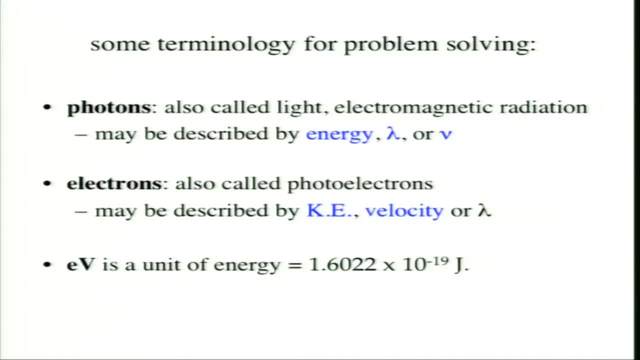 You'll sometimes be told about energy in EVs and sometimes be told about energies in joules. So this is a conversion factor. All conversion factors are different. The conversion factors are given to you on the exam. You do not need to memorize any kind of conversion factor. 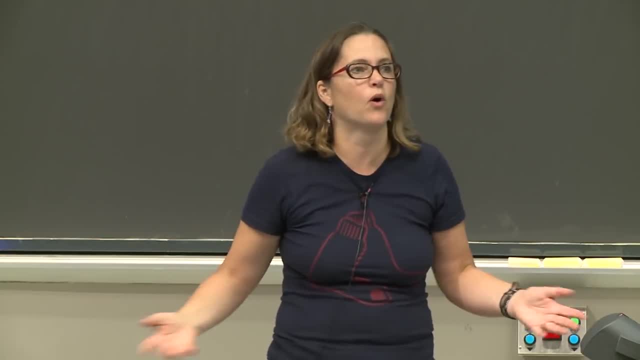 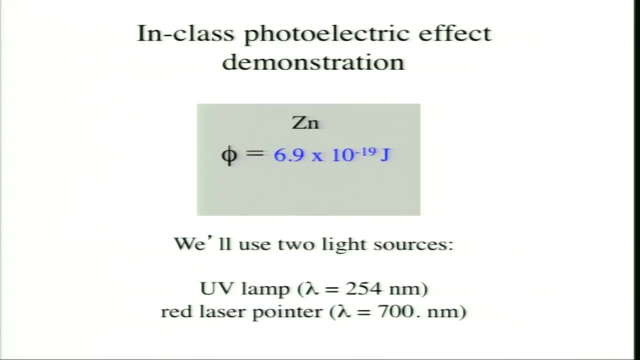 but you need to be aware when someone and you said: joules, what's that a unit for? Or EV, what's that a unit for? All right, so now we're going to do an in-class demonstration of the photoelectric effect. 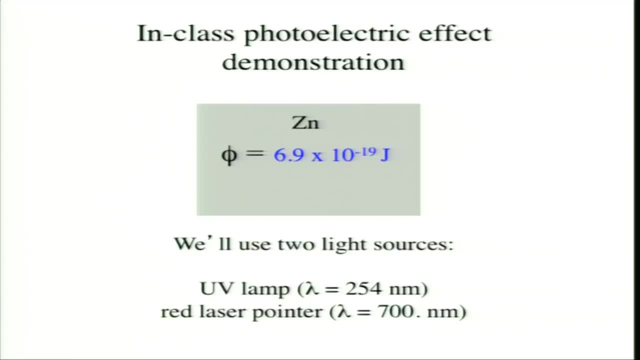 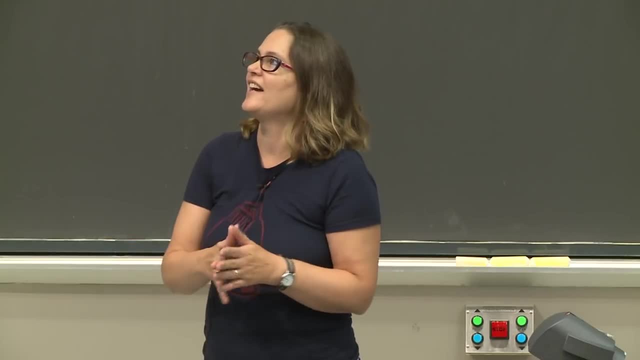 But before we actually do the experiment, we're going to predict what the experiment will show. Always dangerous to do that, so we'll hope it works after we do the prediction. All right, so we're going to be looking at whether we're. 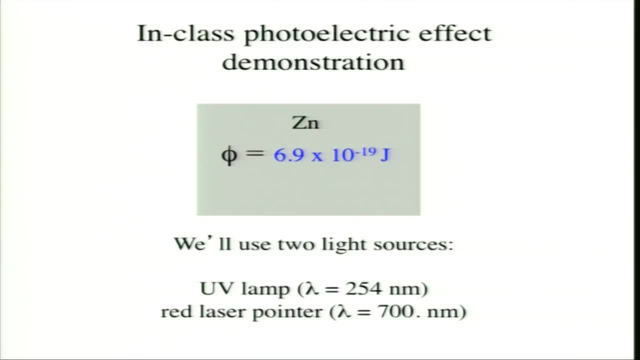 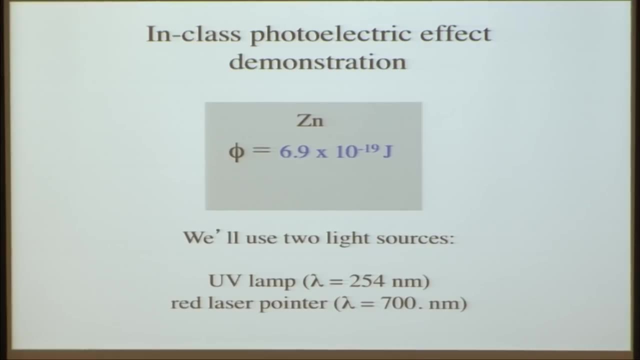 going to get an ejection of an electron from a zinc surface And we're given the threshold energy or the work function of zinc. Every metal, this is a property of metals. They're different, as we saw last time. So this is 6.9 times 10 to the minus 19th joules. 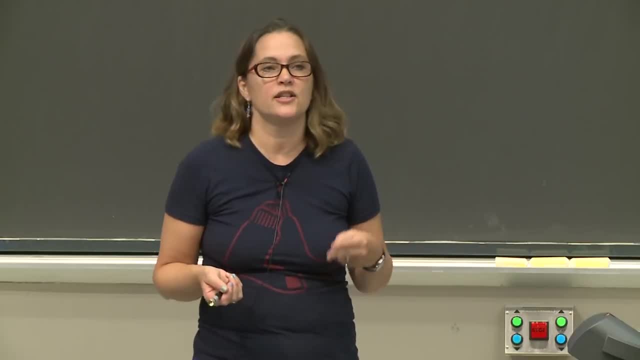 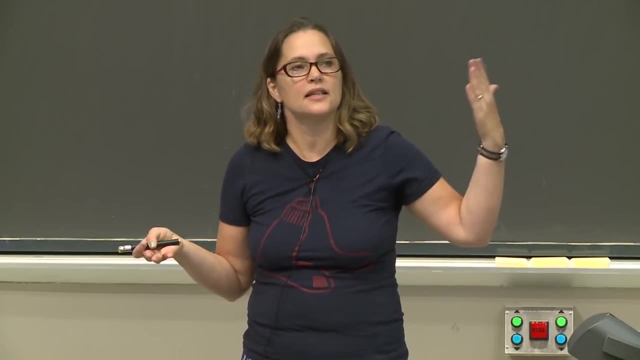 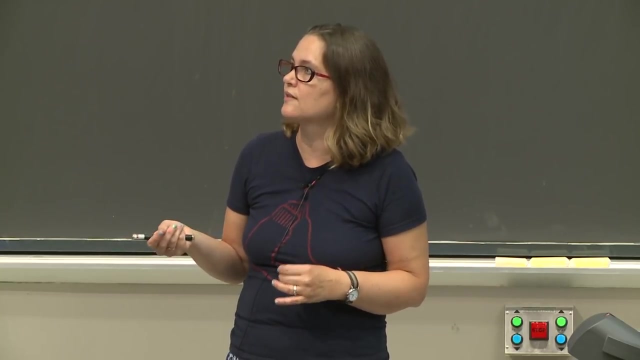 And we're going to use two different light sources that are going to have different wavelengths And we'll predict whether they have enough energy to meet this threshold, to go over the threshold and inject an electron. So the two different sources: we have a UV lamp with a wavelength of 254 nanometers and a red laser. 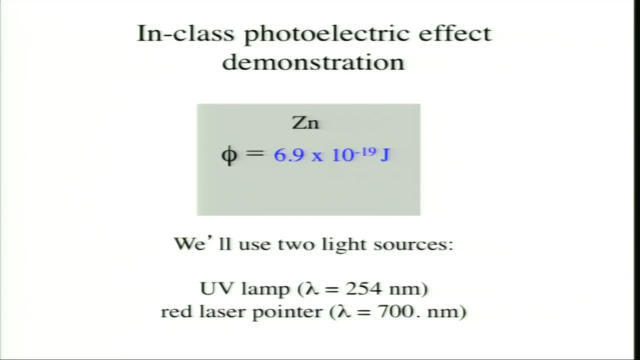 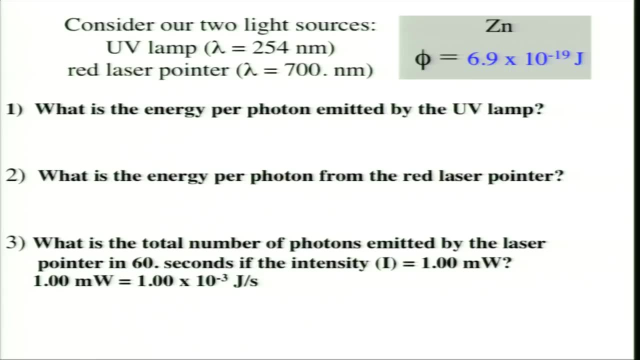 pointer with a wavelength of about 700 nanometers. So before we do the experiment, let's do some calculations to see what we expect. So first we want to see what the energy, or calculate what the energy of the photon will be that's emitted by the UV lamp. 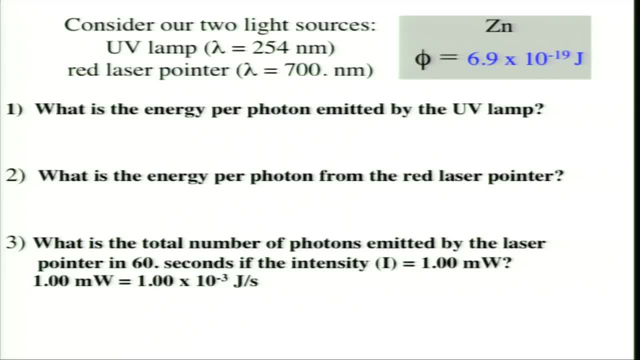 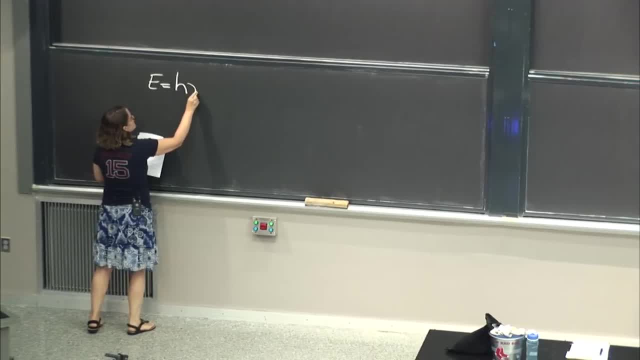 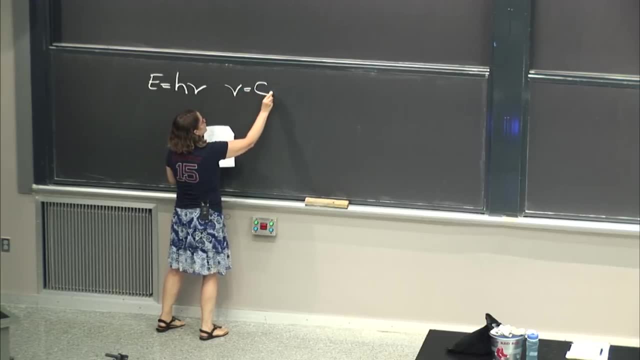 And I will write this down. So what do we know? We know a bunch of things already. We know that energy is equal to Planck's constant times, the frequency. We also know that the frequency is related to wavelength by c, the speed of light. 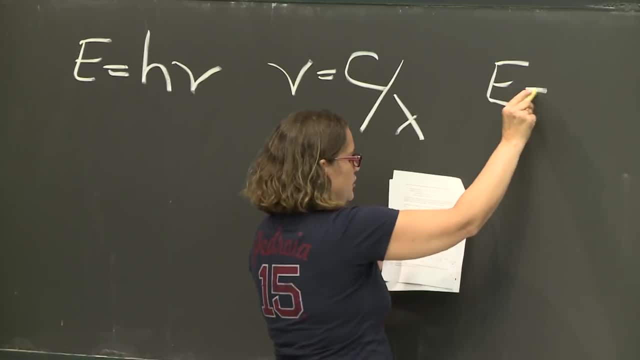 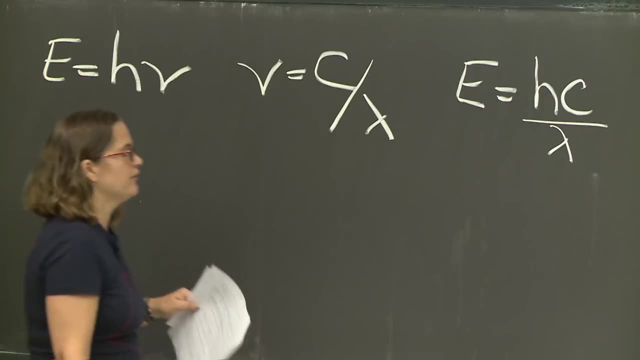 And then we can put those two things together to say: the energy then is also the Planck's constant times, the speed of light divided by the wavelength. So we can use that last equation to do a calculation and figure out the energy that's associated with that particular wavelength of light. 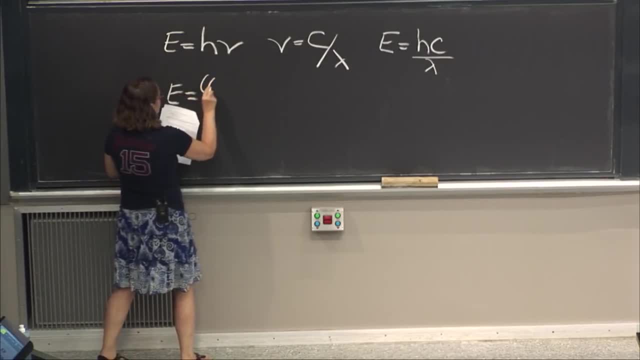 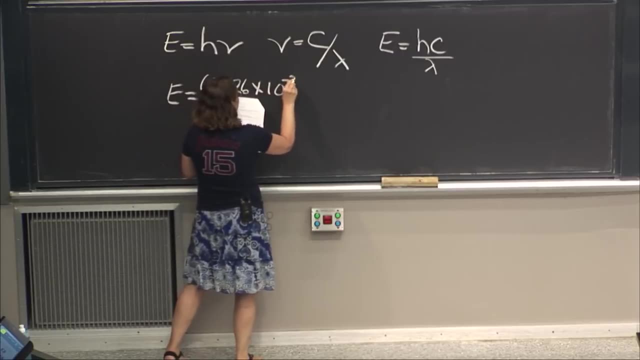 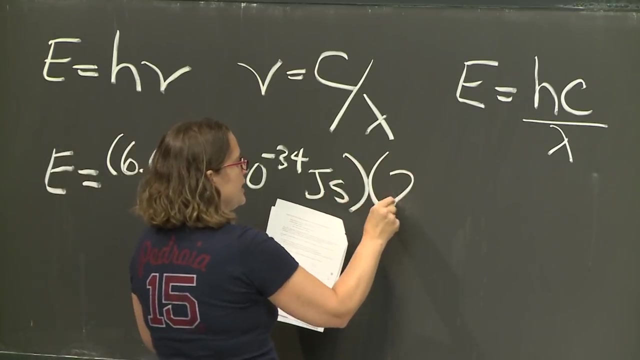 So here we have energy. We're going to write in Planck's constant: 6.626 times 10 to the minus 34.. And the units are joules times seconds And the speed of light, 2.998 times 10. 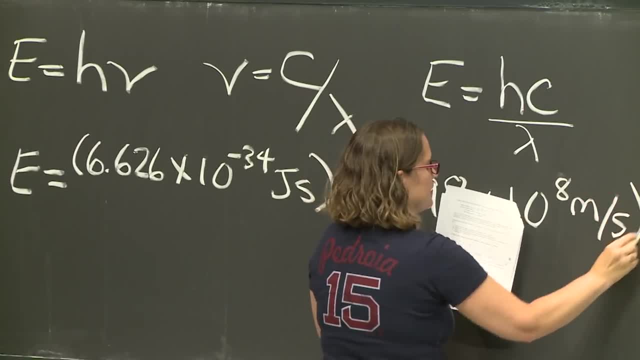 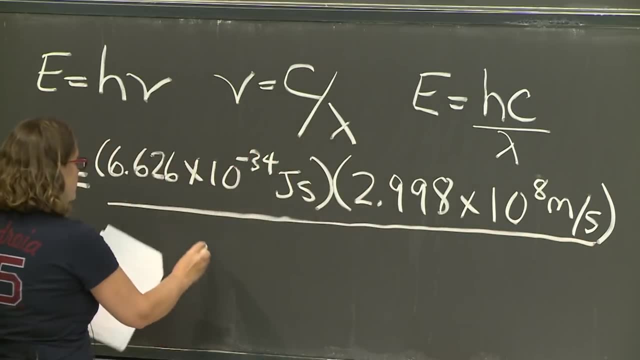 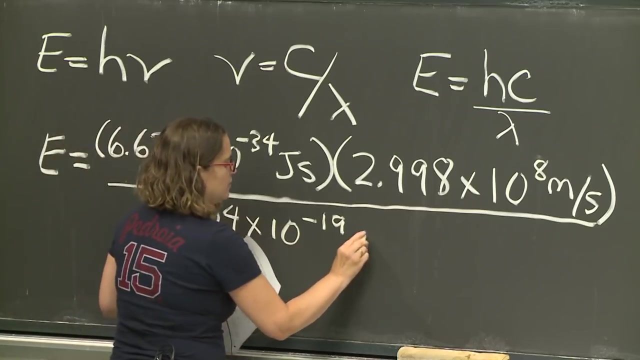 to the 8 meters per second, And we want to divide this then by the wavelength, So we have the wavelength here that we're using first is 254 times 10 to the minus 19 meters. Oh sorry, 9 meters. 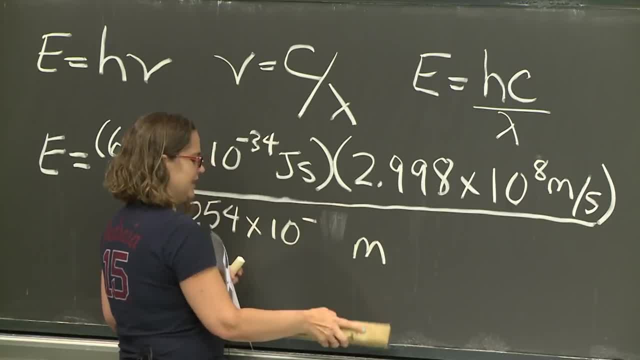 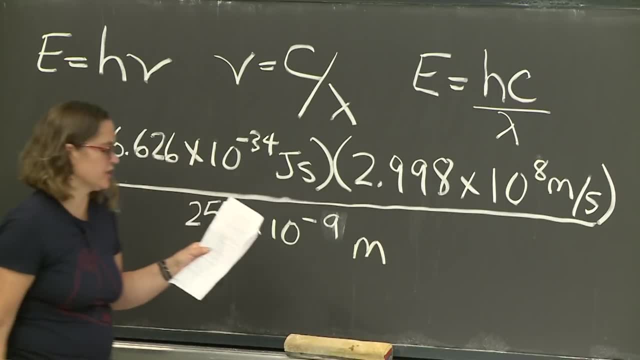 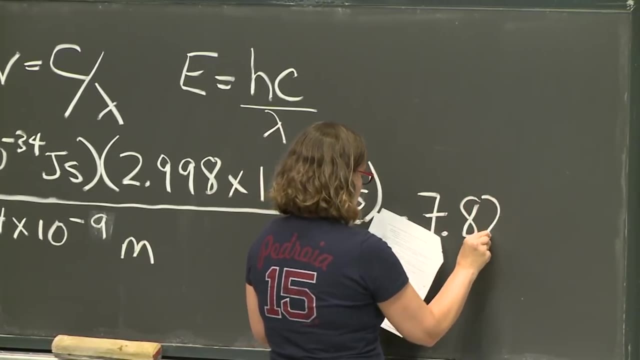 Thank you, I wrote down 19.. I'm like wait a minute, That's not right, OK, OK, OK. So then we can do the calculation out, And here is where I got excited about 19.. We have 7.82 times 10 to the minus 19 joules. 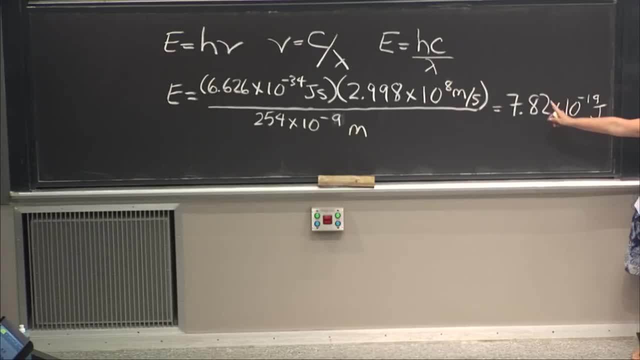 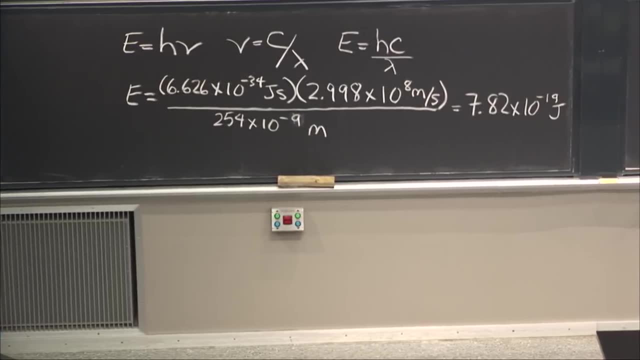 And if we look at the equation, we'll see that the meters are going to cancel, The seconds cancel and we're left with joules, which is good because we want an energy, So joules is a good thing to have. So there we can do a simple calculation. 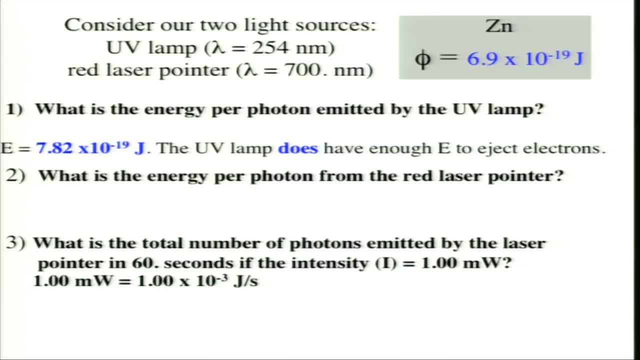 And we can look and say OK. if the energy then associated with that wavelength is 7.82 times 10 to the minus 19 joules, then we ask: is this greater or less than the threshold energy? And it's greater than that. 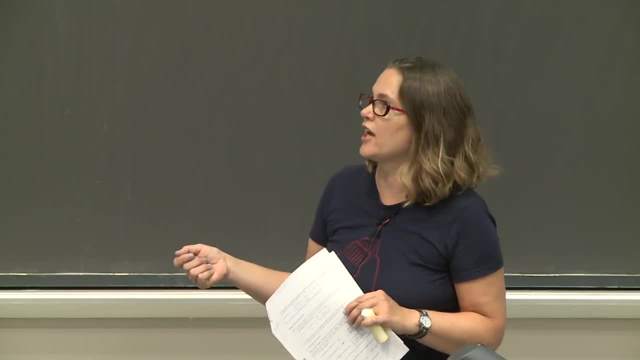 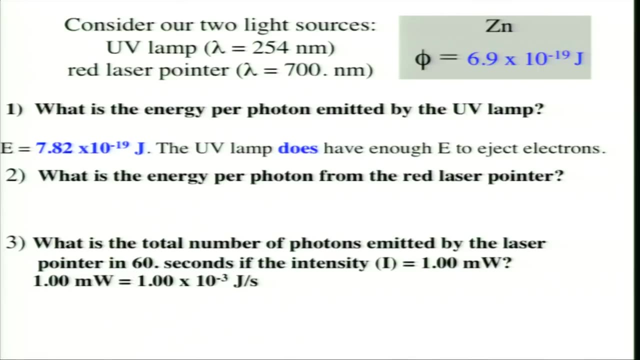 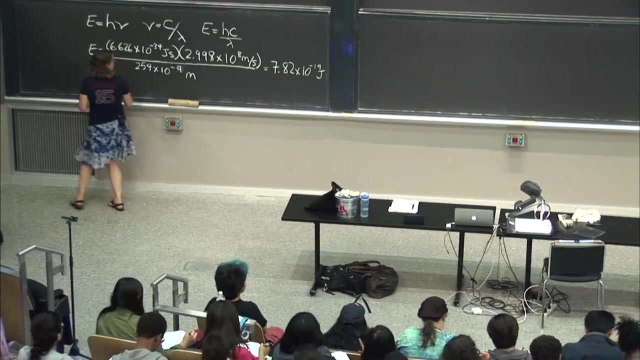 So it does have enough energy. It should eject an electron. So we can try that out and see. Now we can look at what happens with the red laser pointer and see whether that should have the energy that's needed, And so I will just write these things down here. 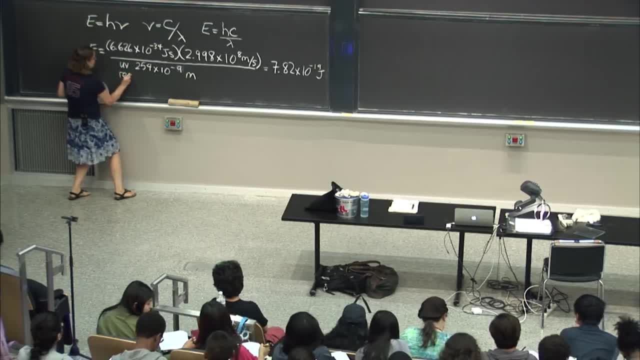 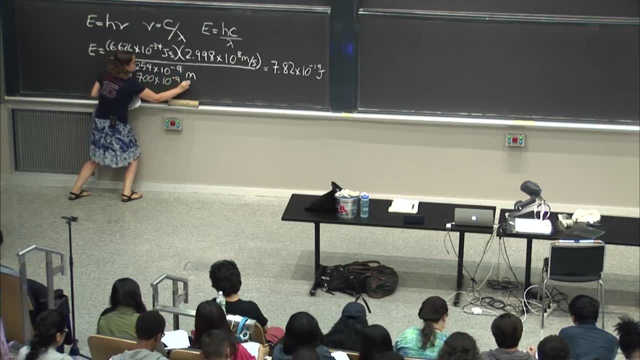 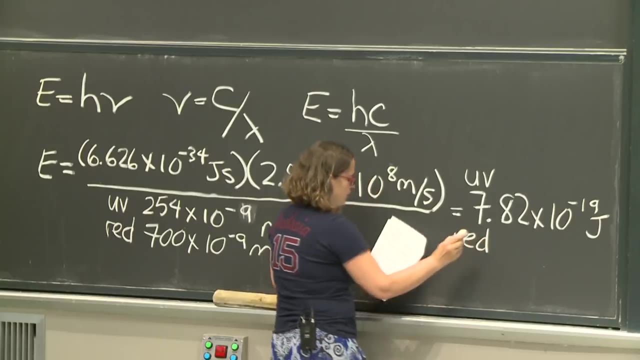 instead of writing it again. So that was our UV, So now our red light. we have 700 times 10 to the minus 9 meters, or 700 nanometers, And so here is our answer for the UV, And our answer for the red light should be 2.84.. 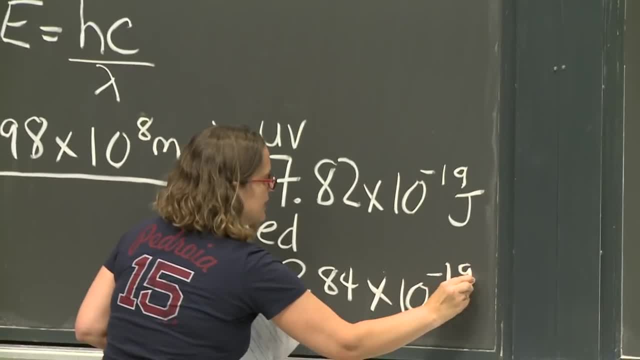 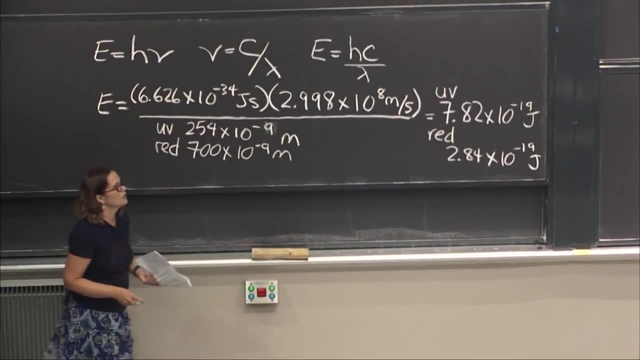 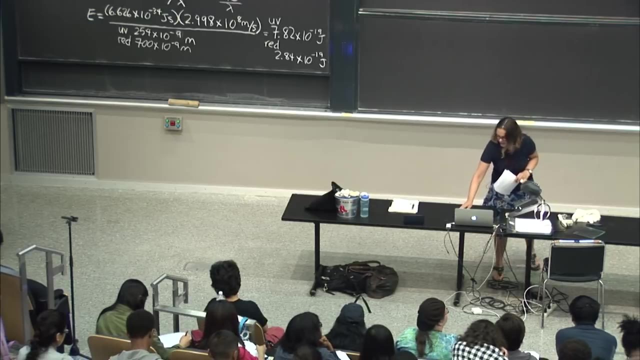 4 times 10 to the minus 19 joules, And I'll move this up a little so people can see that. So does that have enough energy to eject an electron? No, that should not work because that's less than the threshold energy that's needed. 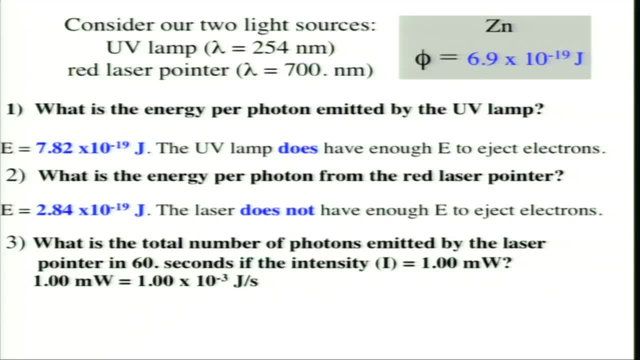 All right, so we'll do one more calculation just for fun, And then we'll do the experiment. So the last calculation we'll do is we'll think about the number of photons that are emitted by a laser in 60 seconds if you have an intensity of 1 milliwatt. 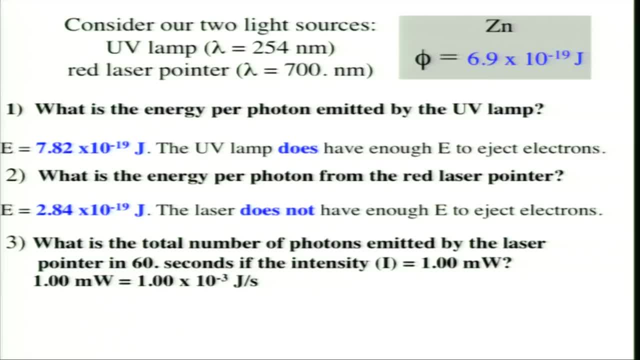 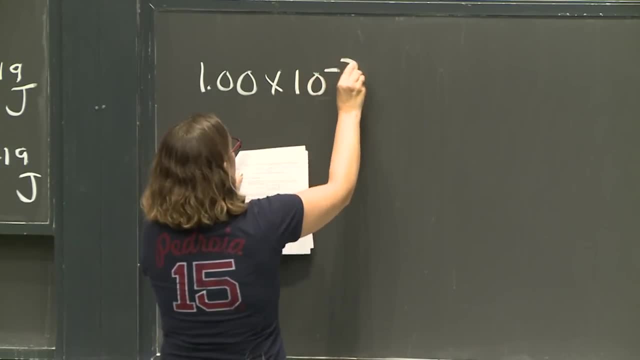 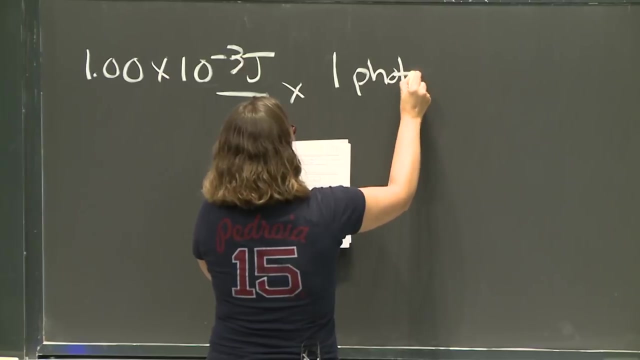 And milliwatt is equal to 10 to the minus 3 joules per second. So we can just do that calculation over here. So we have 1.00.. 0 times 10 to the minus 3 joules per second. 1 photon. 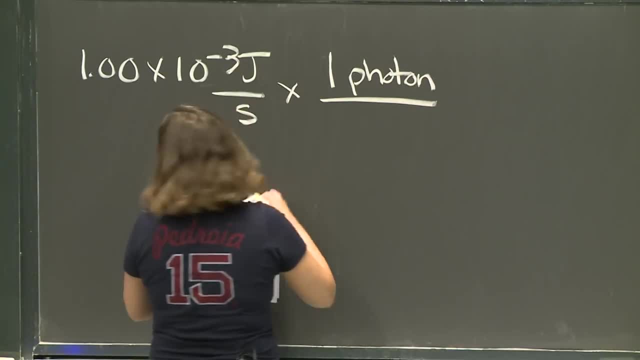 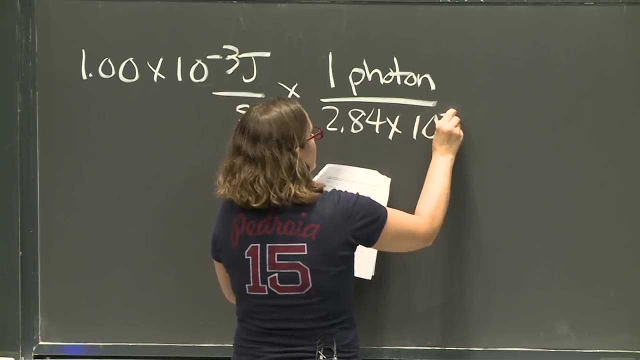 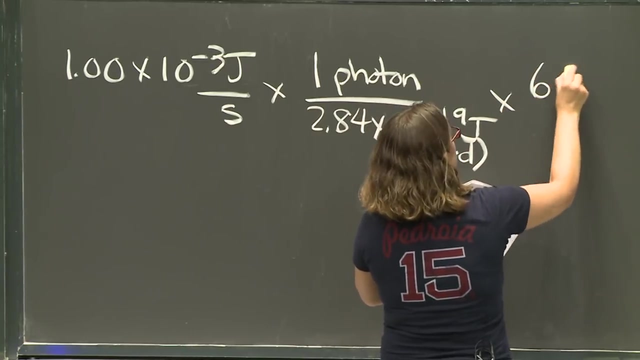 And here this is for the red laser, So we'll use the number that we just calculated over here. So we have 2.84 times 10 to the minus 19 joules for the red laser and times 60 seconds 0.00.. 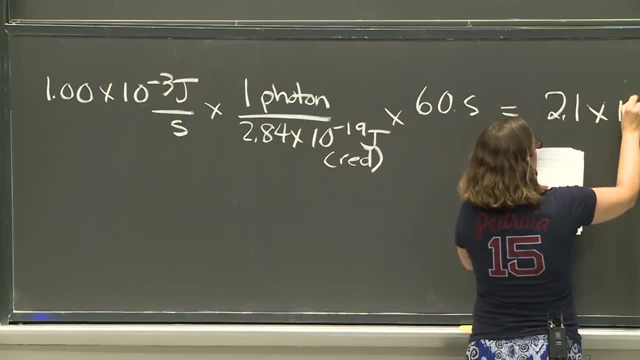 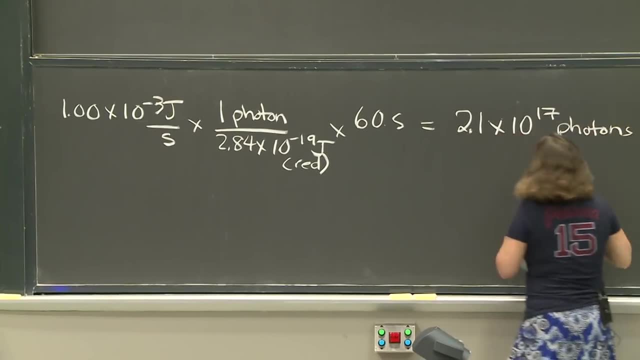 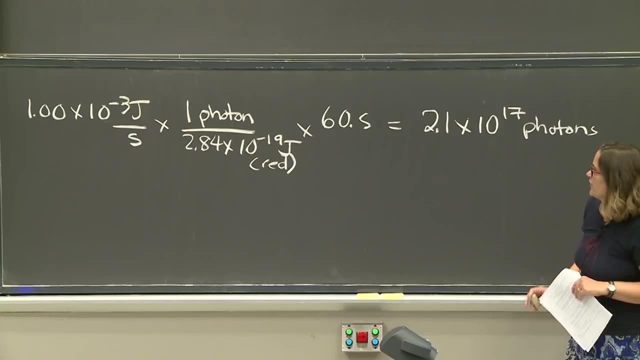 0.00.. 0.00. And we should get 2.1 times 10 to the 17 photons. So that's how much photons if we hold it for 60 seconds, that we're going to be shooting at our metal surface. 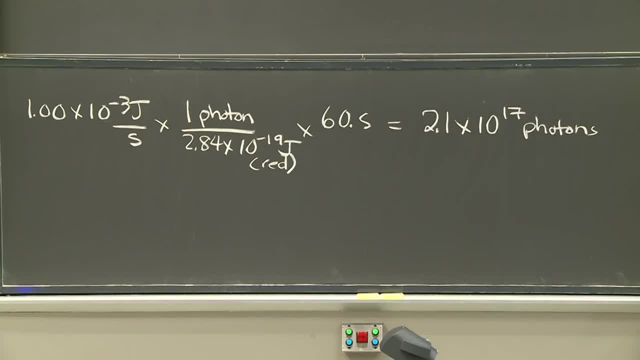 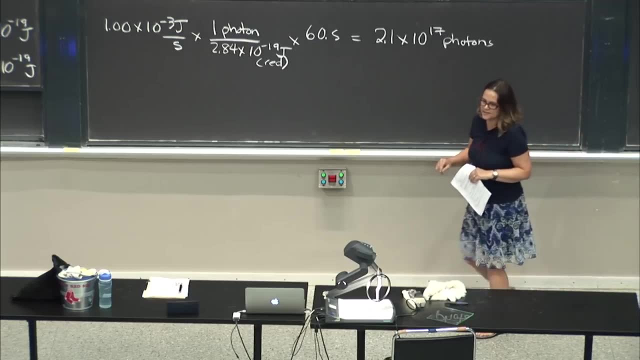 So these are the kind of calculations that you'll be doing on these kind of problems, And now let's see how well the experiment works. So we're going to bring out our demo TAs, who are going to tell you about this demo, and we're going to try to do. 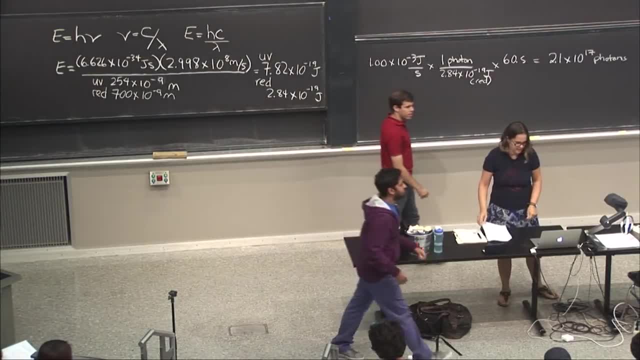 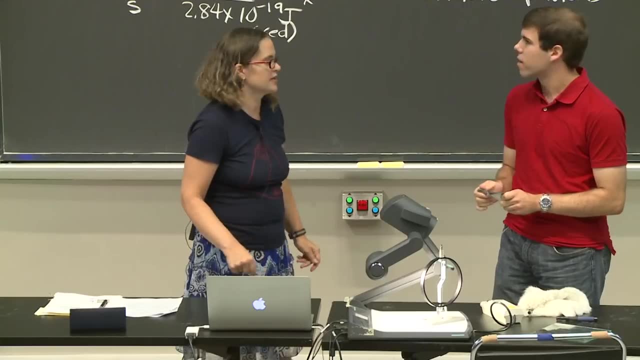 some fancy stuff with this document camera to project it on the screen. So this is all very exciting. Oh, I guess I should put that down, the number, in case you couldn't see it: 2.1 times 10 to the 17.. 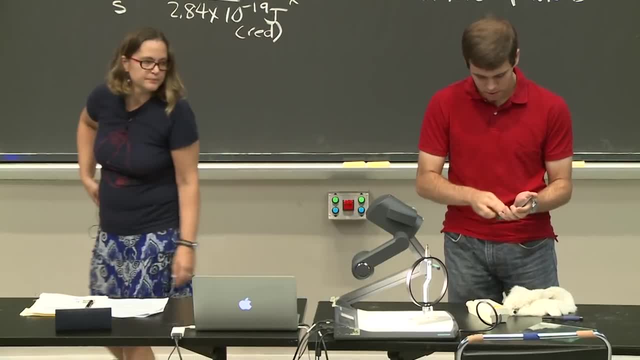 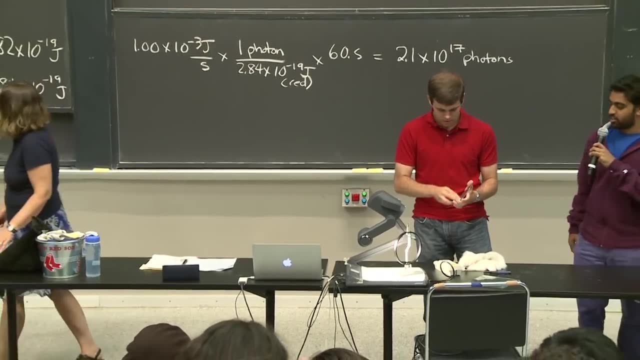 All right. So let's bring. you got the mic, OK. So we've got our metal plate here, that Eric's got in his hand, And what he's doing right now is he's rubbing it with a little bit of. what is that actually? 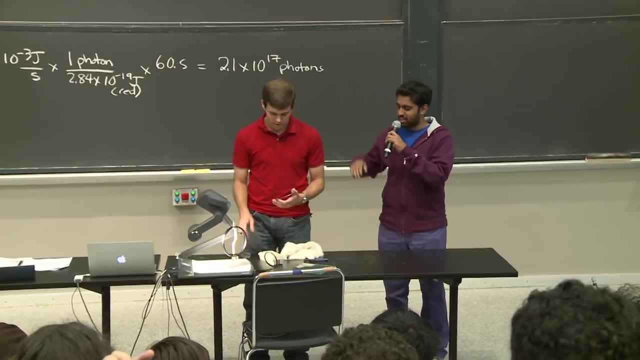 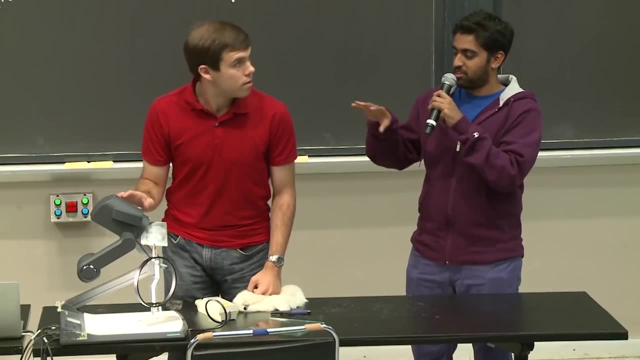 It's steel wool. It's, yeah, Steel wool. Oh, OK, So that's just going to get the aluminum oxide off, because sometimes you guys will get to it, but sometimes you can get a reaction of aluminum with the moisture in the air and that's. 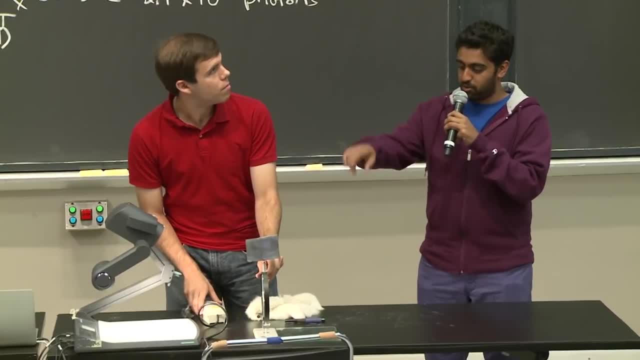 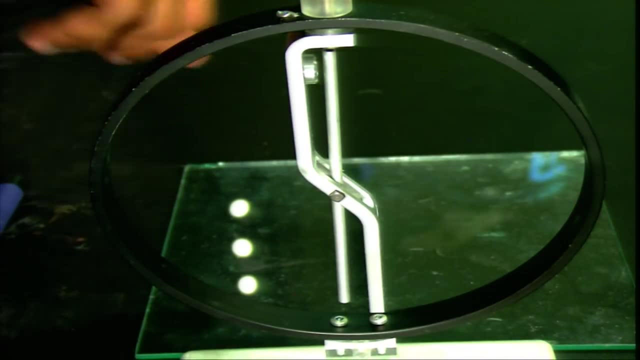 going to cause aluminum oxide, So he's getting rid of that. And now we've put this on a. what is this? What do you call it? A detector of some kind? So basically, when he charges this, what's going to happen? 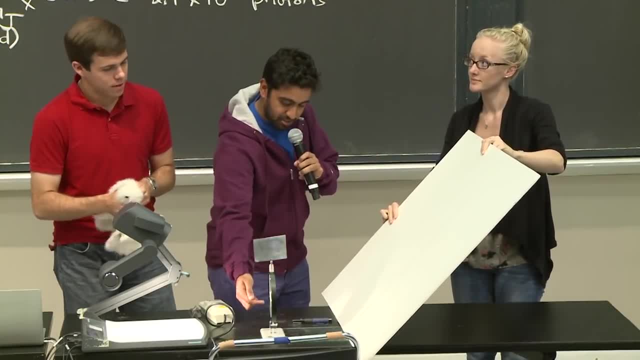 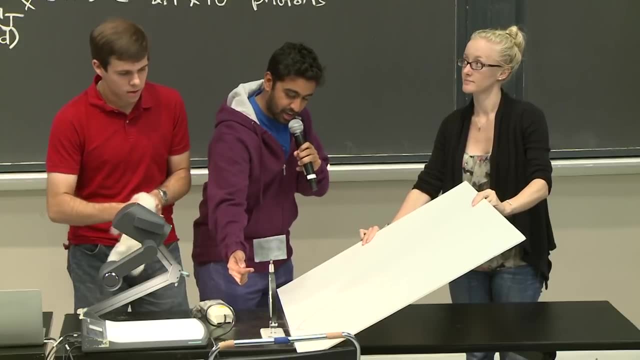 is that you have this plate and you have this, this joint, and they're both going to be electrically negative, right, because you've introduced some electrons And they're going to repel each other because they're both negative. Two negative charges repel each other. 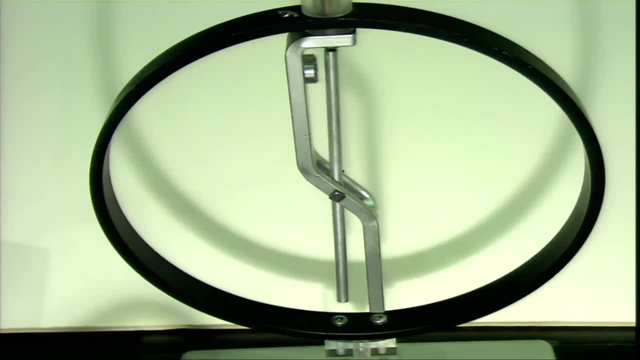 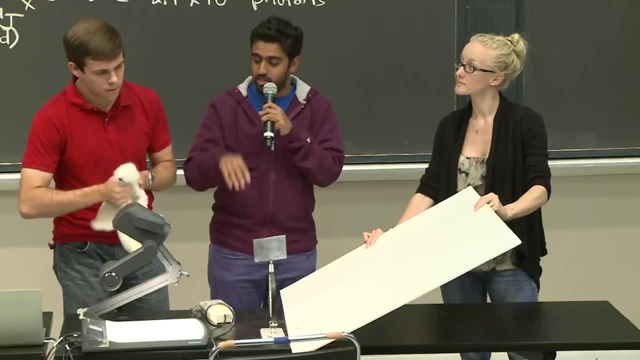 So you're going to see some space develop, as Eric's done. Now. what he's doing is he's got a plastic rod here that he's charging with the fur and he's introducing those electrons onto the plate. So now we've got a negatively charged plate. 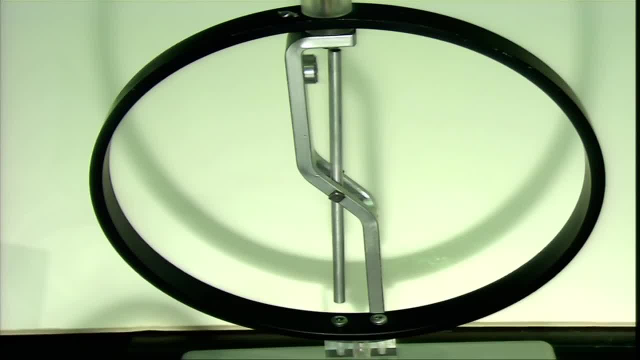 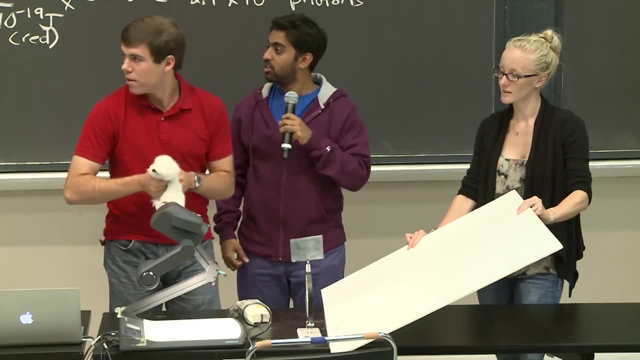 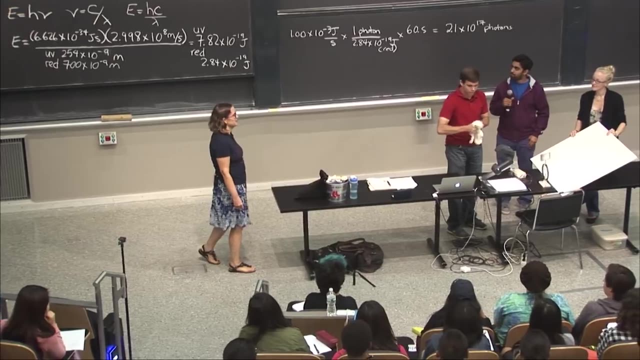 and you can see that by the fact that you see some repulsion between that rod and the rest of the detector, which is actually working out pretty nicely, So once-. So let's say this experiment is very weather-dependent. If it's really humid or too dry, it doesn't work nearly as well. 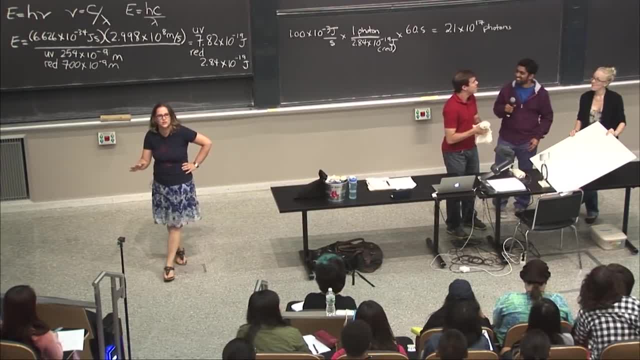 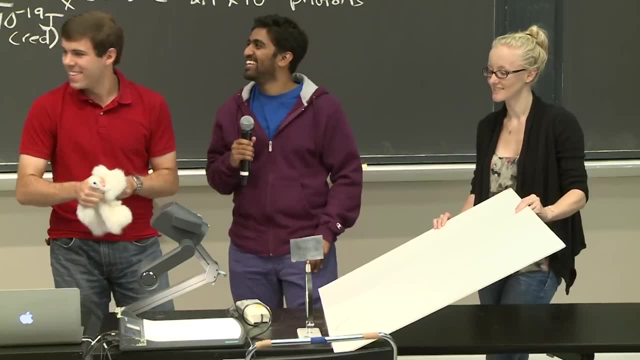 But today, today's good weather, Today's good weather for this experiment, Not so much good for sunbathing outside, but good weather for this experiment, Although we have a UV lamp, so maybe That's true. OK, so now we've got a charge. 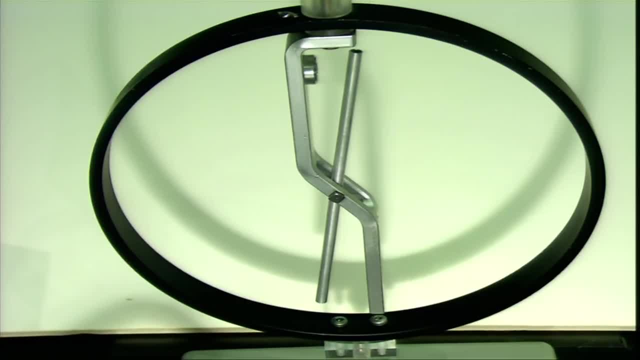 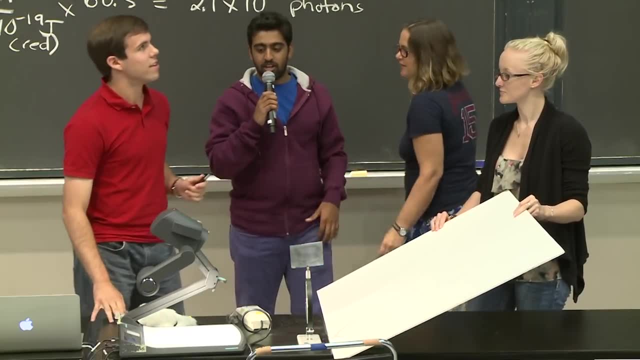 Actually, that's the green laser point. Let's get the red. It's underneath here, I think. Oh yeah, OK, so now- We could do the calculation for the green, If you want to do the calculation for the green? 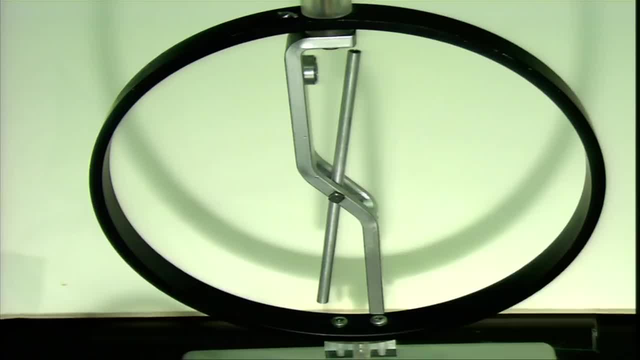 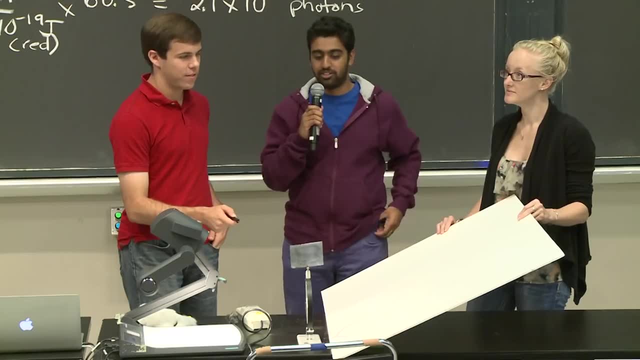 we can try it later. Eric's got a red laser pointer in his hand. He's going to shine it and we're going to see that nothing happens because, as we calculated, the energy of these photons is not enough to get over the threshold. 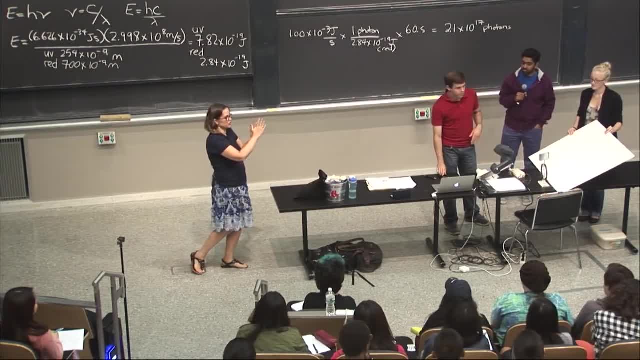 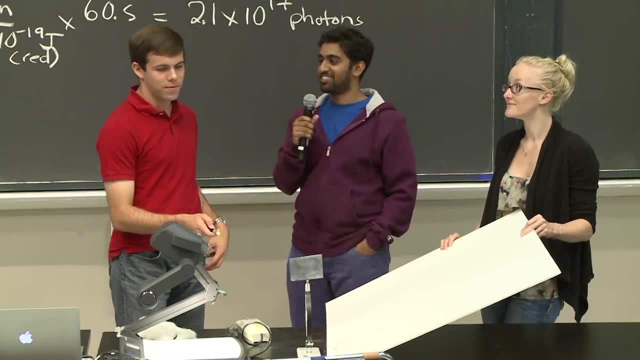 of this particular metal. So if electrons were being ejected, you should see it move. Just try the green one And we'll do it one more time. Maybe the green one will work. It doesn't All right. well, now we have to see if the UV built it up. 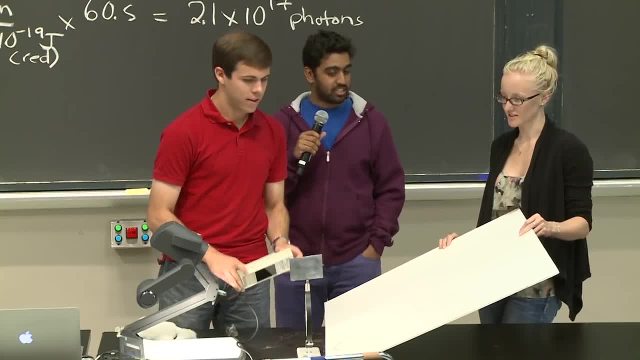 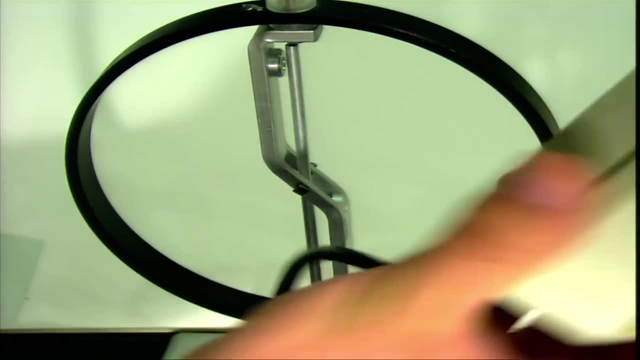 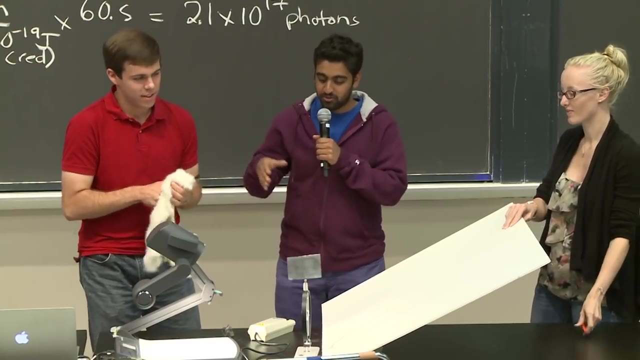 The UV should work. Let's see. OK, so maybe- I guess it worked, It did work, Could sort of see that. So maybe we can charge it up again while I talk about it. So the UV lamp obviously has enough energy. 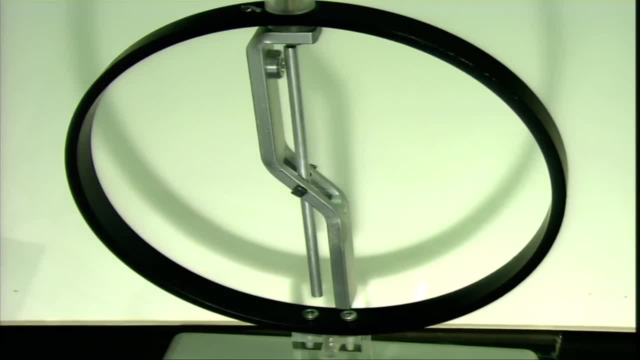 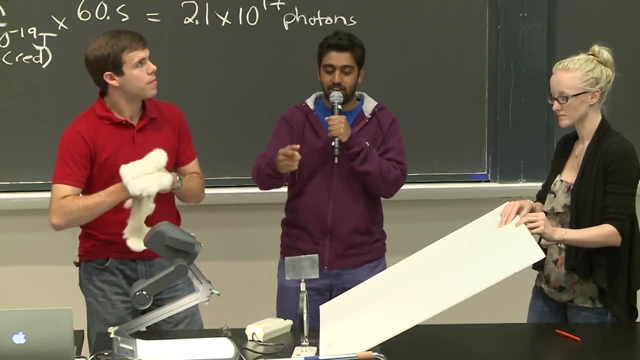 in each of these photons. So when you shine that light at the metal, you have the electrons on the surface which are being ejected. And if those electrons get ejected then the whole system becomes neutral. If the systems become neutral then that rod can go back. 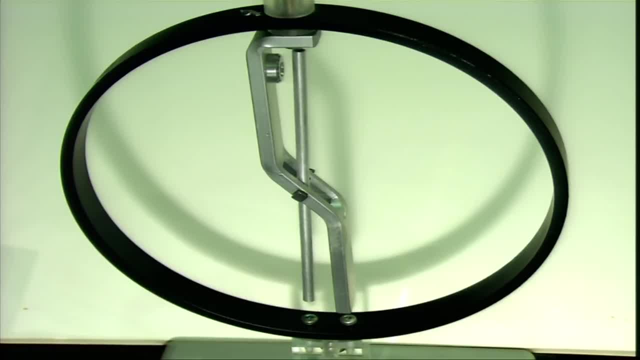 and feels a repulsion because the two parts are no longer negative. So once we charge this up again, maybe we can go to the other side. I think it's good. It's good, Yeah, that's good. Oh, It'll be fine. 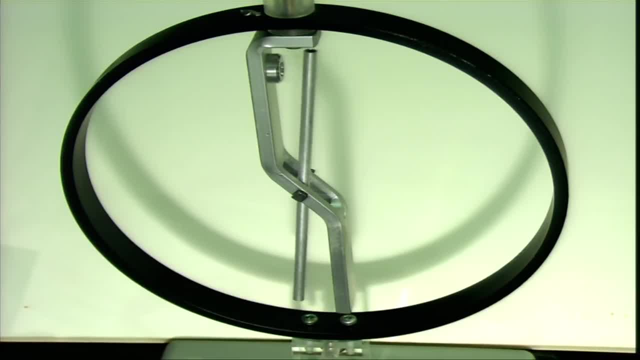 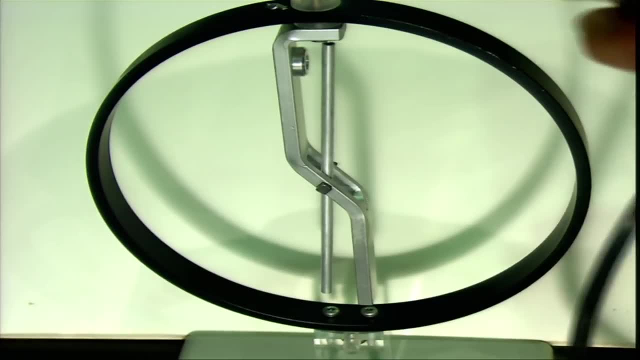 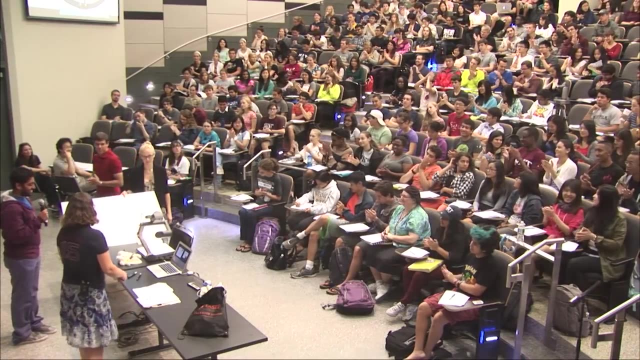 That's fine, Wait a minute, OK. OK, Now we're just going to try it again And yay, Yay, Yay, We got it. OK, All right, Great, We can just kind of leave this here. 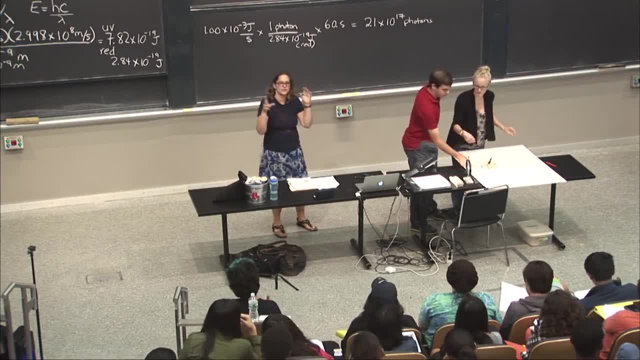 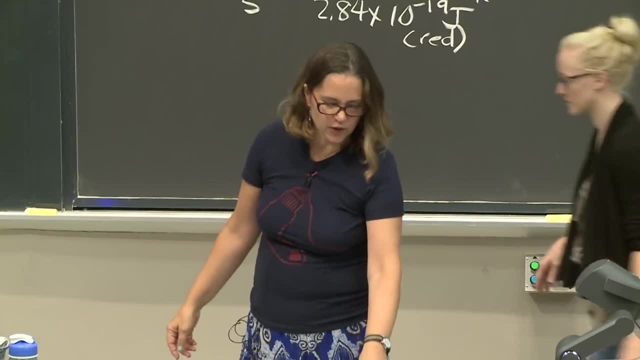 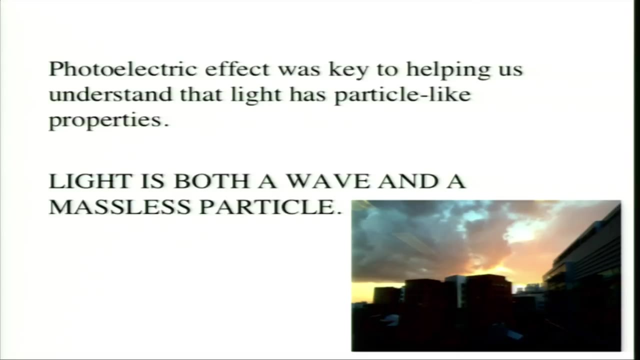 All right so, and I think he held it for 60 seconds to sort of know how many photons were coming off too, if you want to do that calculation. So again, the photoelectric effect was really important at this time in understanding the properties that were being observed. 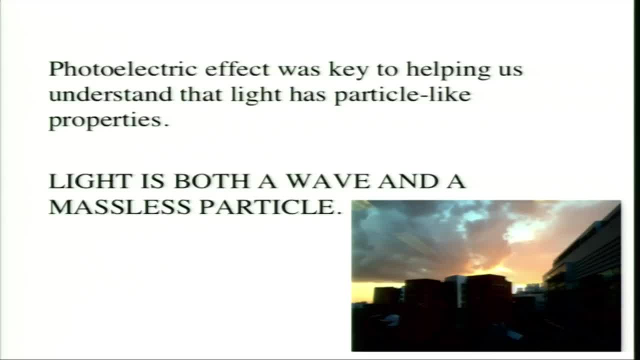 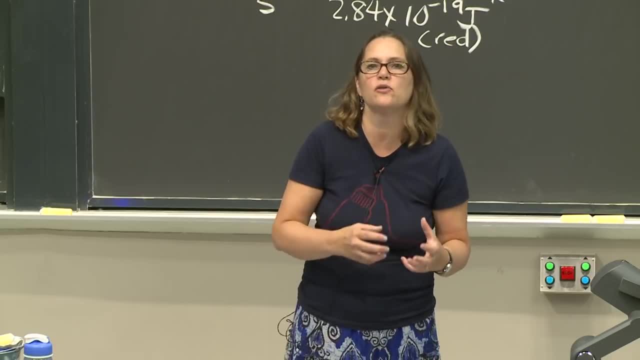 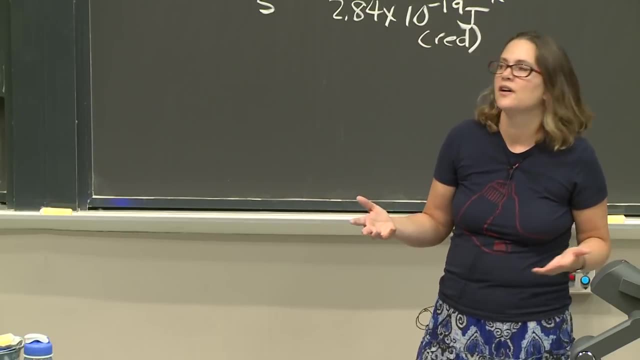 to help us understand about this quantized energy of particles, that light had this particle-like property. It had this quantized energy And you needed a certain amount of it to eject an electron from a metal surface. So we all know that light is a wave. 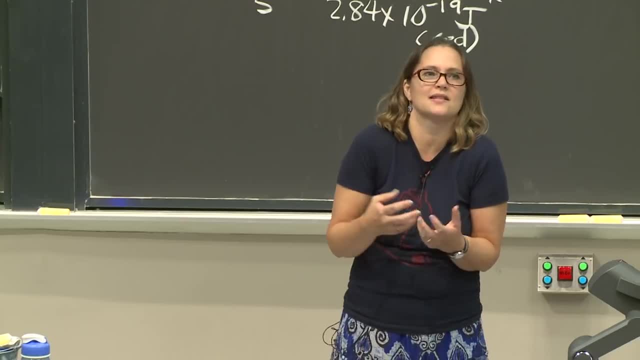 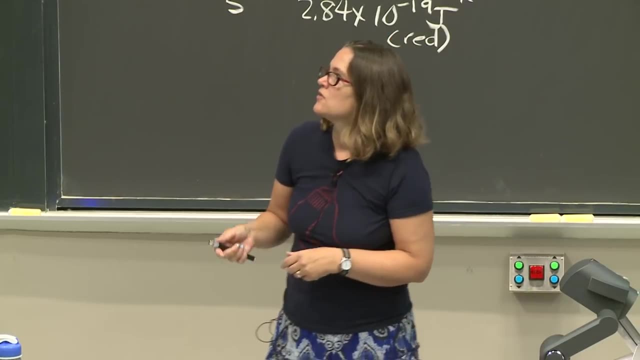 But now there's this evidence that, even though it's pretty much this massless particle, that it still has particle-like properties. So light is a really amazing thing. This doesn't really show up very well. It's a view of the Stata center. 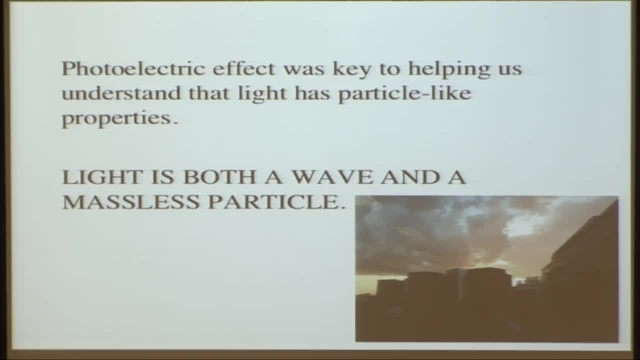 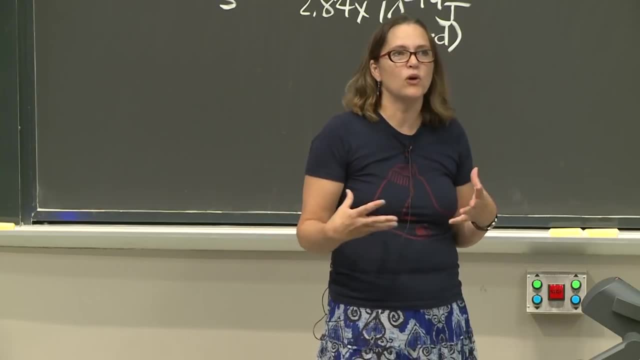 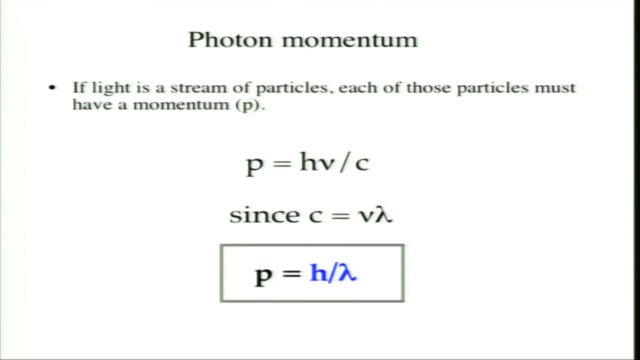 The Stata center always has some really spectacular sunlight coming around it sometimes. All right, so now, if this is true, that means that photons that have this quantized energy should have momentum as well, And so Einstein was thinking about that, And so he reasoned that this had to be true. 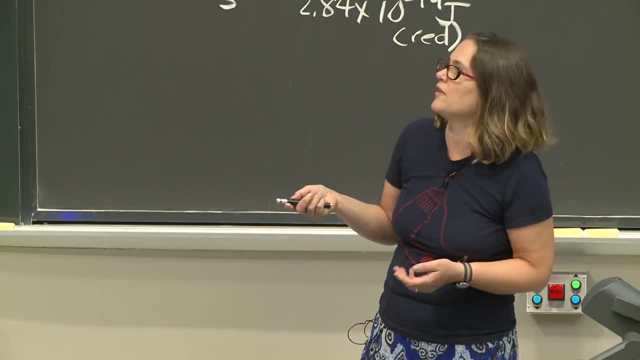 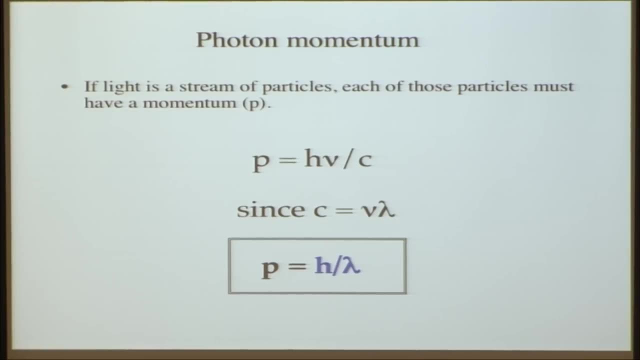 There had to be some kind of momentum associated with them, And so momentum, or p here is equal to Planck's constant times, the frequency divided by the speed of light, c, And since the speed of light is equal to the frequency times, the wavelength of the light. 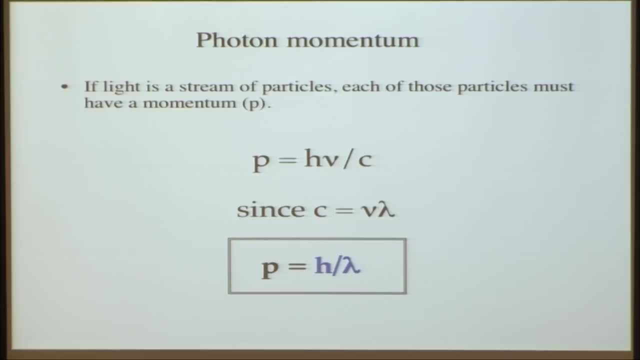 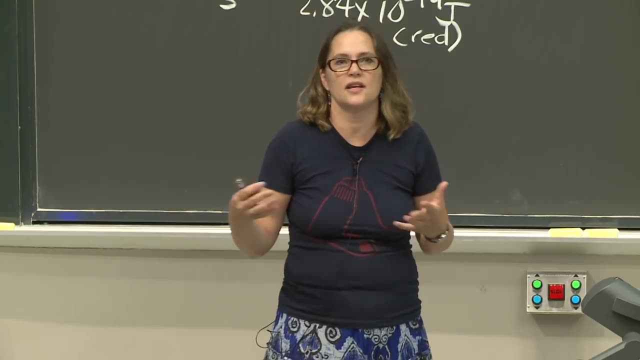 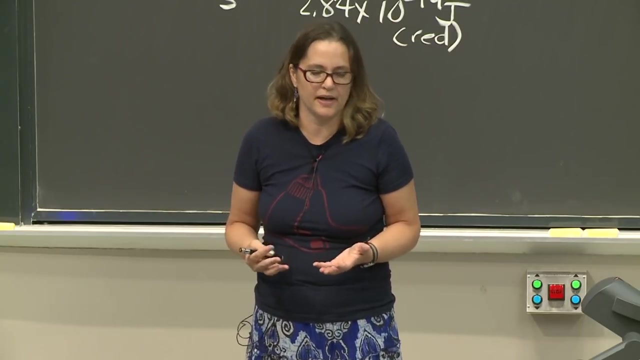 then the momentum should be equal to Planck's constant divided by the wavelength. So this is really. we're talking about momentum in terms of wavelength, this inverse relationship here. This was just kind of a crazy idea to be thinking about momentum when you're talking about light. 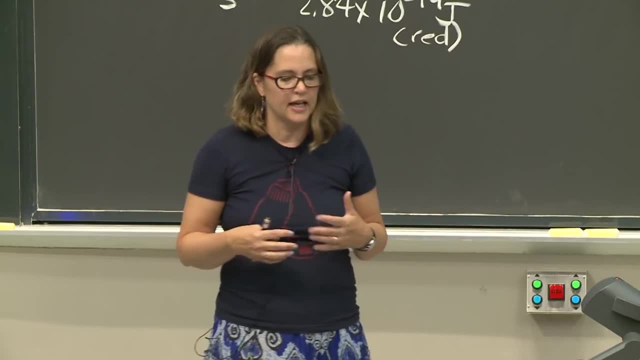 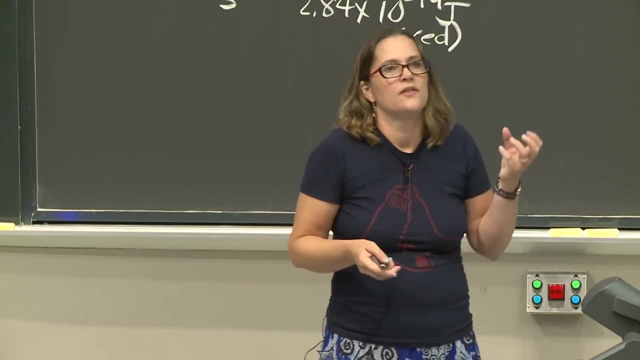 And this really kind of came out of the photoelectric effect, And also there were some experiments done by Arthur Compton that also showed that you could sort of transfer this momentum, And so that's really cool And so that's again this sort of particle-like property. 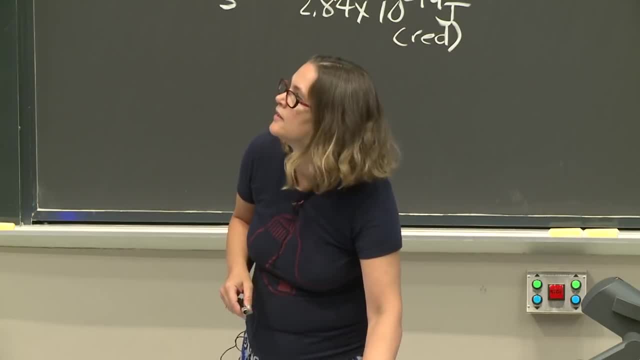 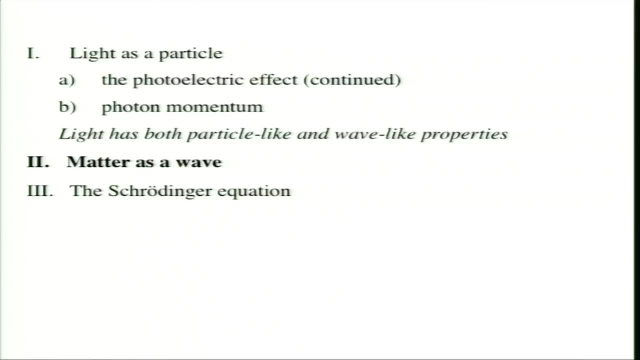 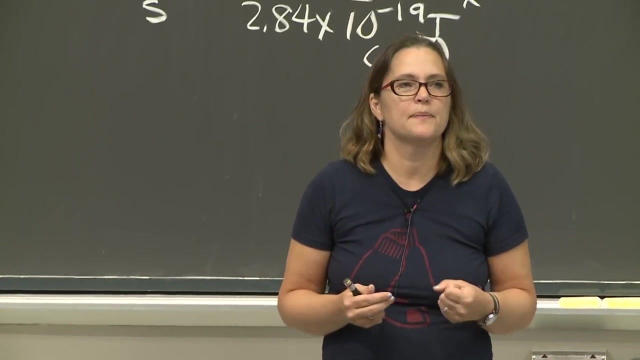 So it's a really exciting time. OK, So we're going to now move to matter. So we've been talking about light, and how light has this dual particle wave-like properties? But what about matter? So we accept that matter has particle-like properties. 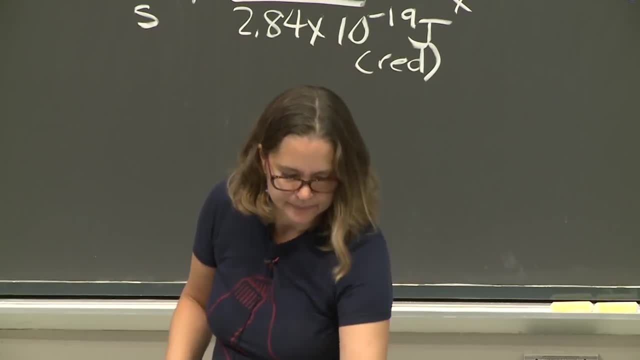 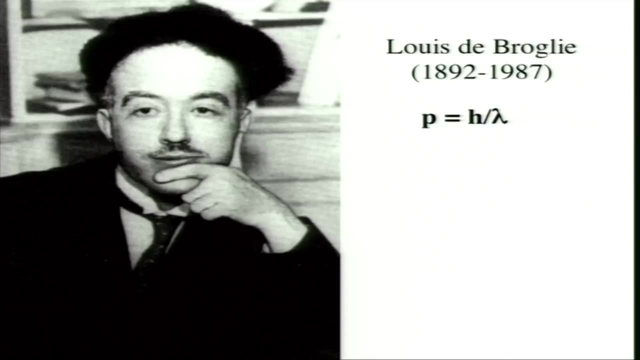 But what about as a wave? So enter de Broglie into this area, And so he was following sort of what Einstein was thinking about And he said, OK, so that's pretty cool If you have, momentum is equal to Planck's constant divided. 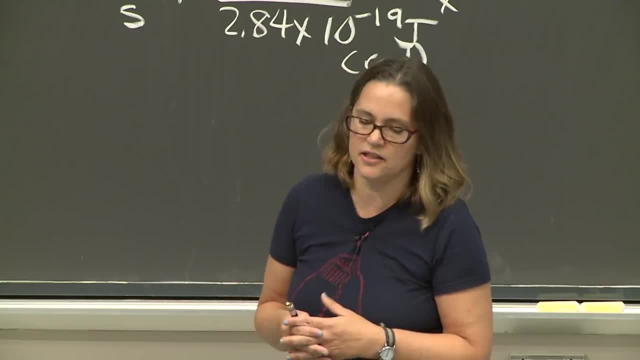 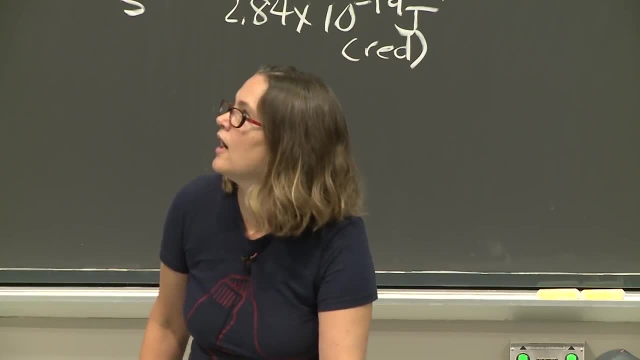 by wavelength. if you could think of things that have wavelengths as having momentum. And he said: or I can rewrite this equation and say that the momentum is equal to Planck's constant divided by wavelength, So we can write this equation that wavelength 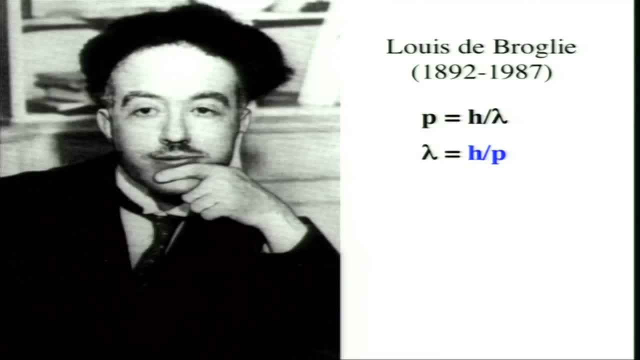 equals Planck's constant divided by momentum, And we know something about momentum. We know that momentum is often associated with something's mass times, its velocity, So therefore I should be able to rewrite this equation again in terms of wavelength being equal to Planck's constant. 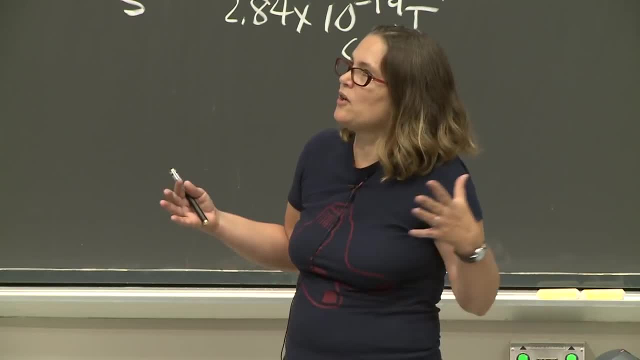 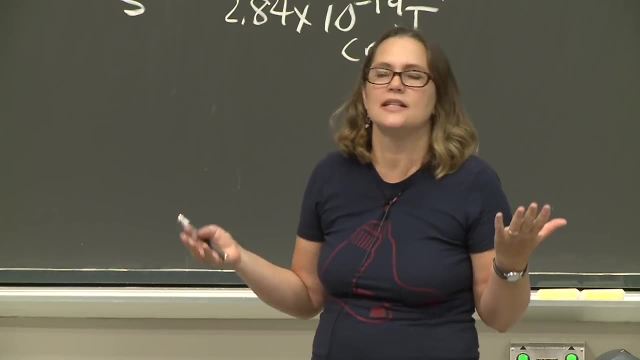 divided by a mass and a velocity, And here we are expressing wavelengths in terms of masses. So this was really something, And this was basically his PhD thesis. I think maybe it had more pages than that, but this would have probably been enough. 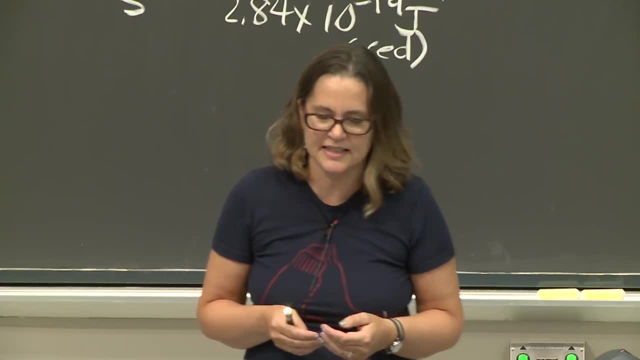 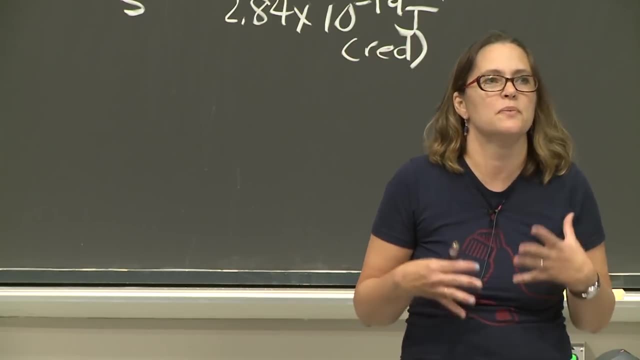 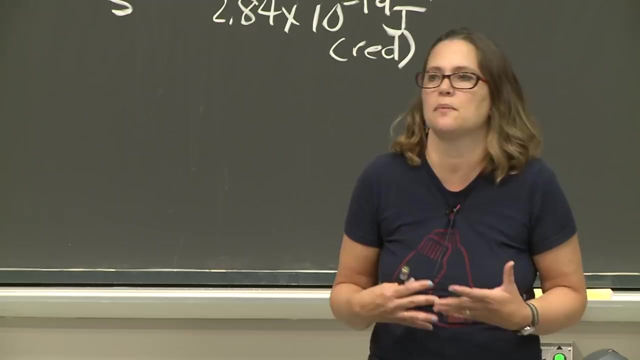 This sort of cover page. this is my PhD thesis, And Einstein said that he had lifted the corner of a great veil with really just manipulating what was known at the time and rearranging these equations and presenting relationships that people hadn't really put together before. 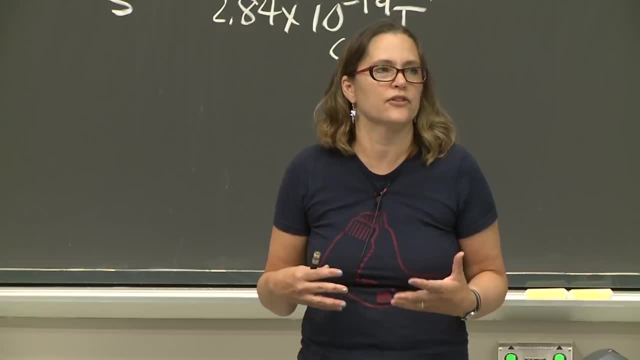 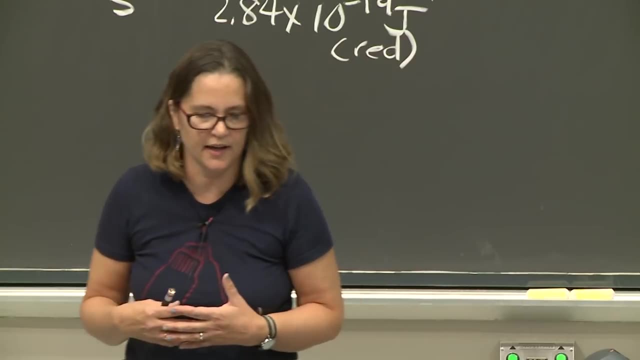 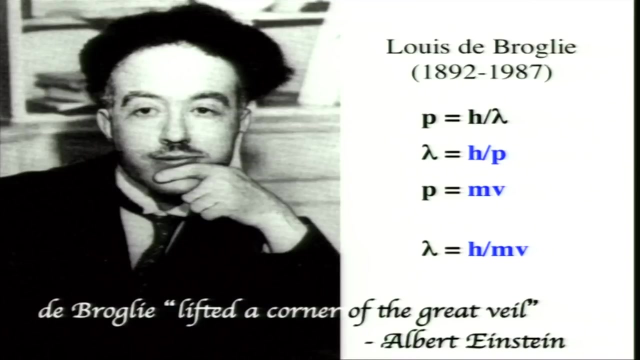 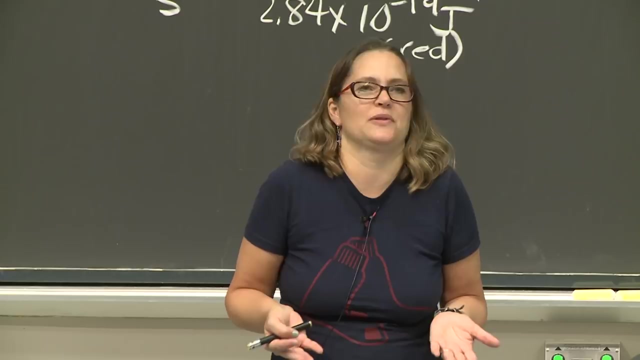 So he ended up winning a Nobel Prize, basically for his PhD thesis, which is a fairly rare thing to have happen, But this was really an incredible time. So, if this is true, if you have equations that relate wavelengths to mass and particles have wave-like properties, how come we don't see this? 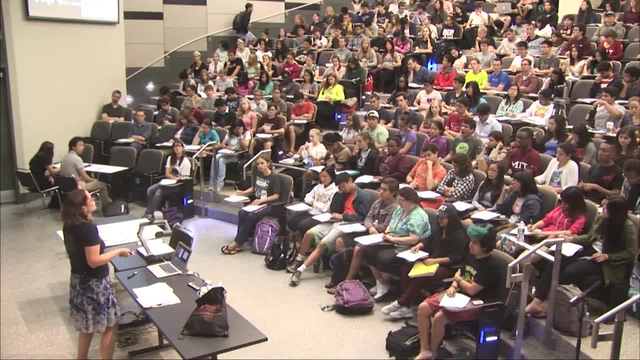 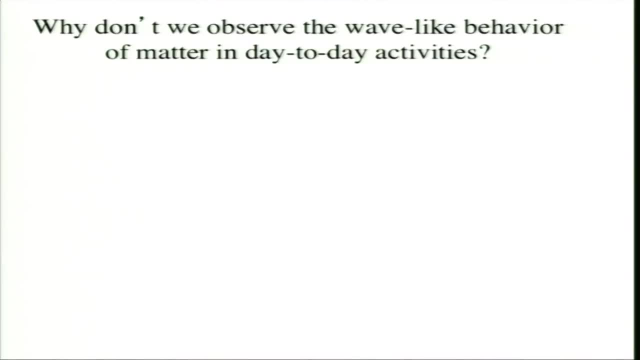 How come this isn't part? How come no one noticed the particle going by And sort of this wavelength associated with it? So why don't we observe this wave-like behavior if, in fact, it is associated with particles? So let's think about this a minute. 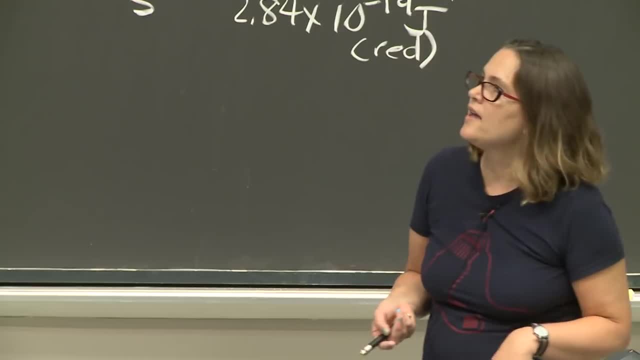 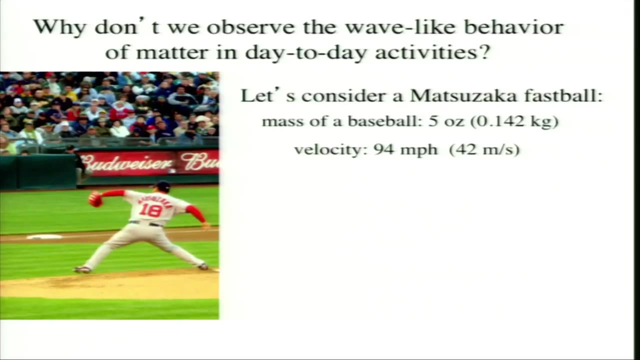 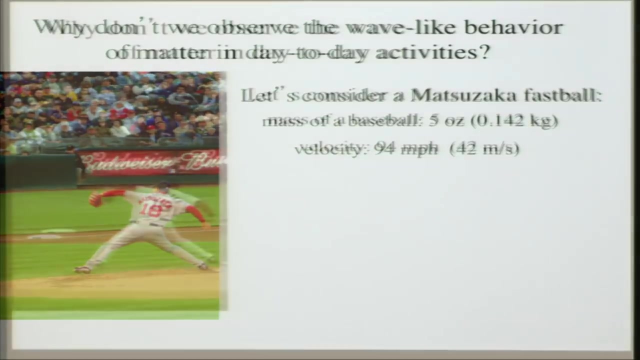 And we can consider why, when you go to Fenway Park- and you should, because it's fun and you watch someone throw a fastball- why you don't see a wave associated with that fastball. So we can consider a fastball and that the mass. 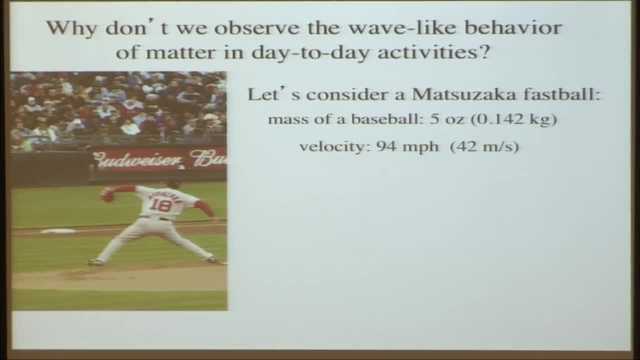 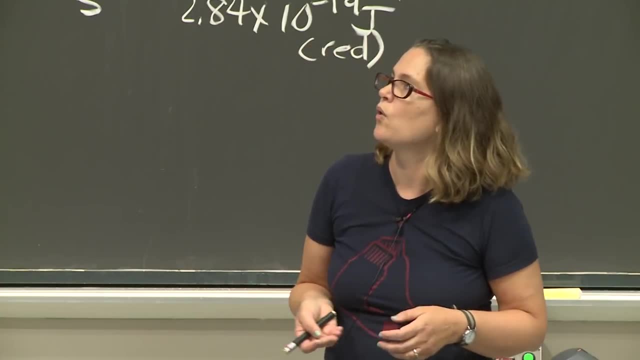 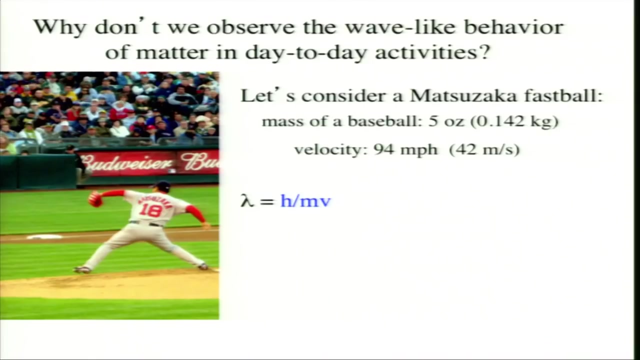 of a baseball is about 5 ounces, or 0.142 kilograms, And a velocity of a fastball is around 94 miles per hour, or 42 meters per second, And so we can do a little calculation and figure out what the wavelength associated. 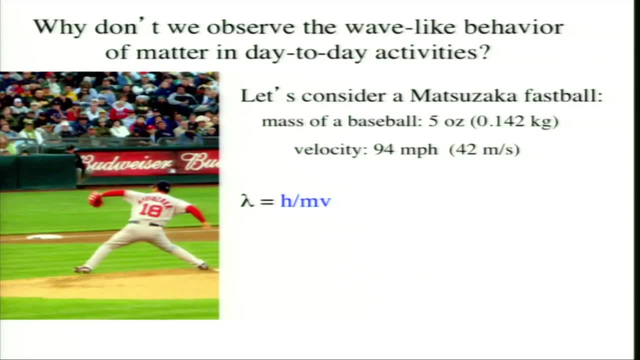 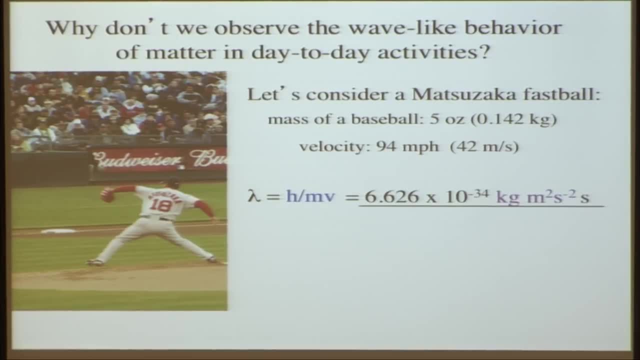 with that ball should be. So wavelength should be Planck's constant Over the mass times the velocity of the ball, And we can plug in these values. And here's Planck's constant again. And now you'll note I did something with the units. 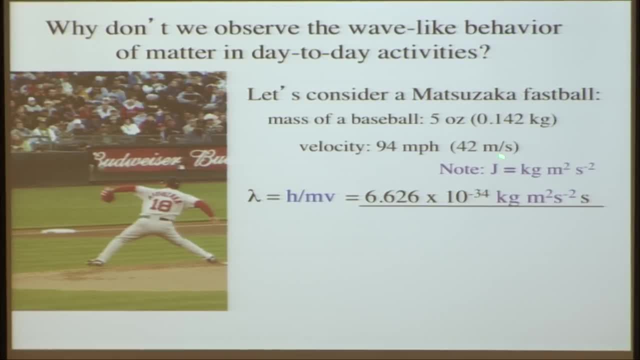 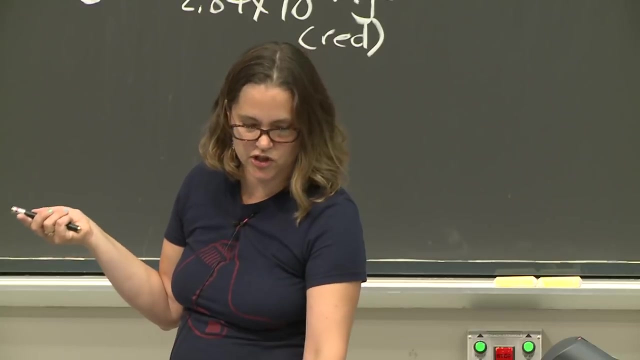 So instead of joule seconds, I substituted joules with kilograms meters, squared seconds to the minus 2. And that's what's equal to a joule. And I'm going to do that so I can cancel out my units. And again, all of this will be provided on an equation sheet. 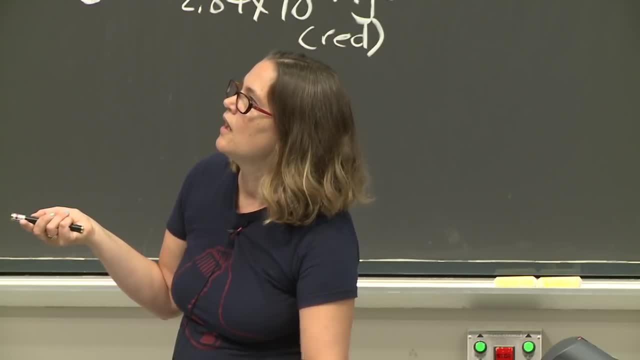 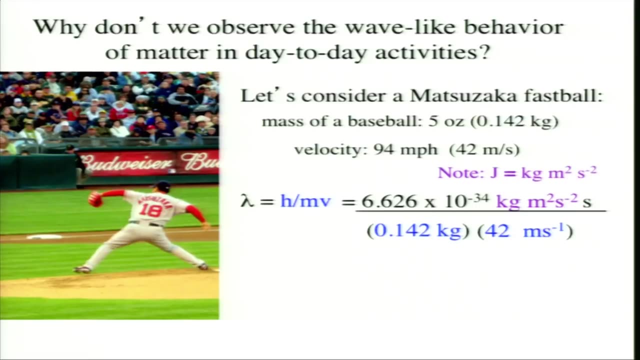 You do not need to remember all of these conversions. And so over the mass of the baseball and the velocity of the baseball, And we're going to put the velocity in meters per second, so our units can cancel out, And so I'll just cancel units out. 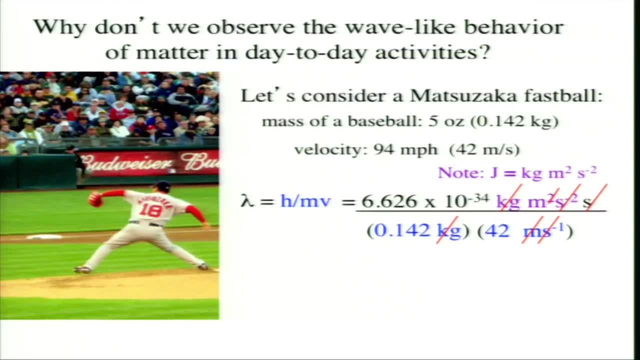 So we're canceling our kilograms, We're canceling one of the meters and canceling all of the seconds, And we have one meter left, which is good because we're talking about the number and we're talking about wavelength. So that's the unit we should have. 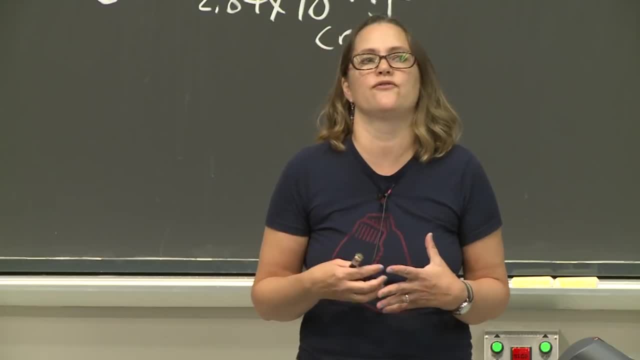 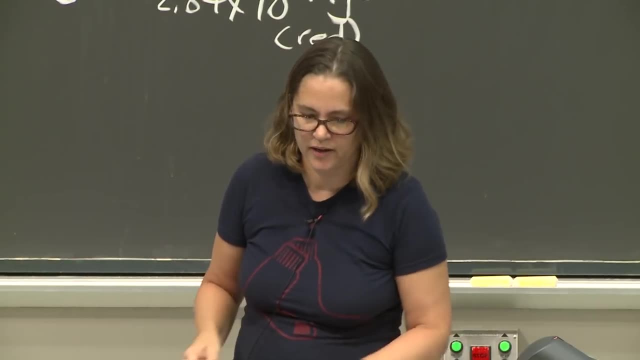 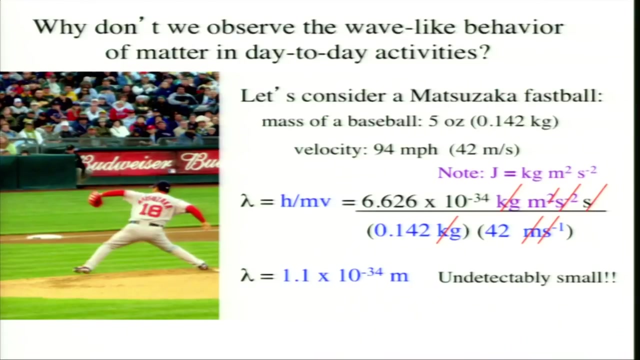 And the wavelength is 1.1 times 10 to the minus 34 meters. That is a really small number times 10 to the 34. And it is, in fact, undetectably small. OK, so now, why don't you try your hand at this? 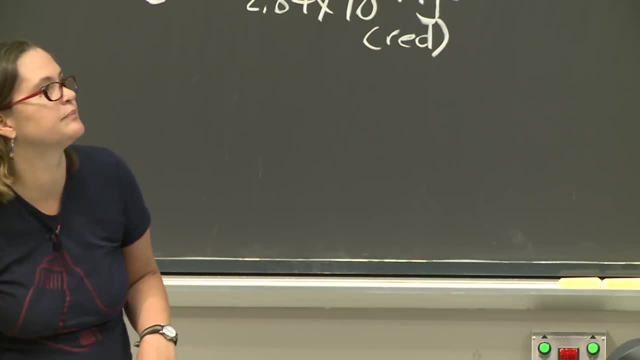 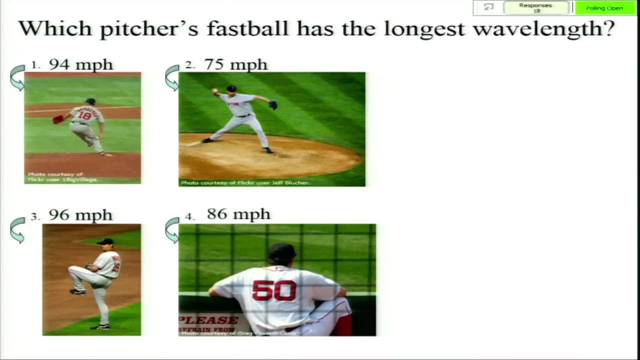 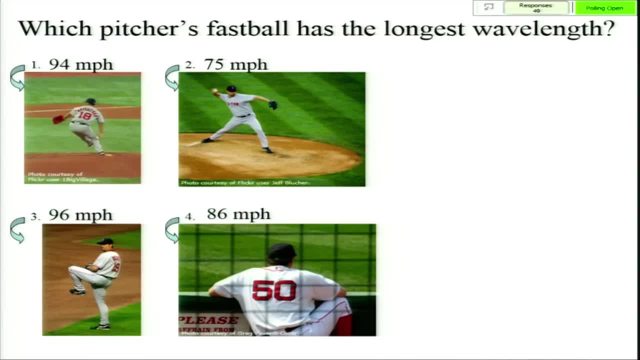 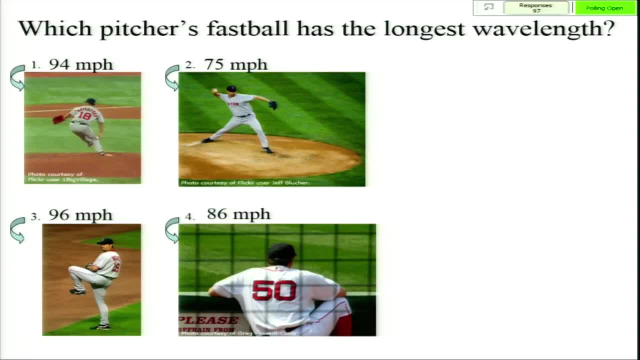 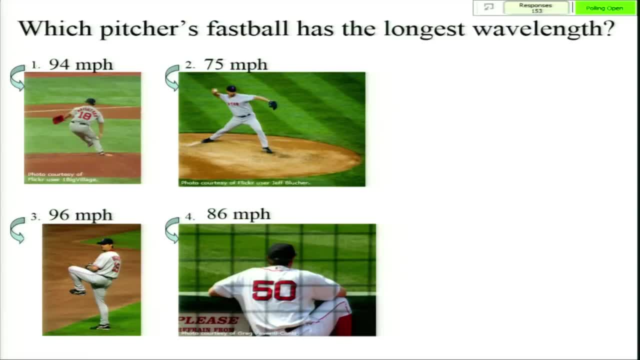 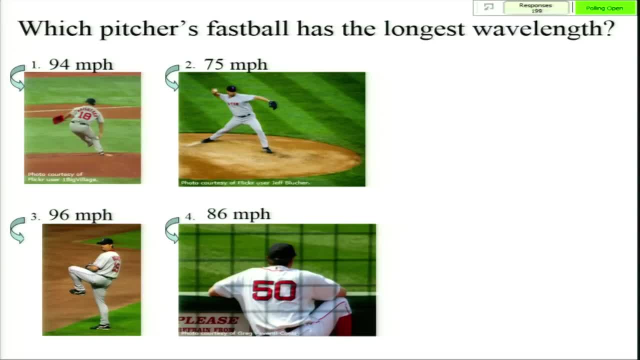 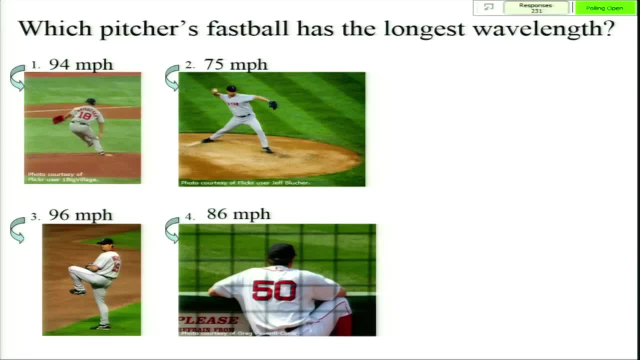 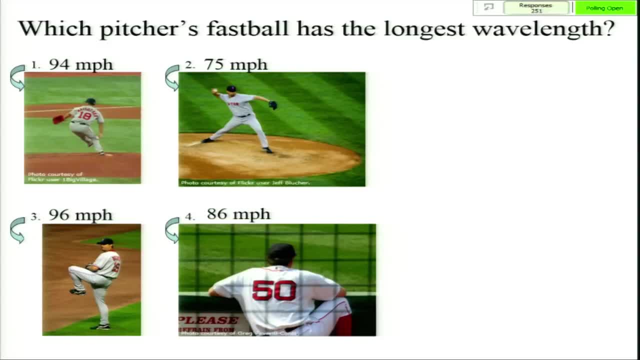 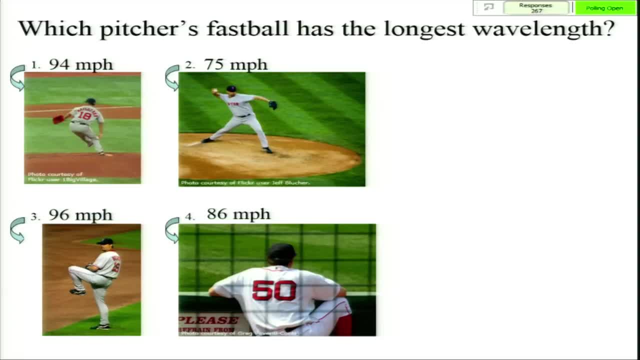 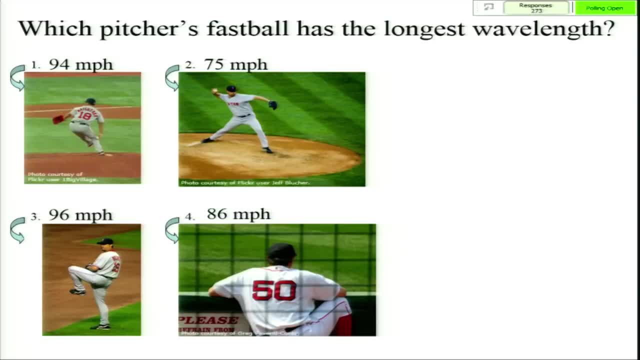 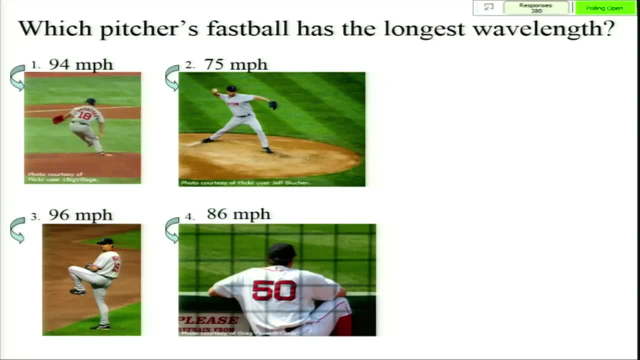 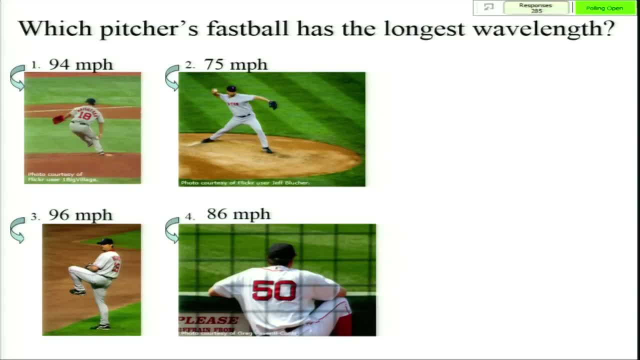 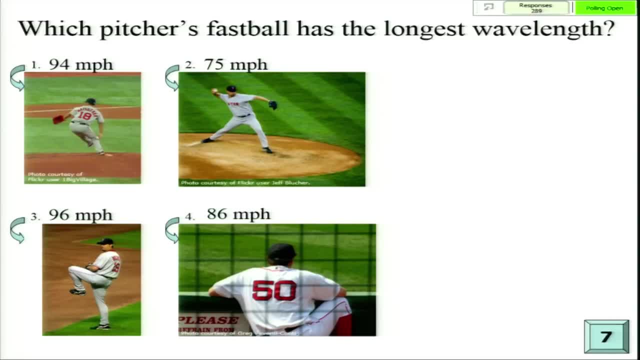 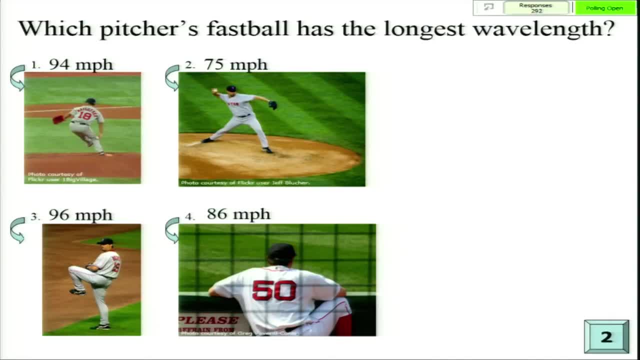 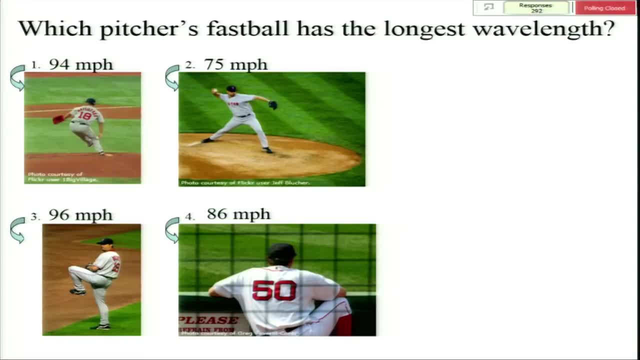 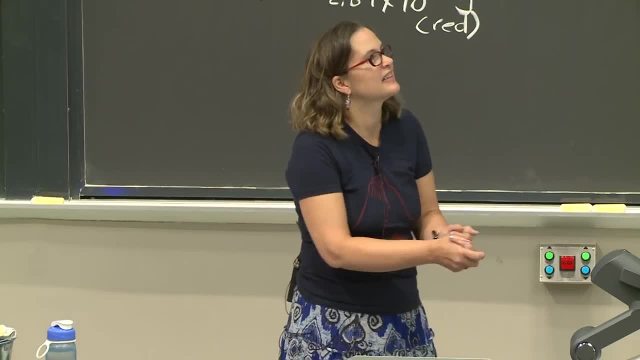 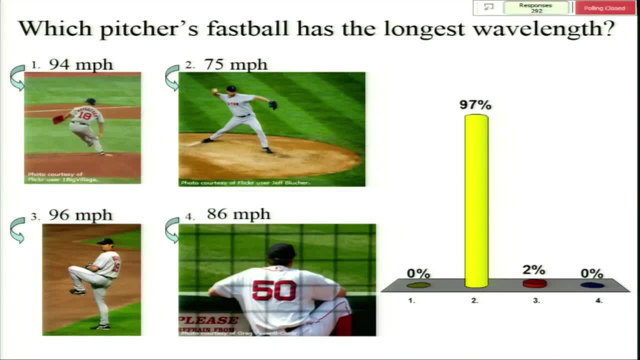 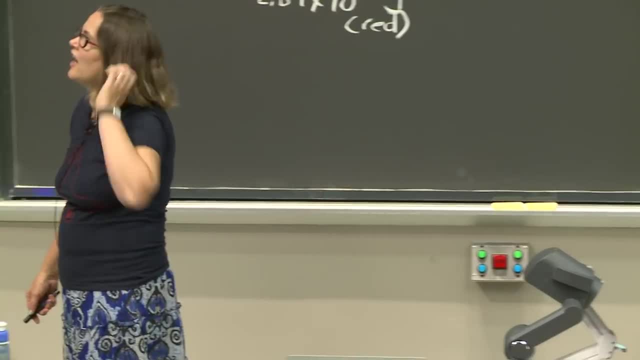 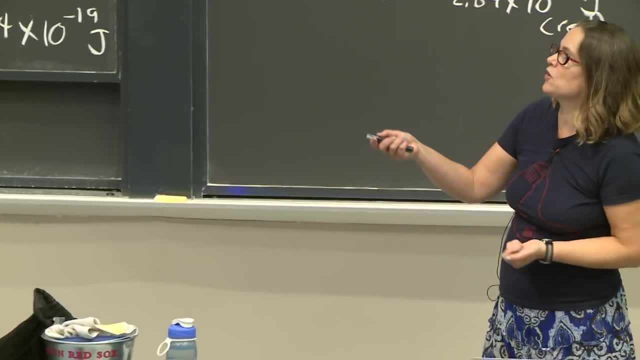 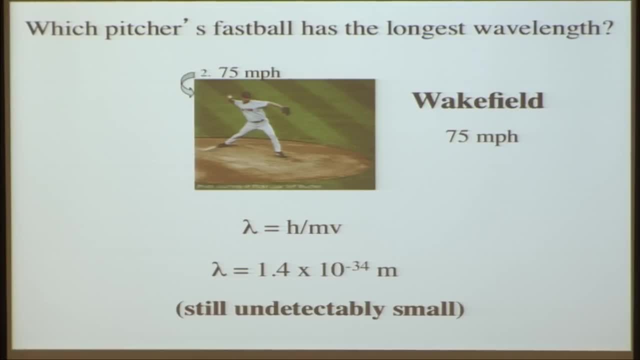 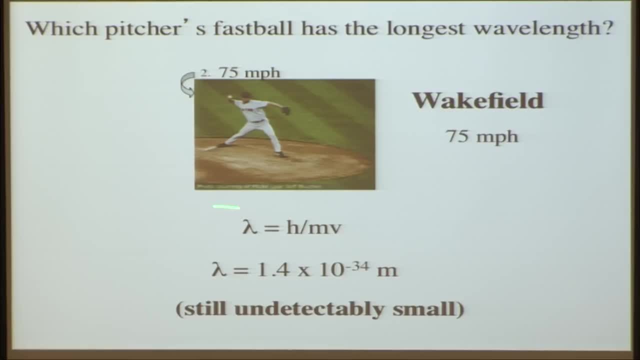 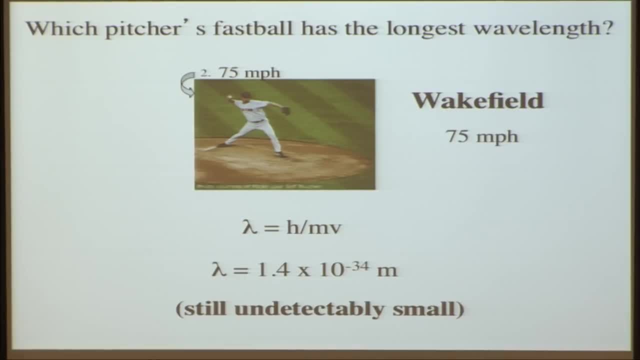 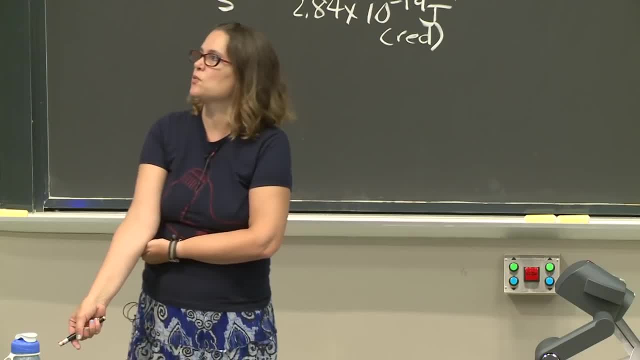 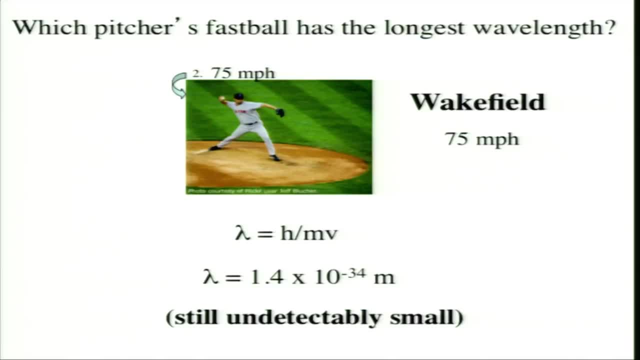 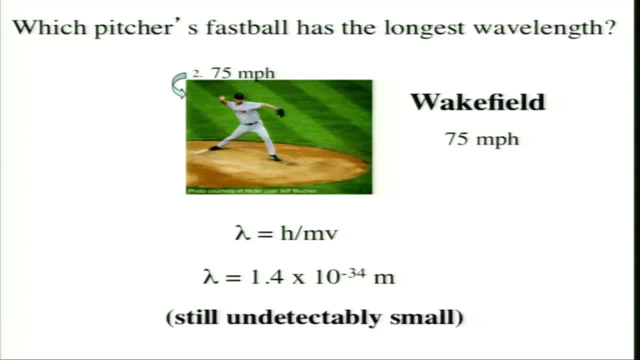 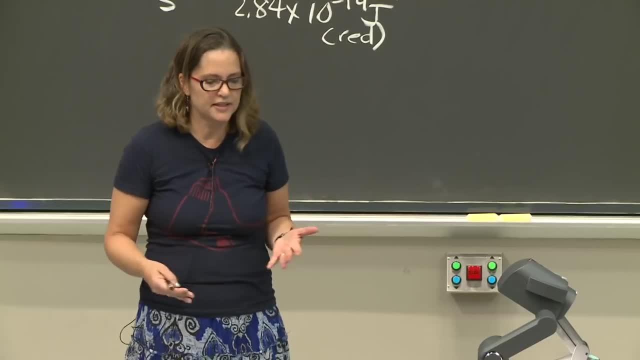 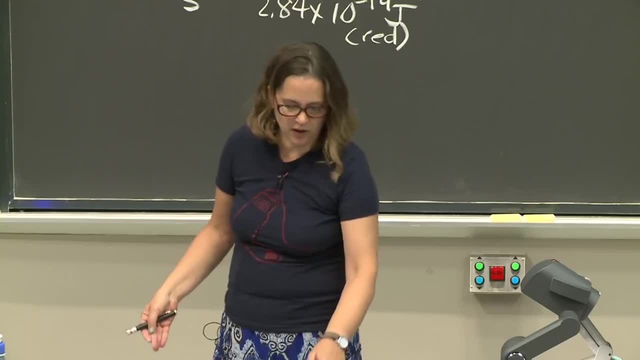 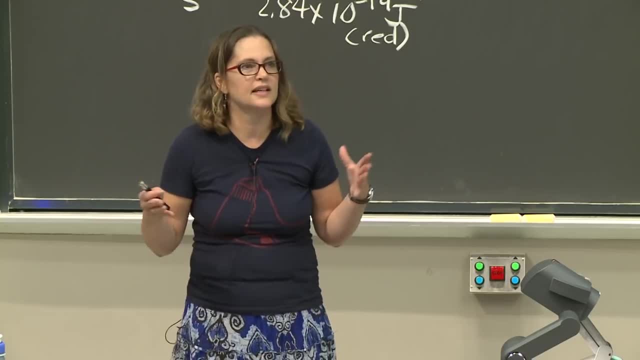 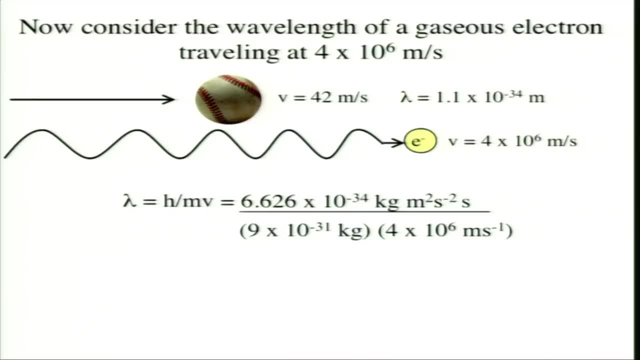 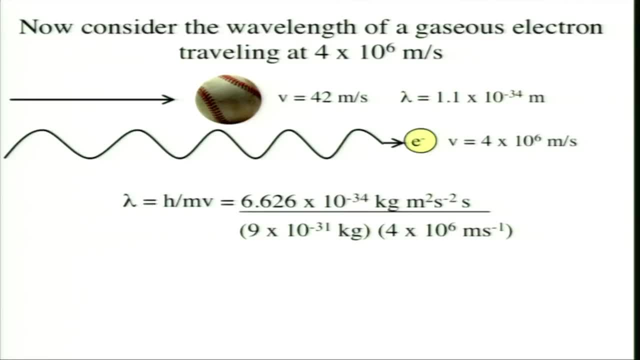 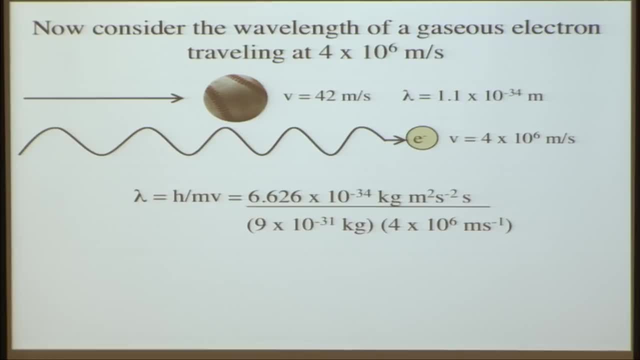 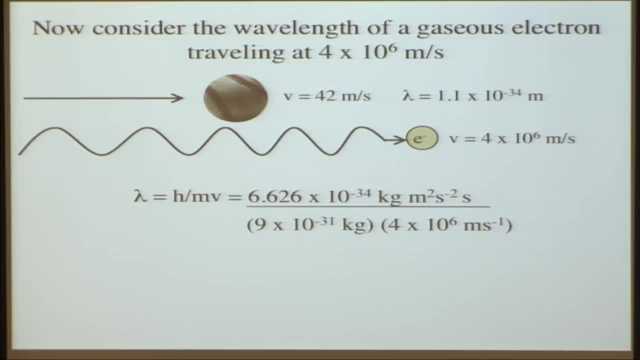 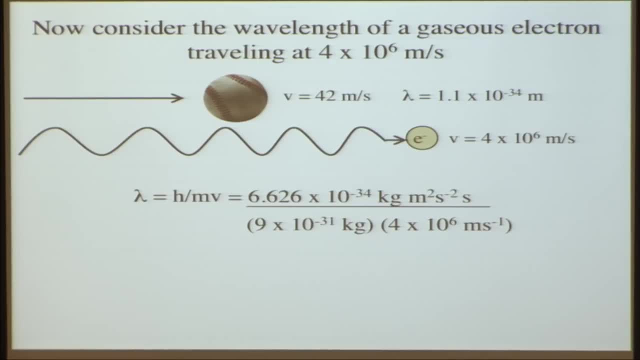 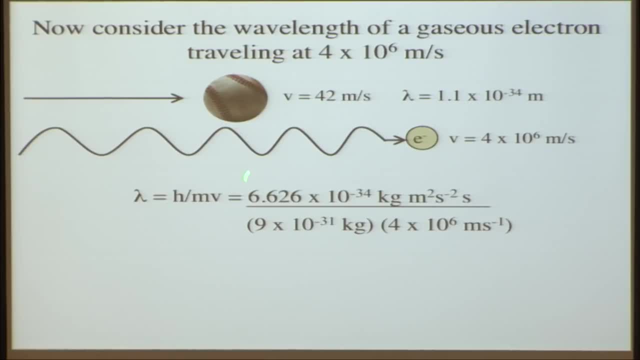 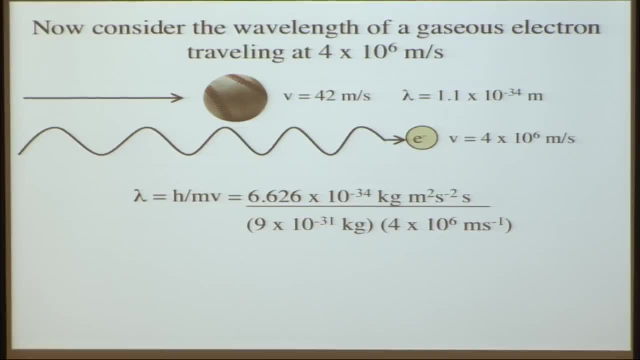 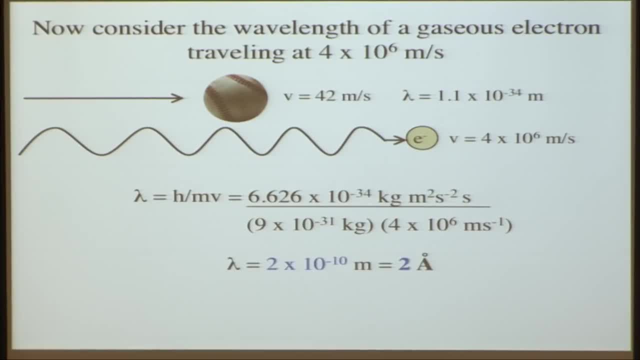 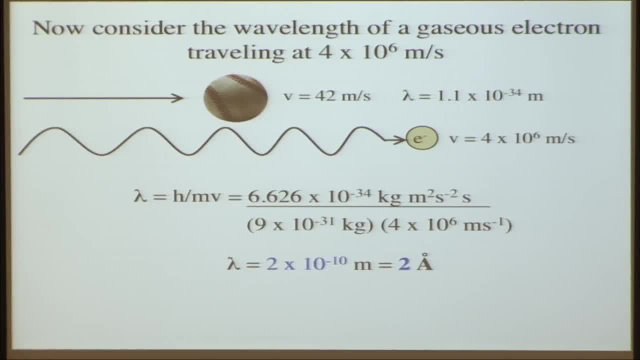 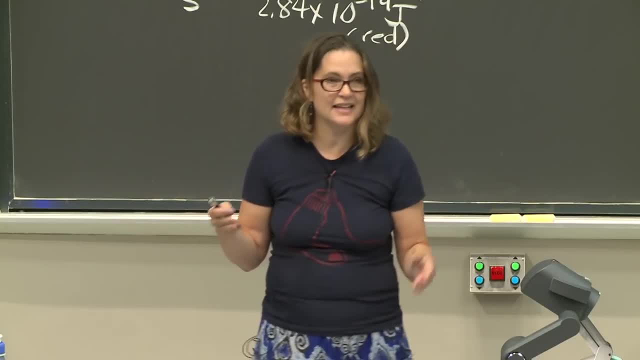 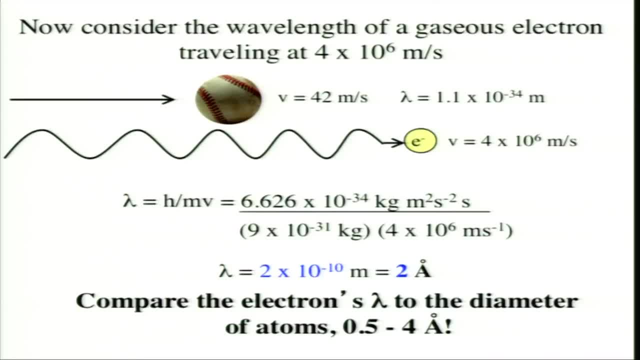 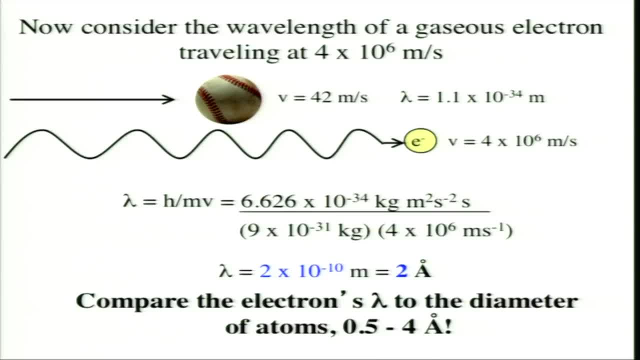 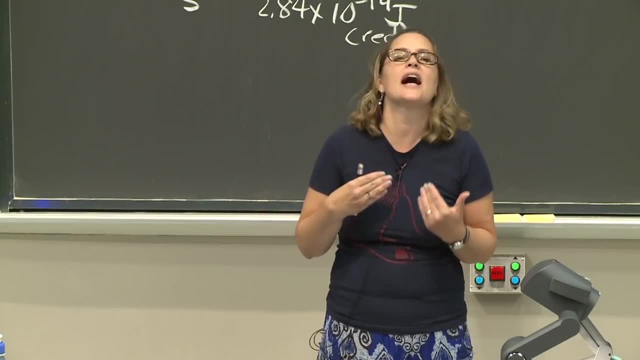 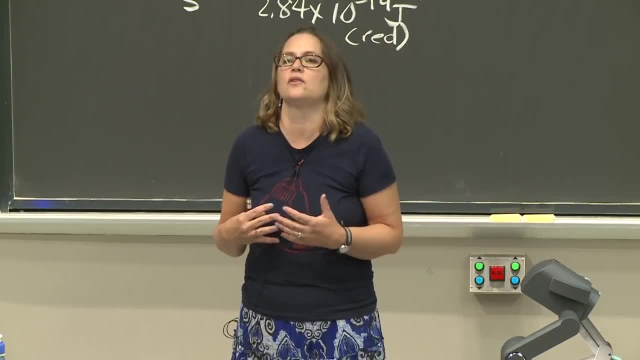 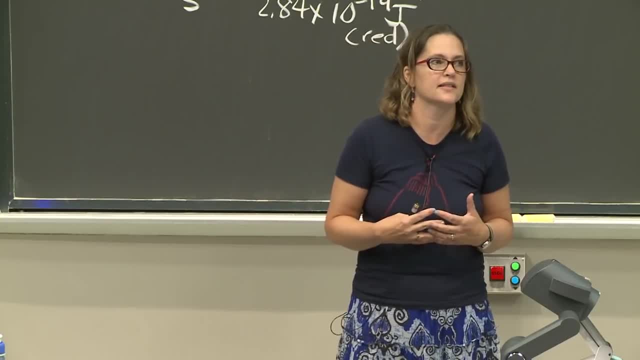 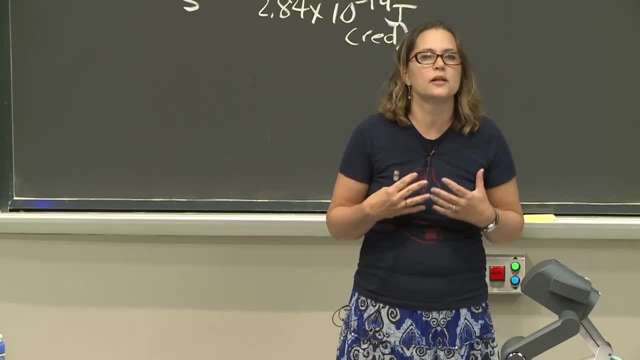 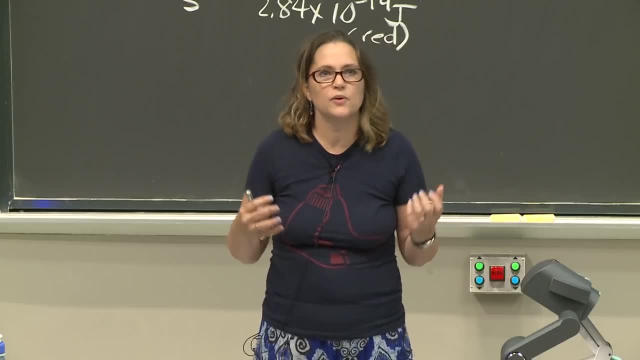 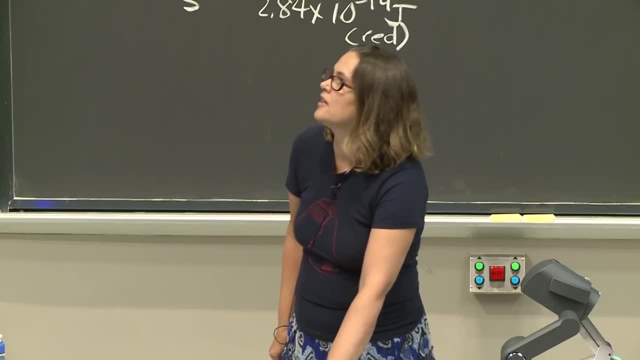 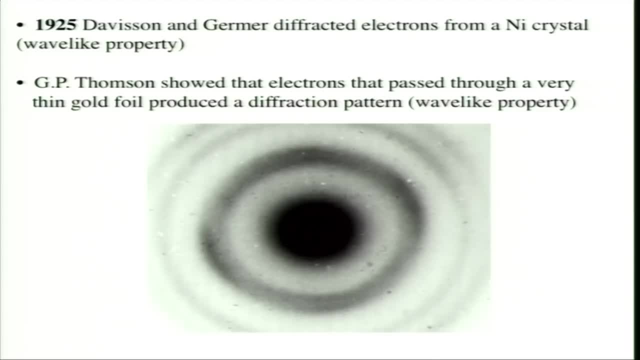 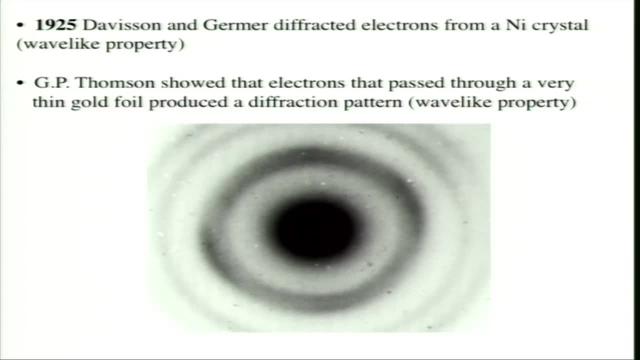 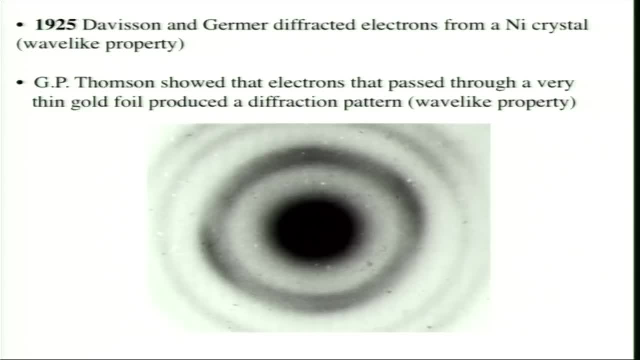 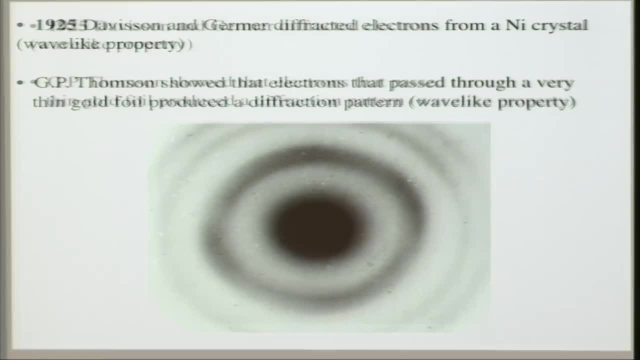 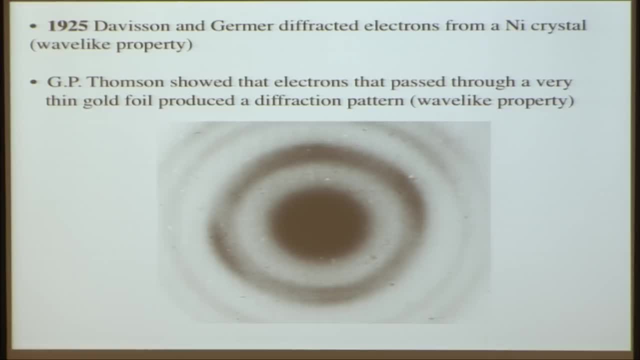 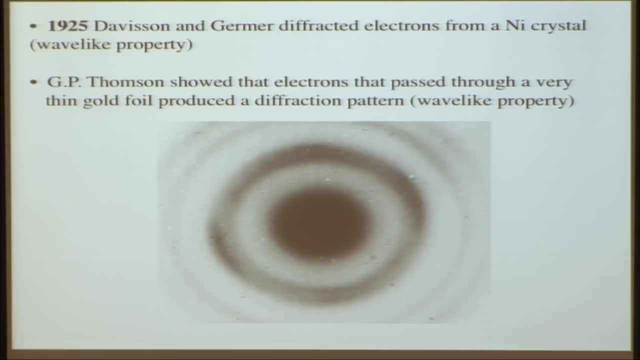 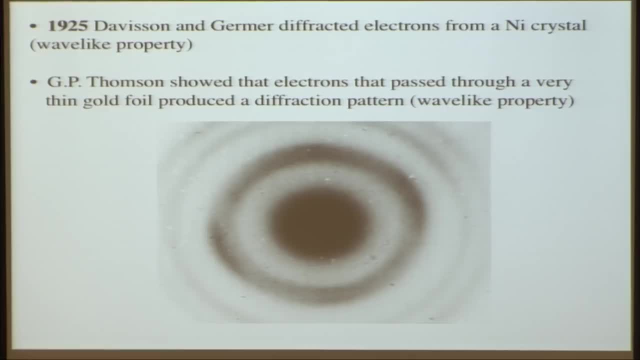 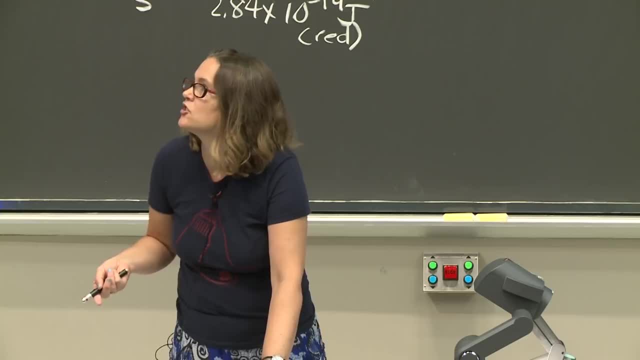 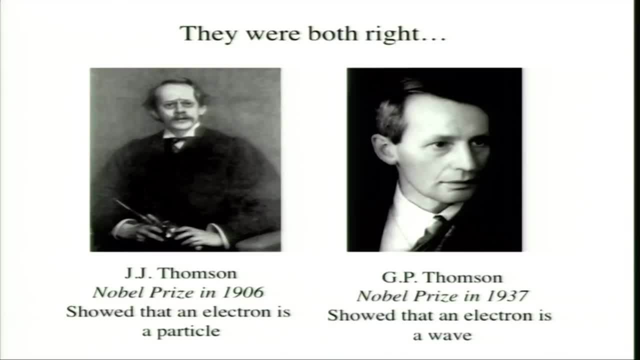 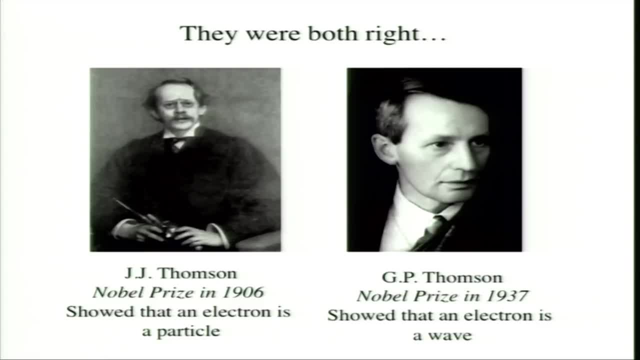 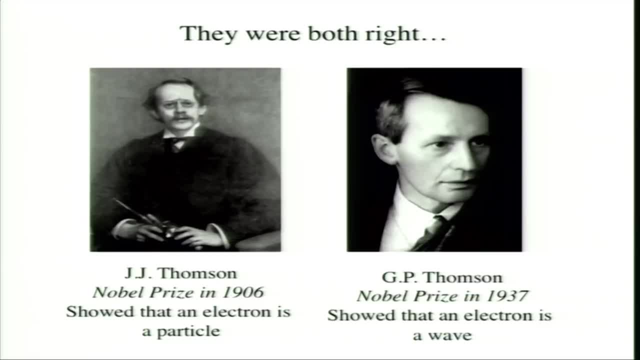 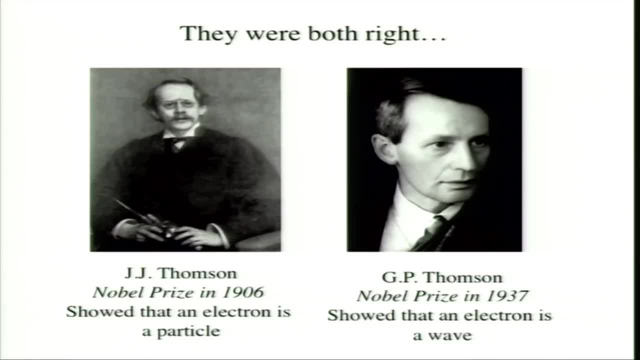 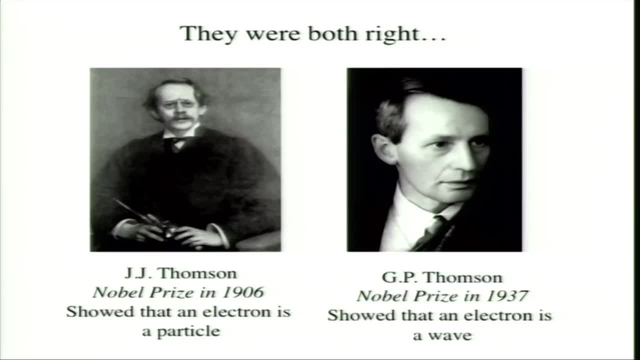 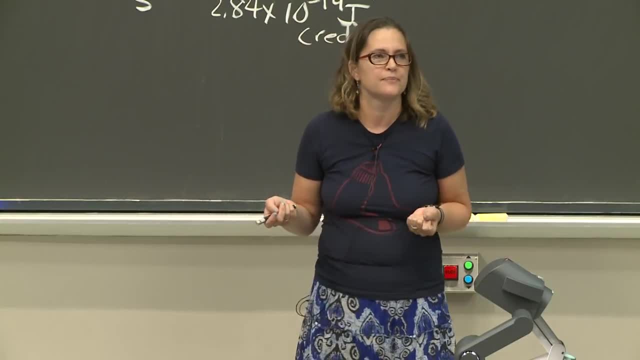 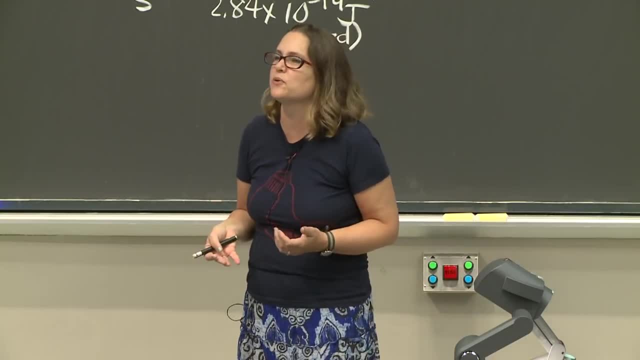 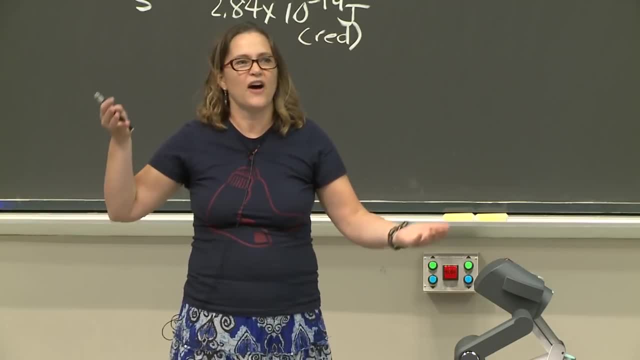 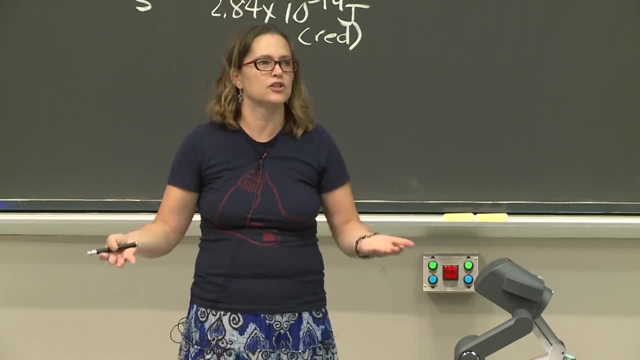 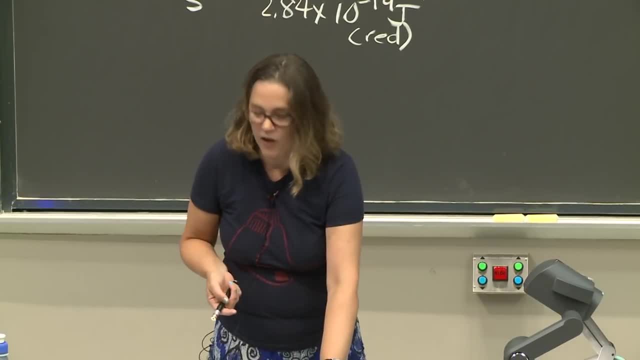 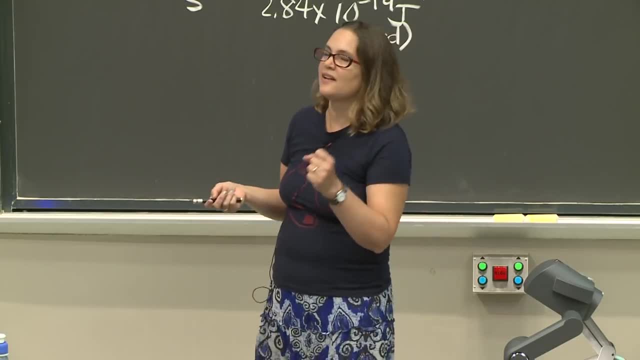 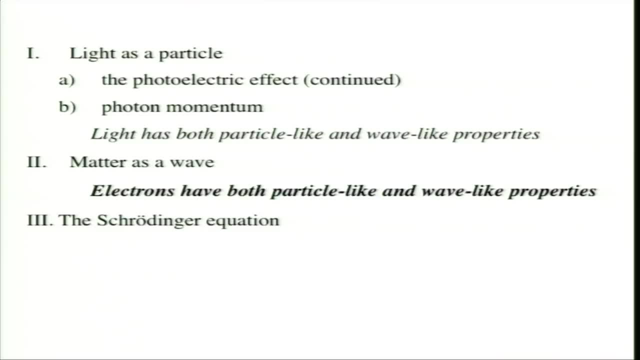 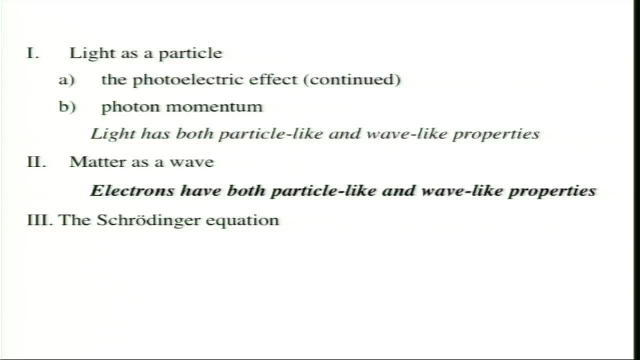 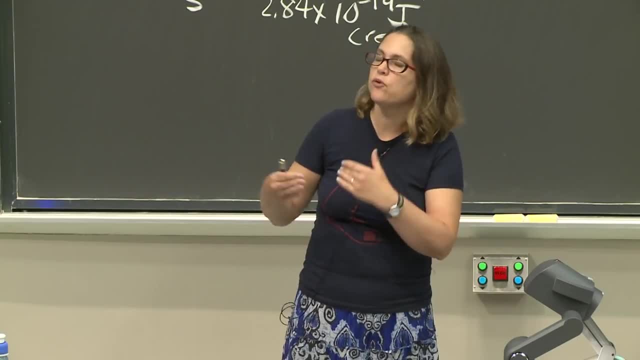 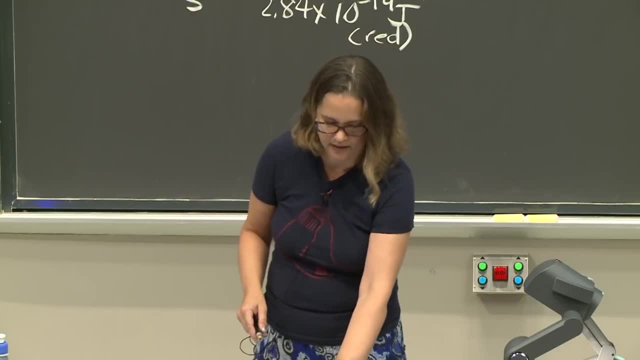 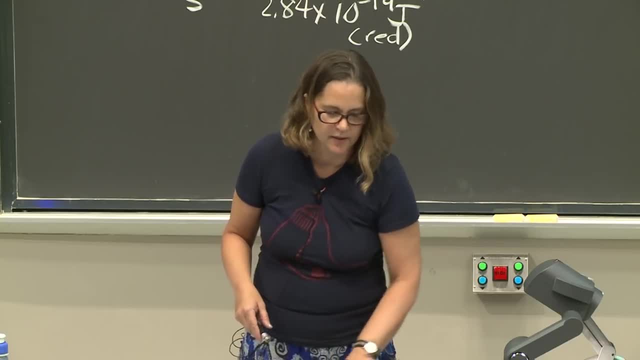 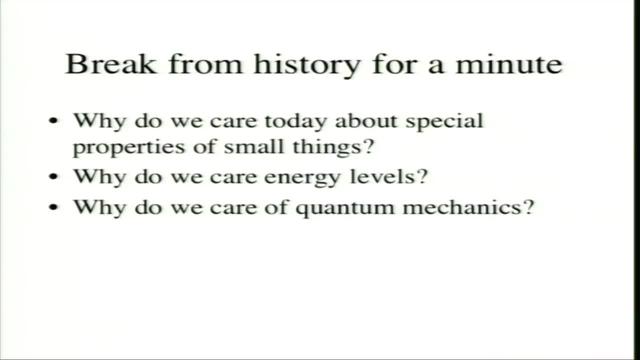 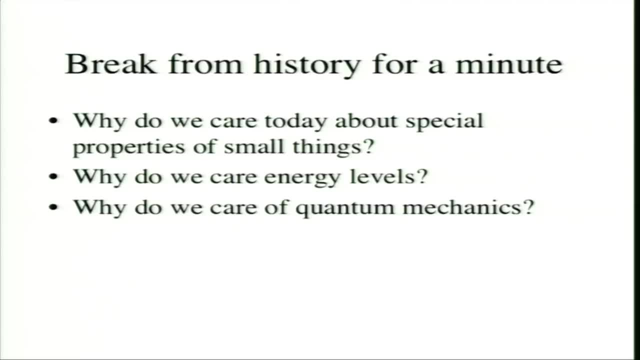 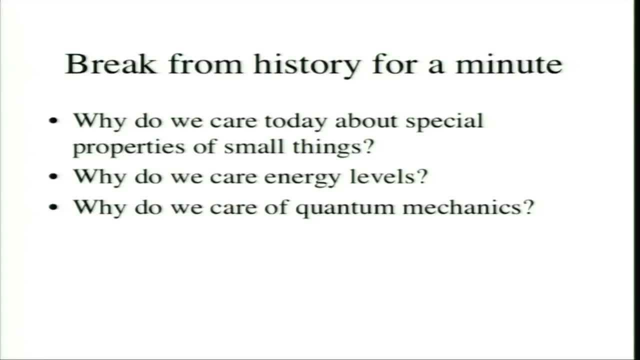 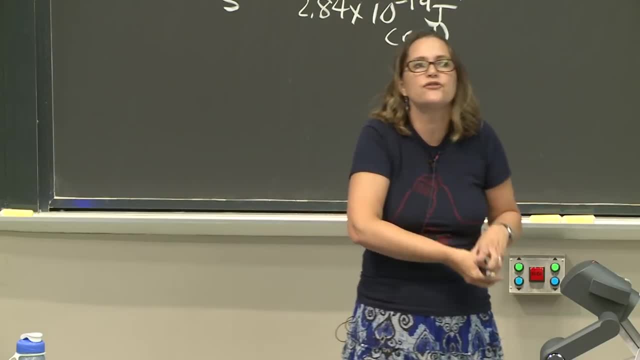 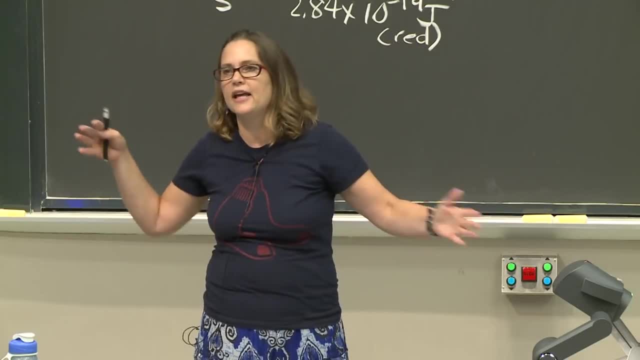 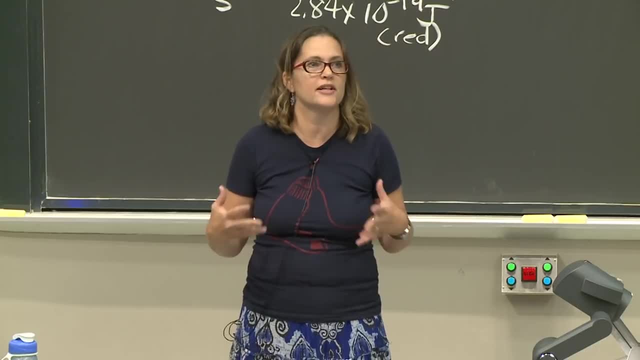 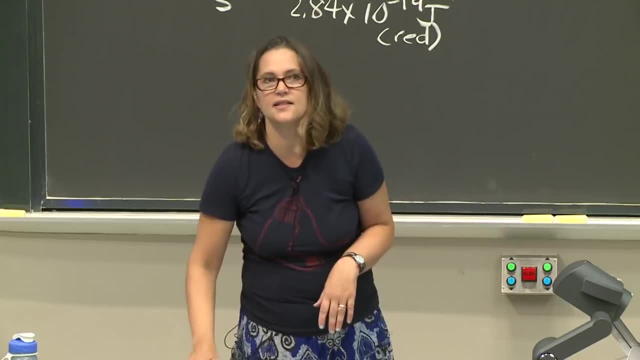 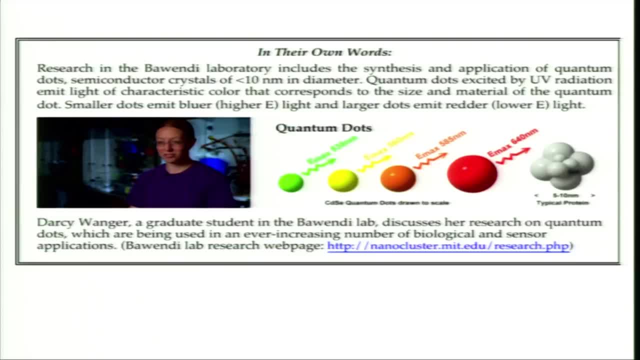 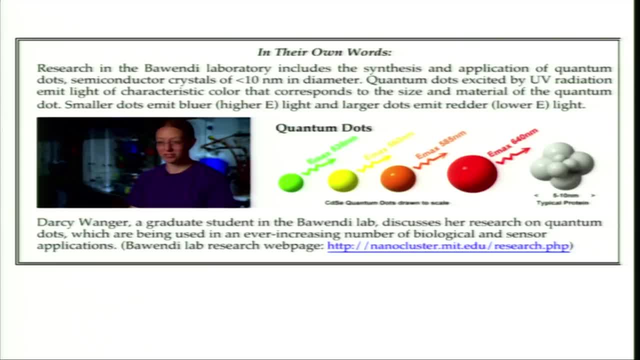 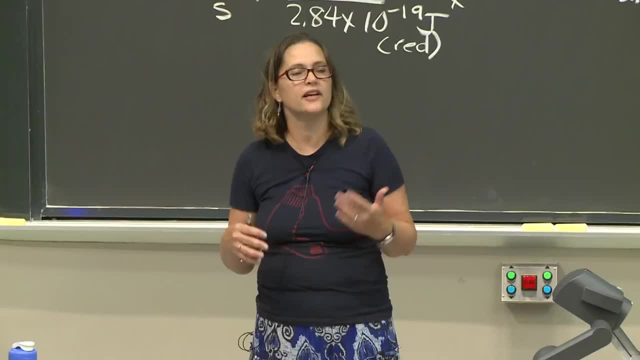 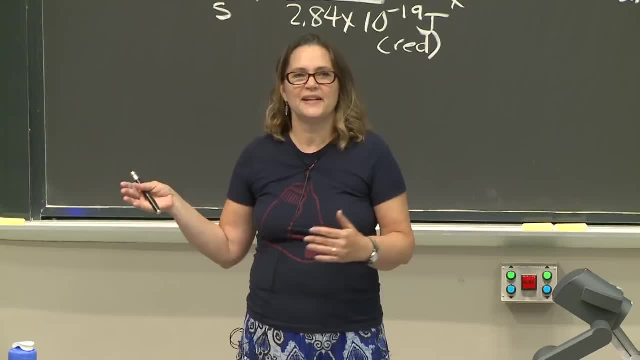 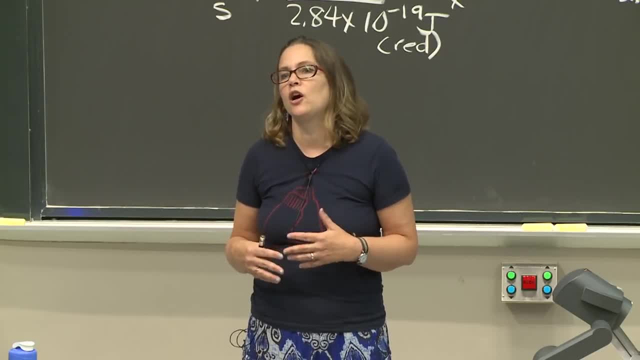 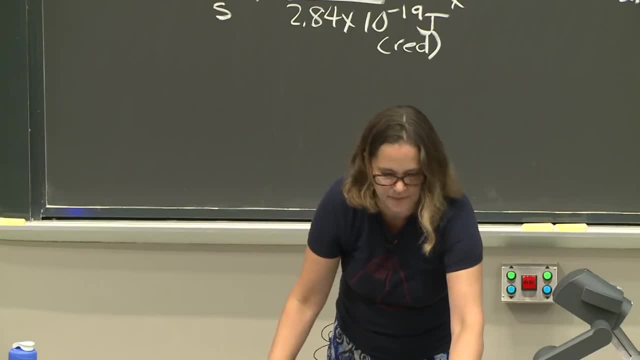 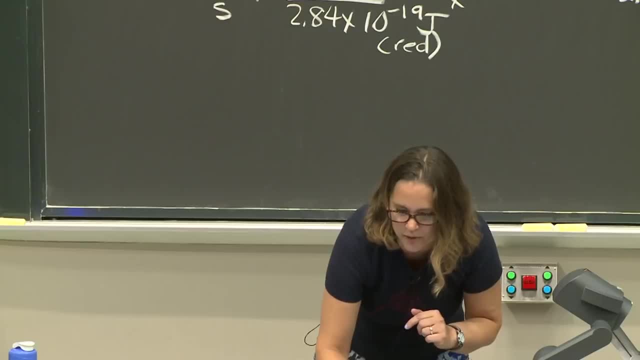 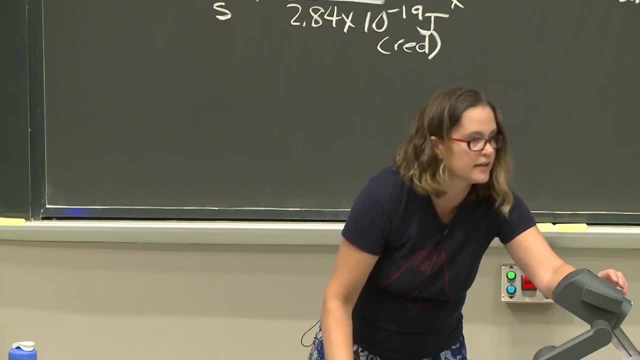 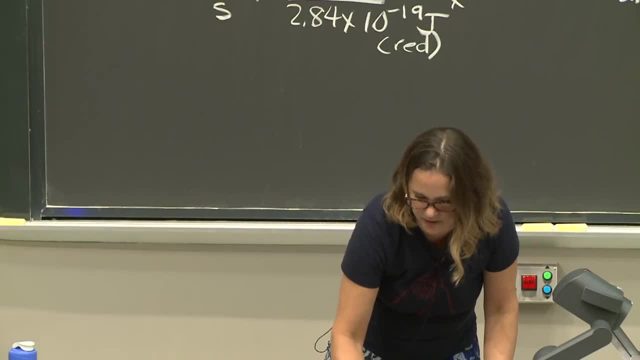 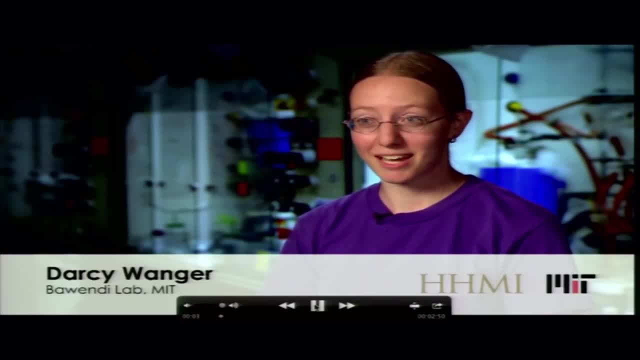 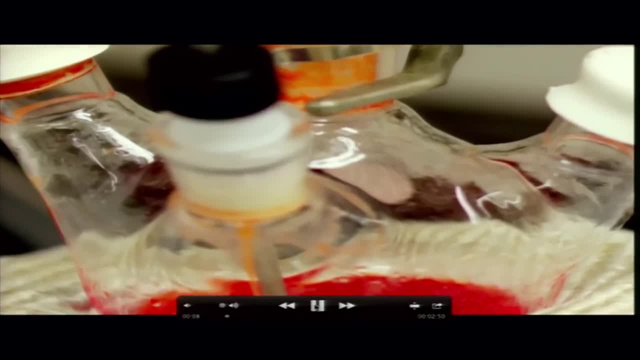 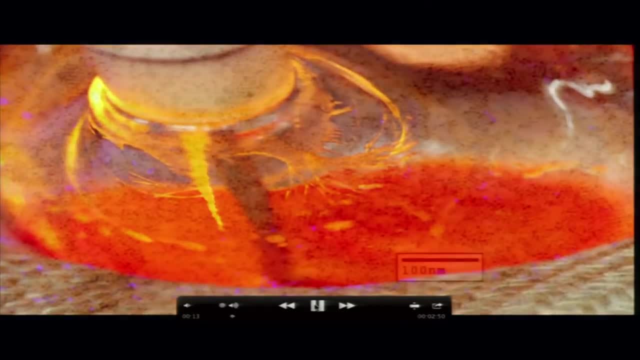 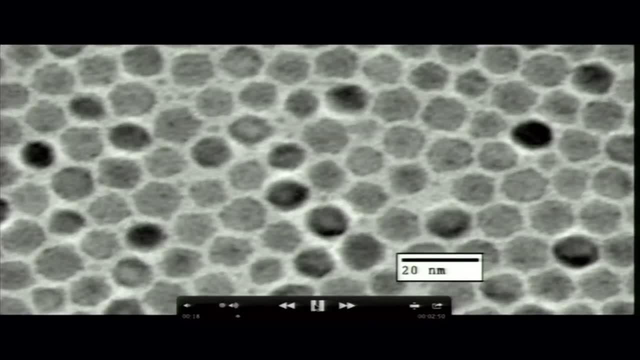 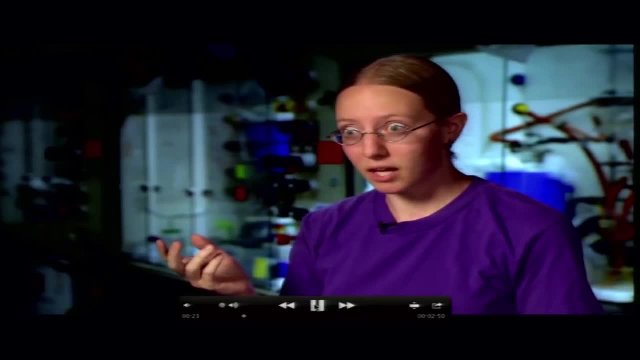 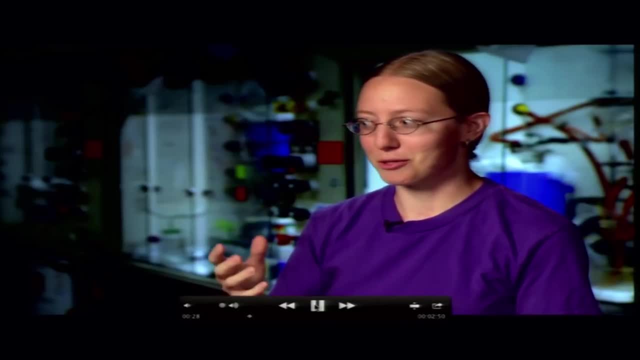 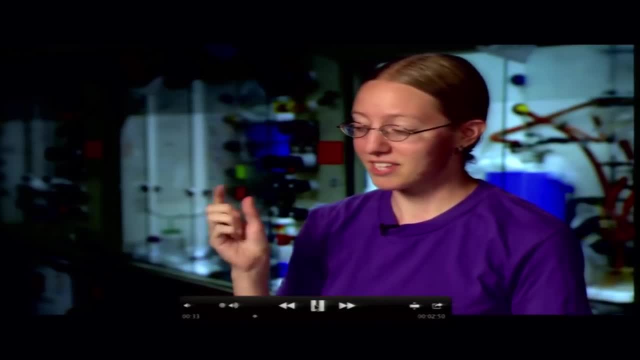 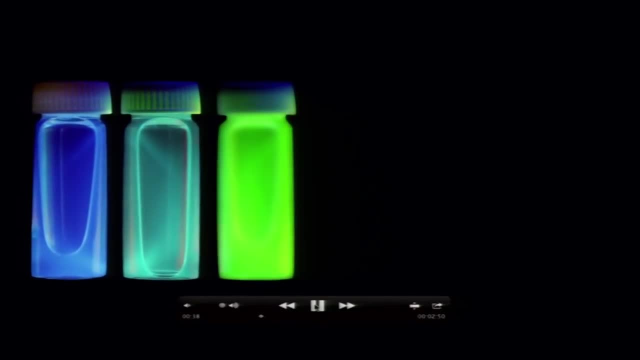 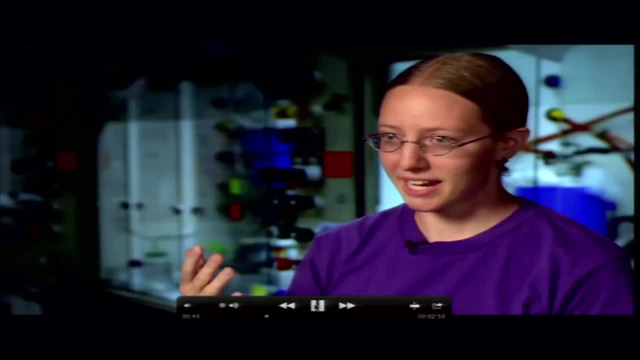 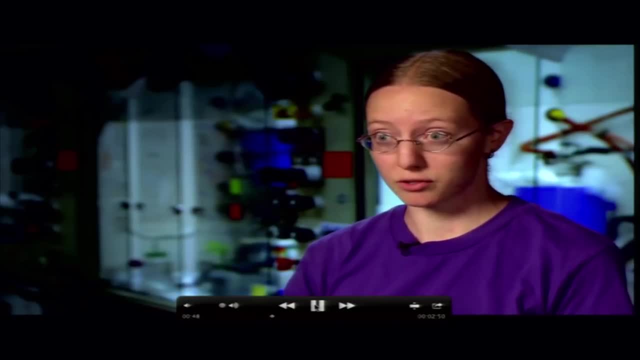 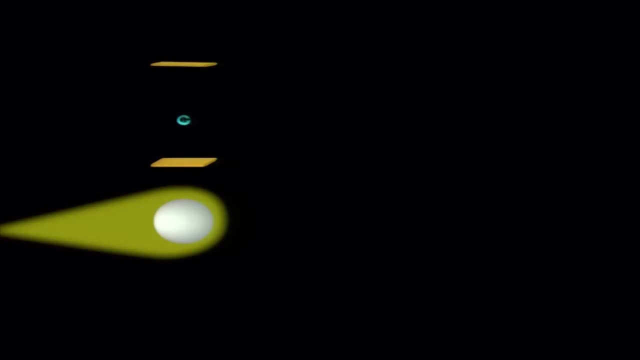 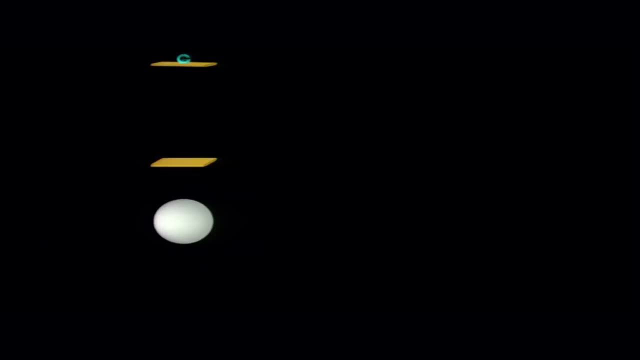 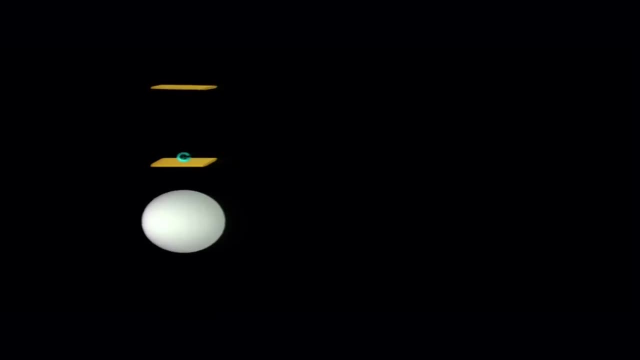 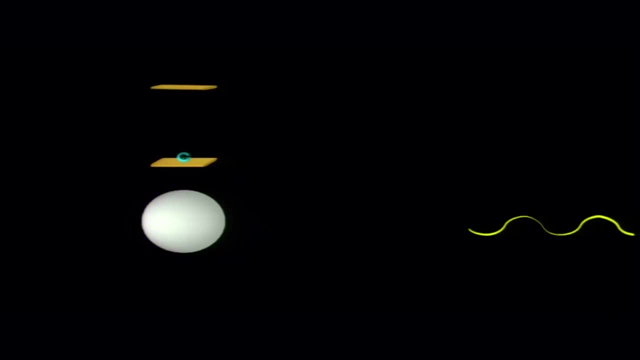 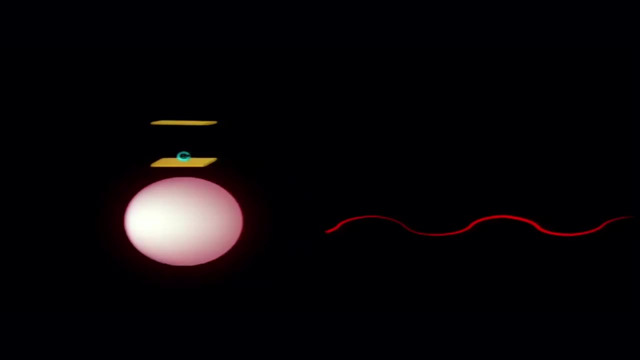 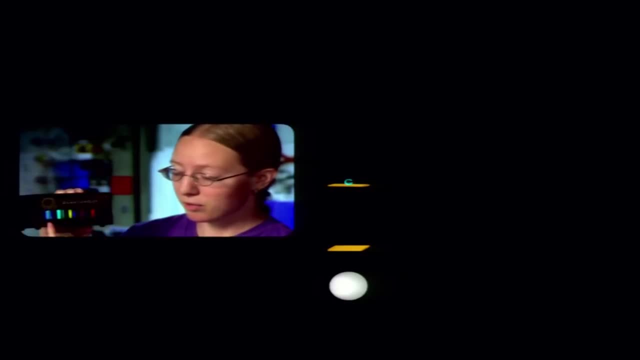 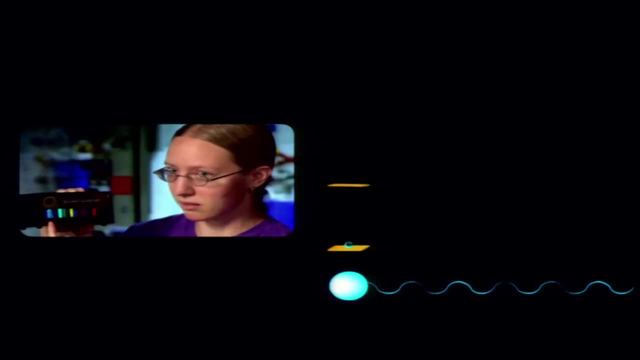 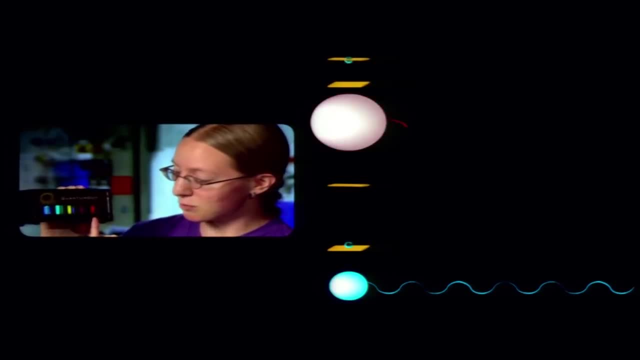 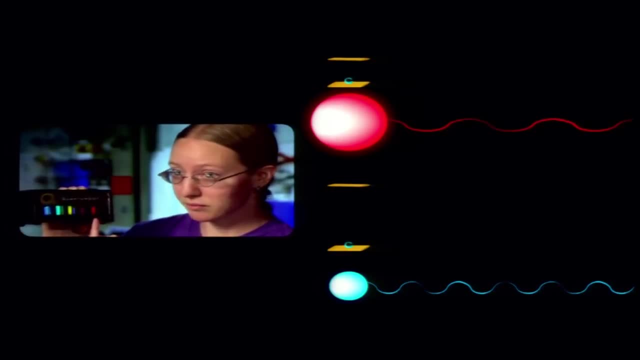 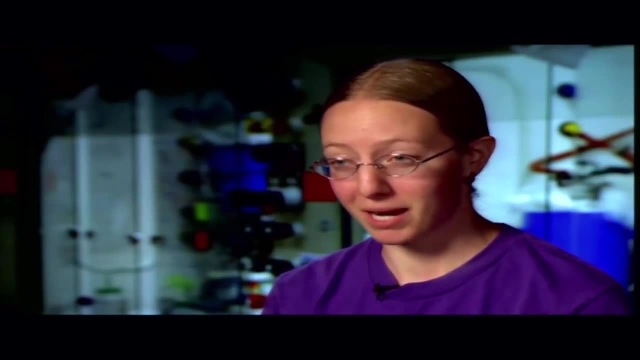 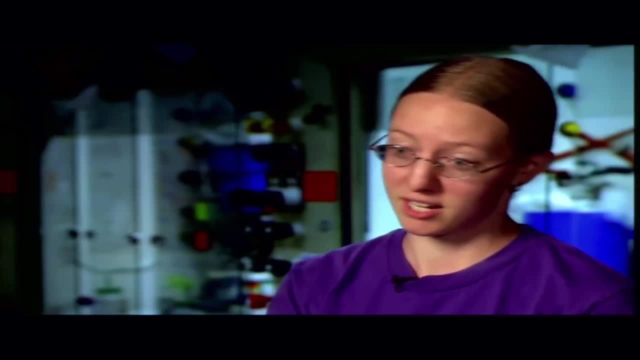 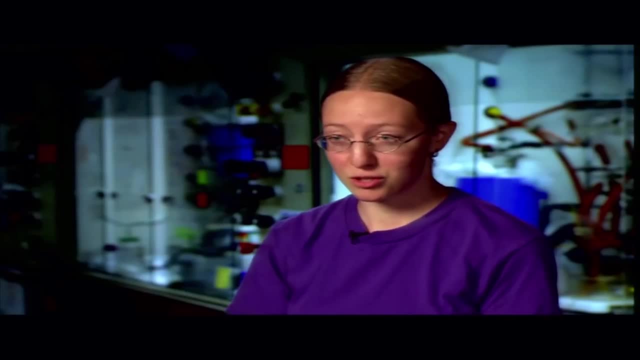 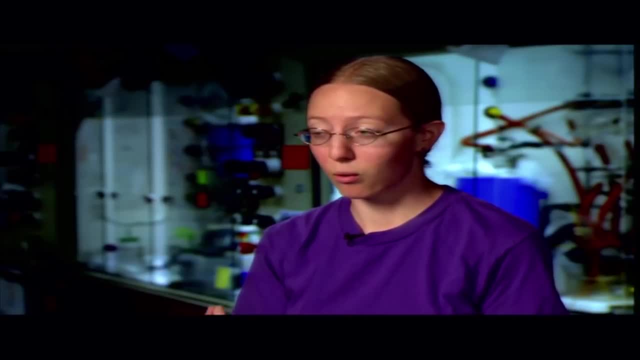 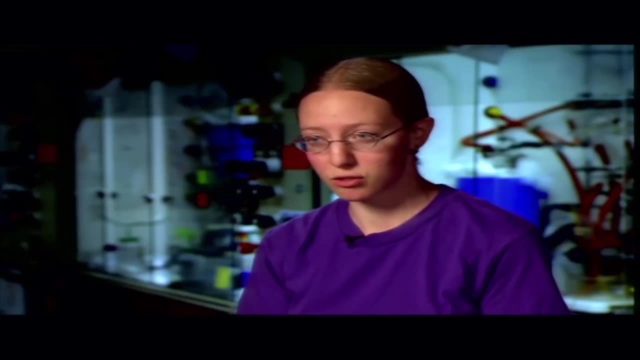 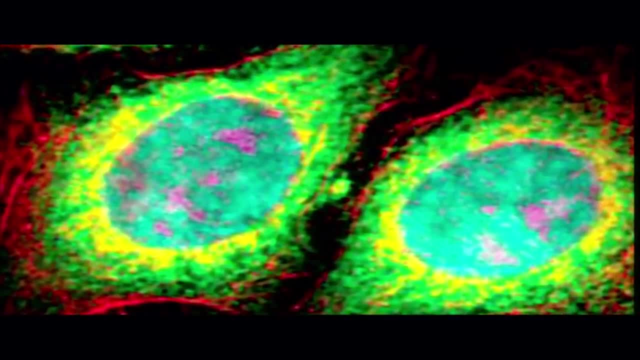 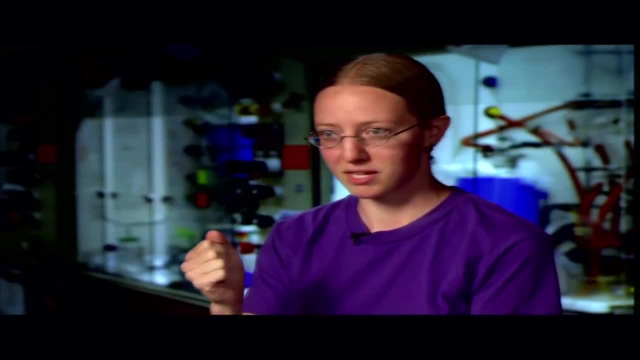 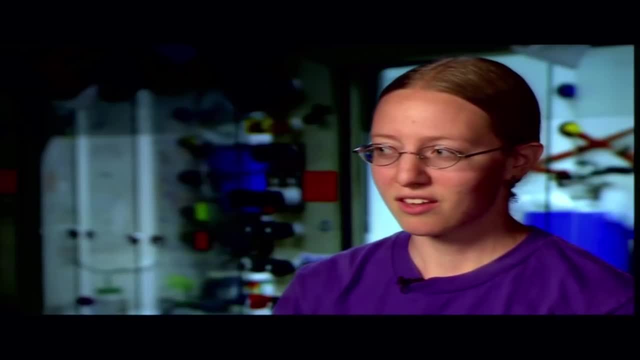 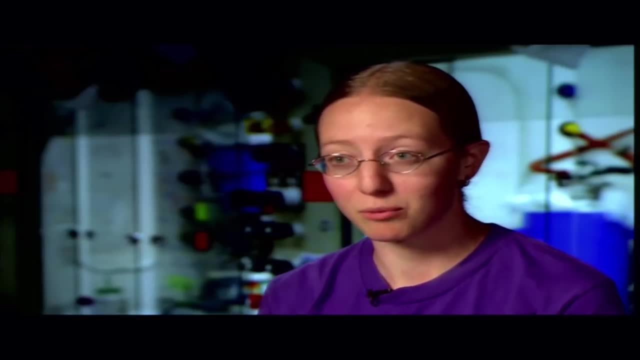 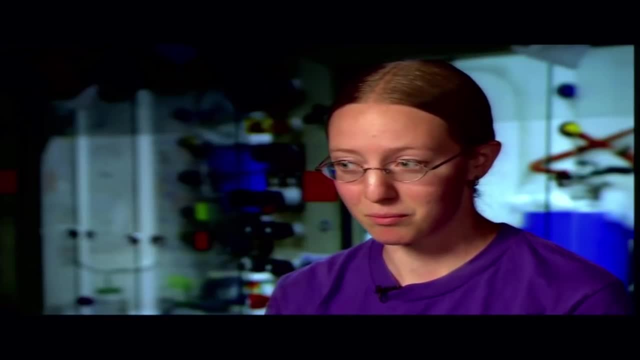 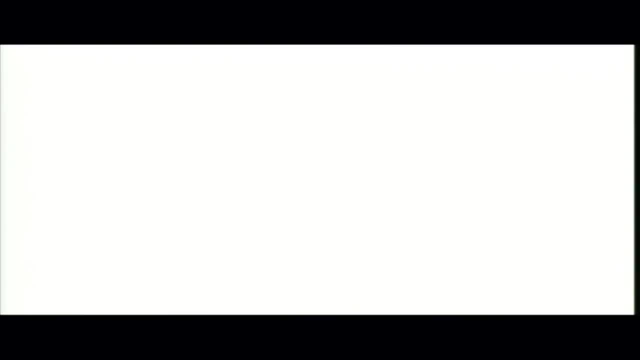 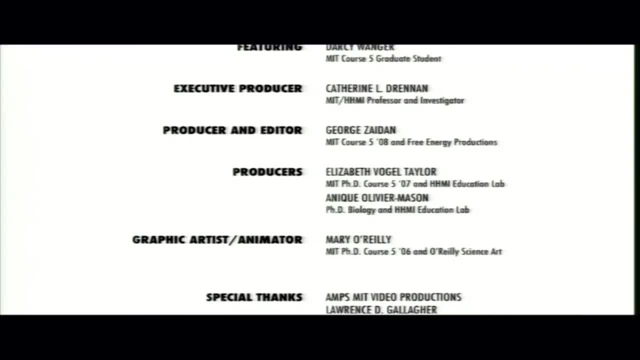 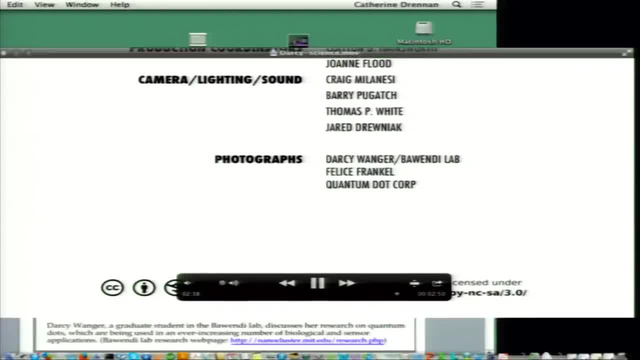 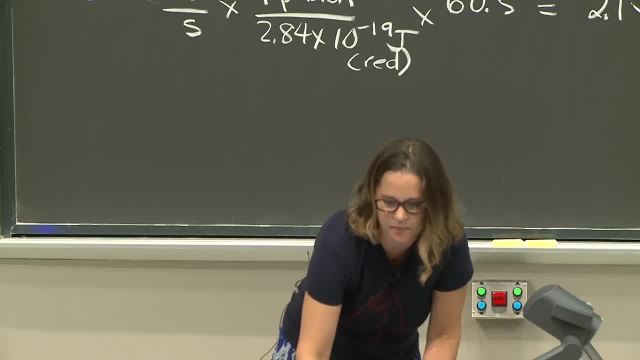 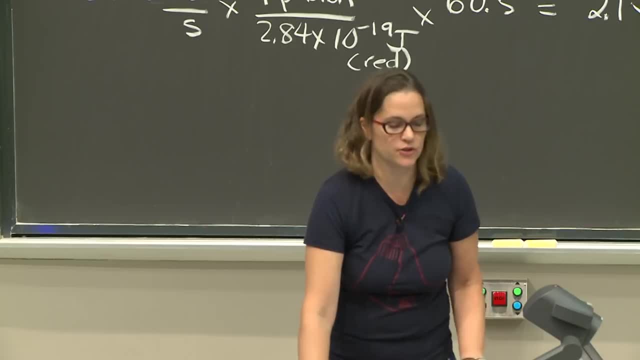 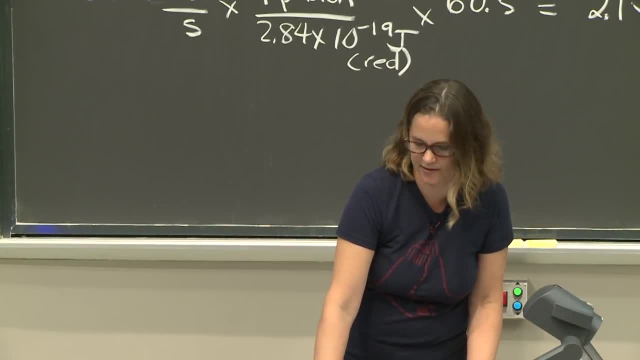 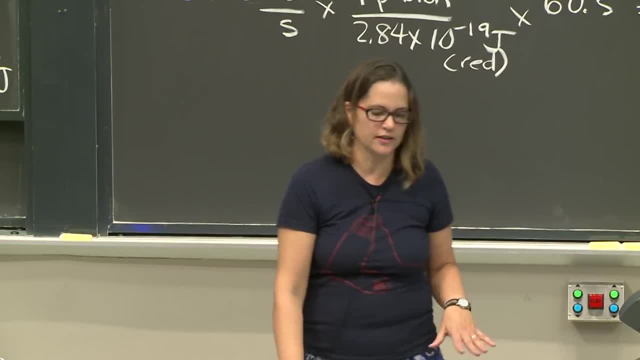 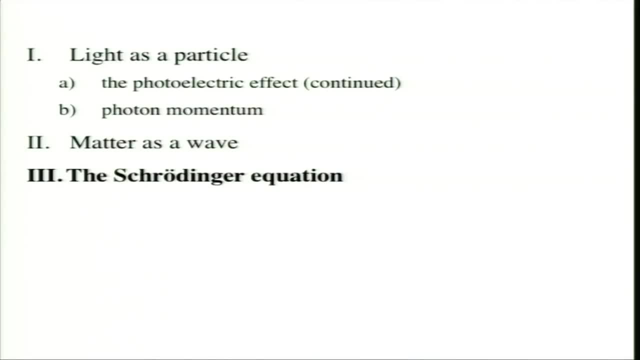 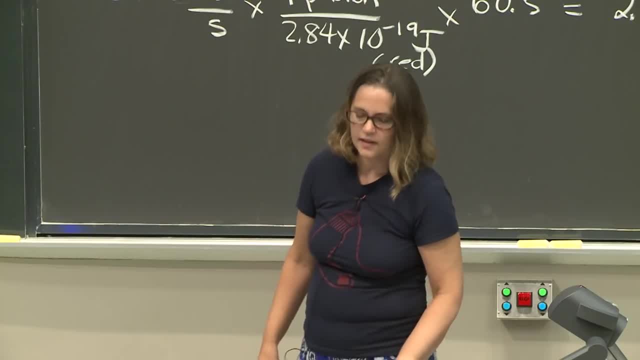 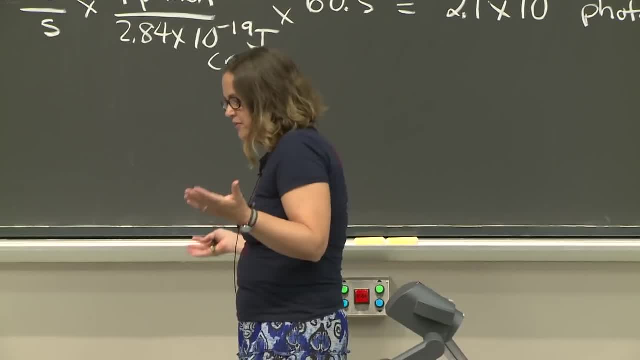 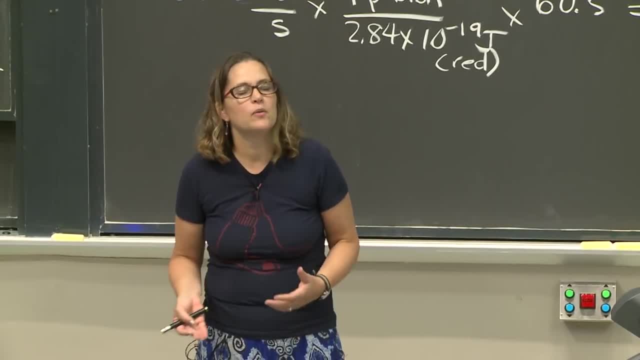 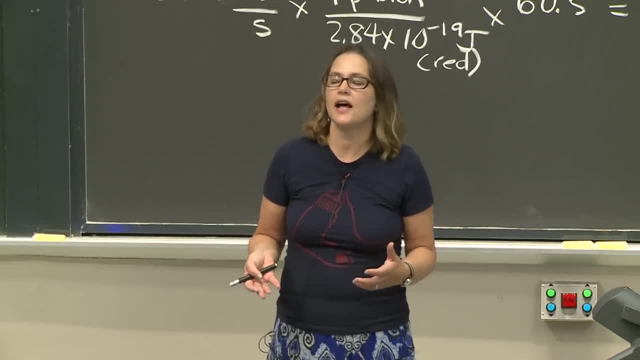 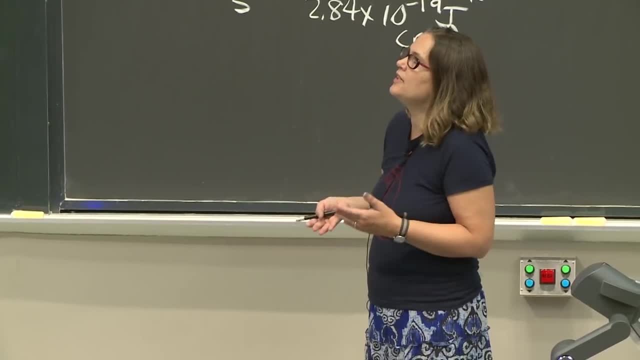 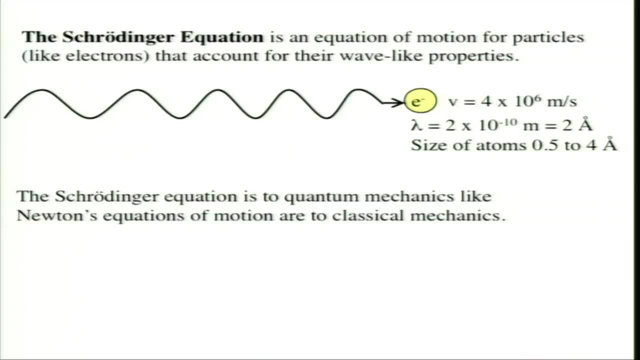 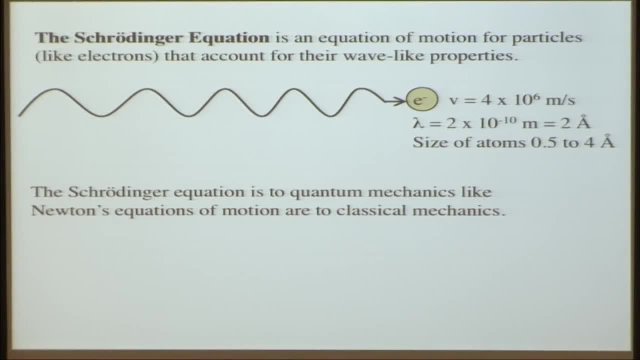 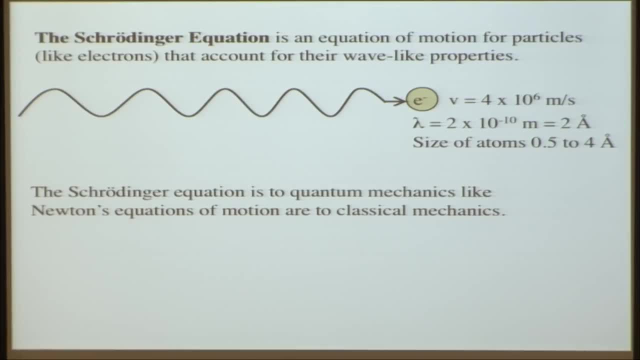 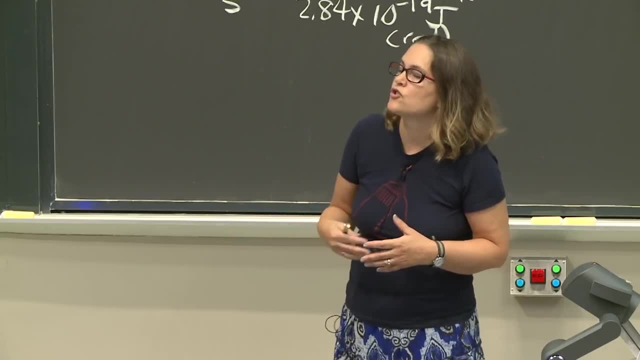 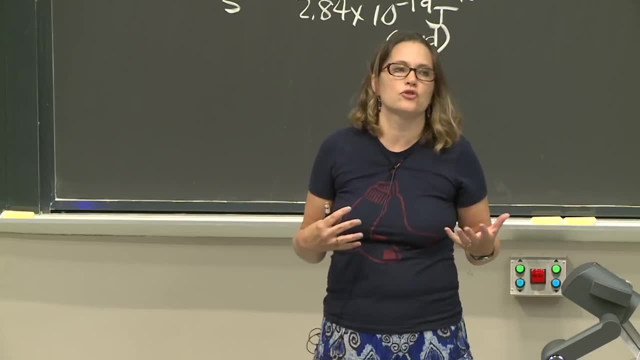 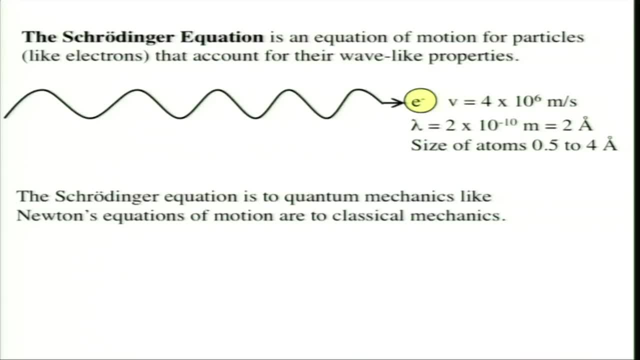 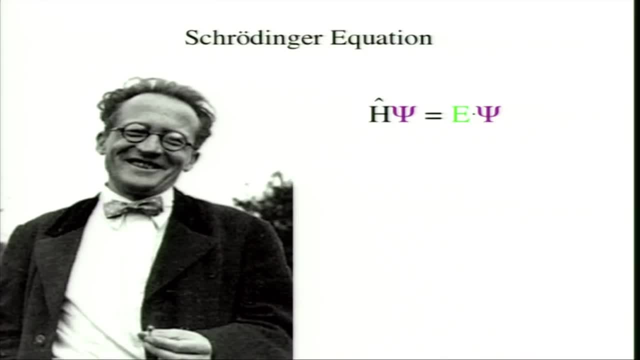 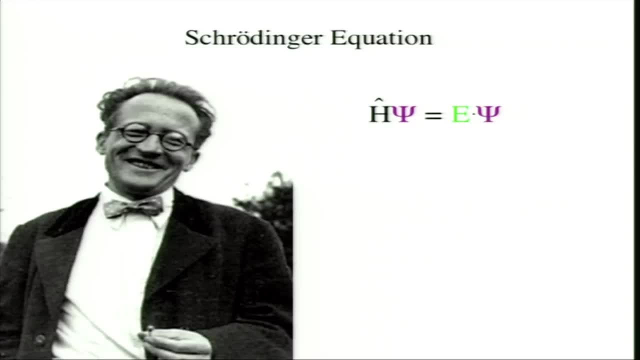 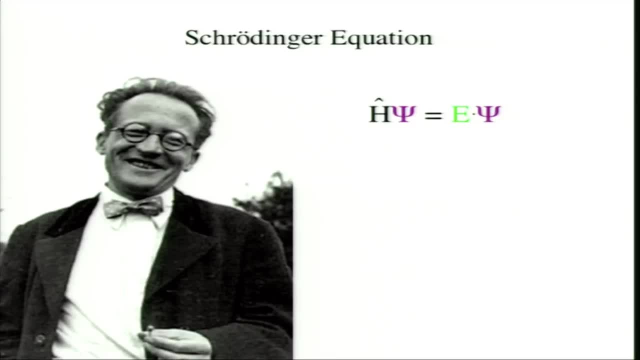 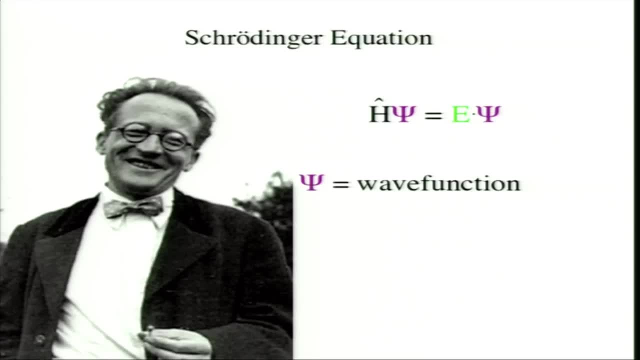 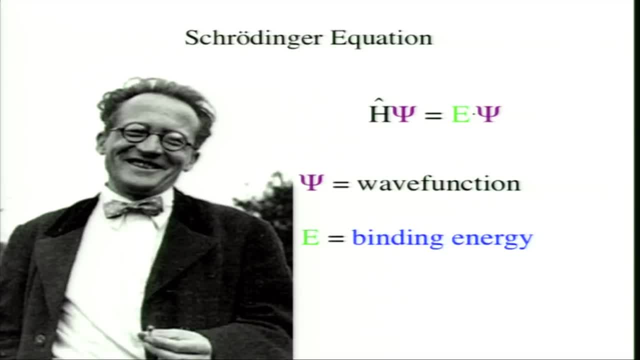 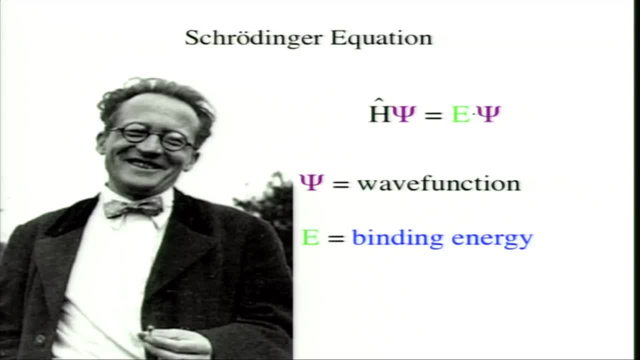 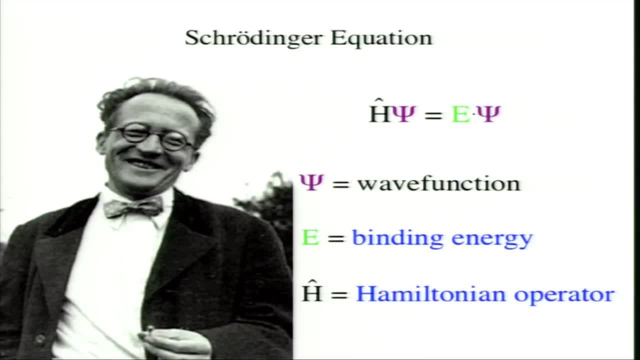 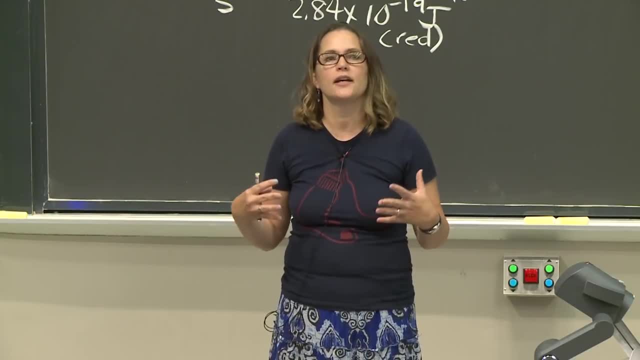 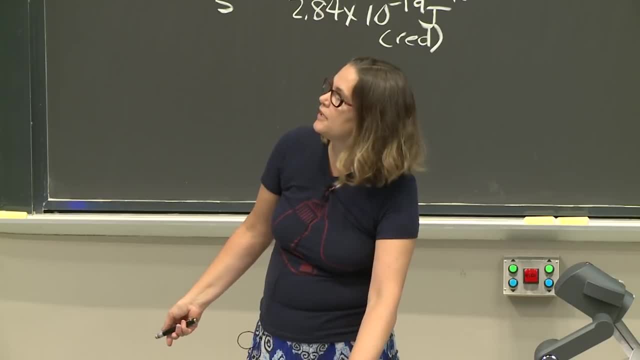 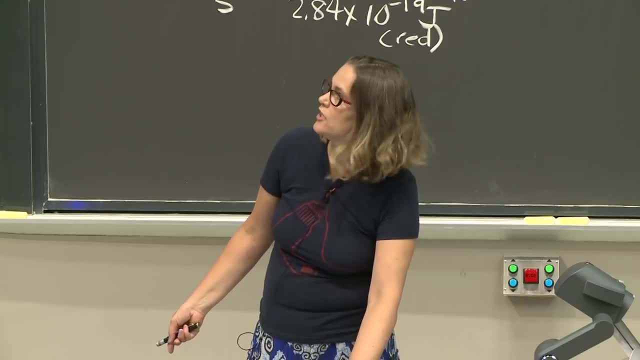 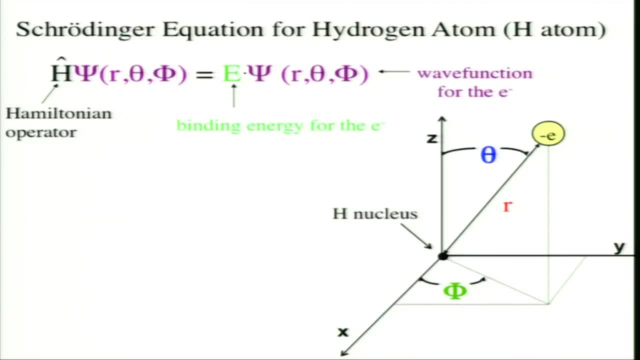 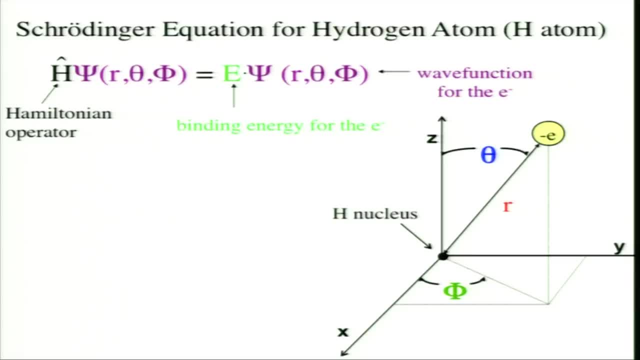 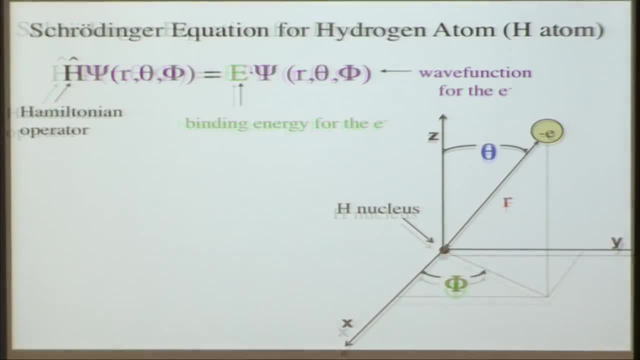 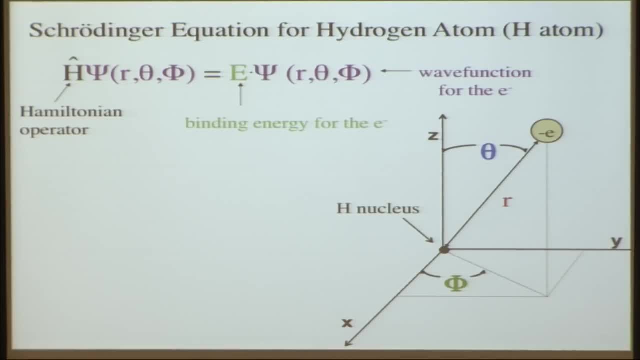 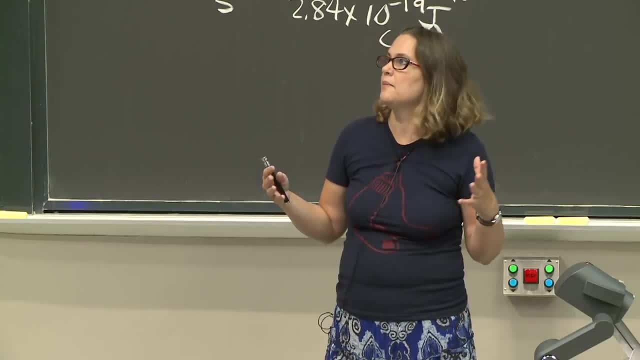 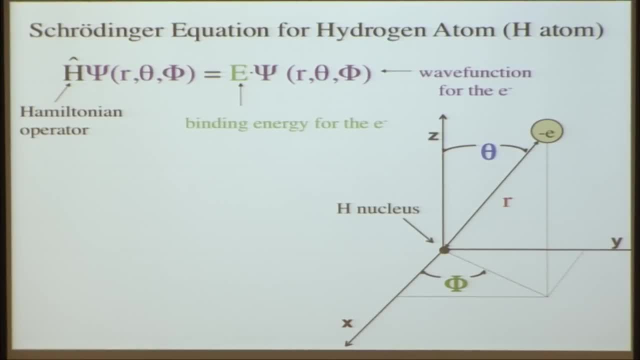 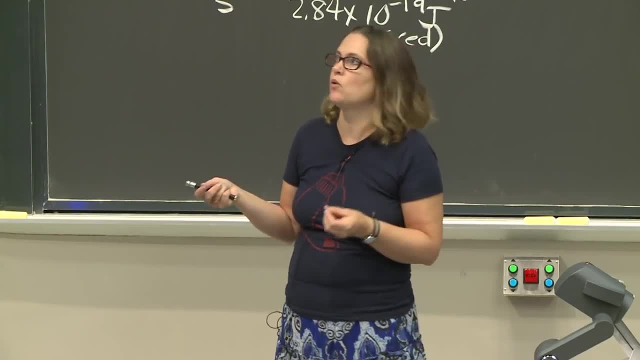 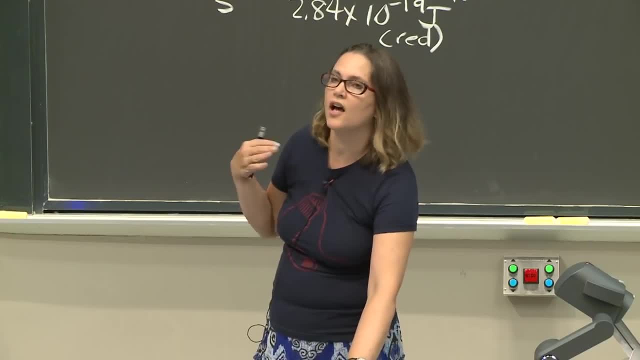 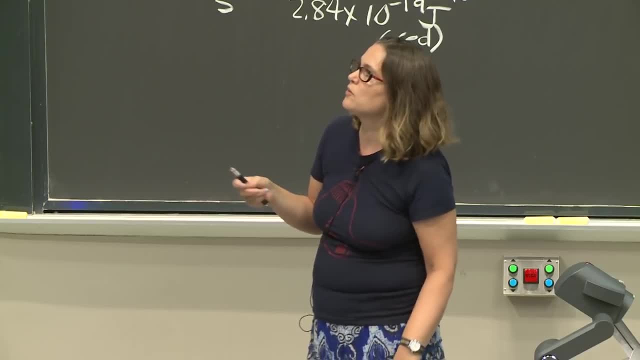 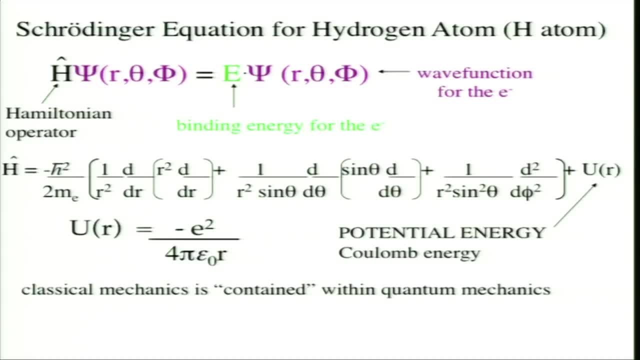 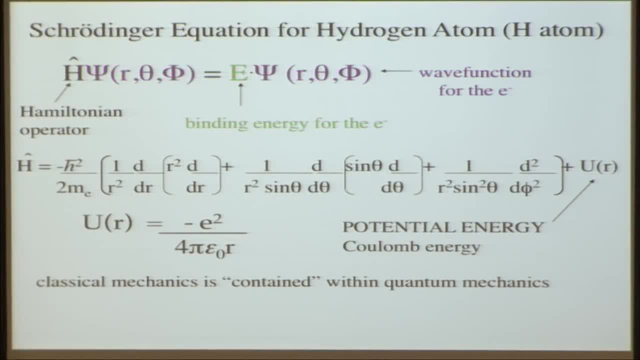 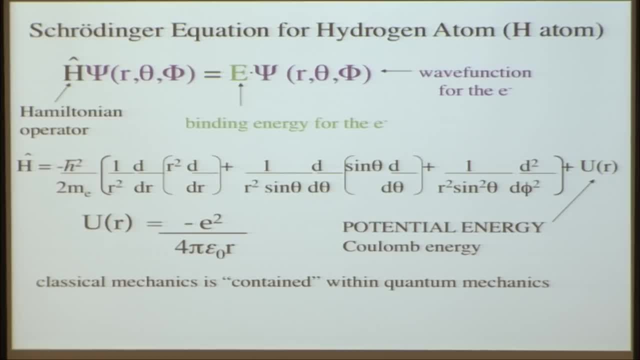 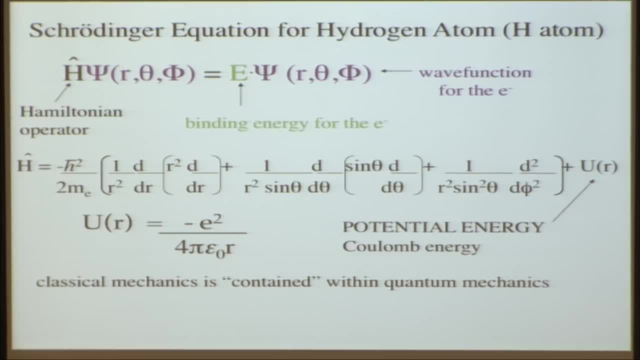 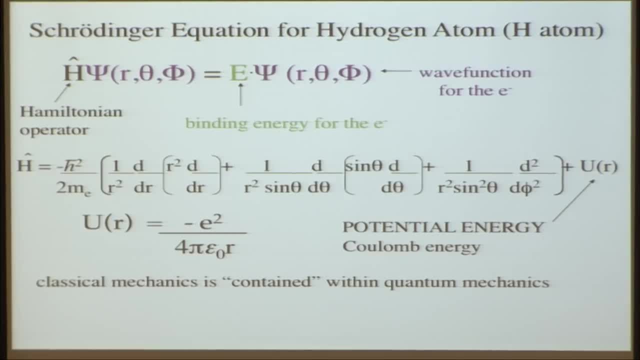 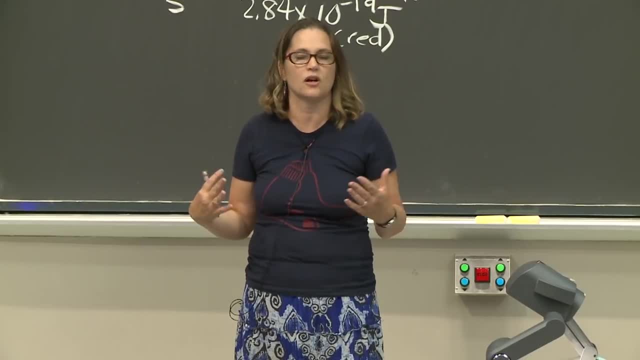 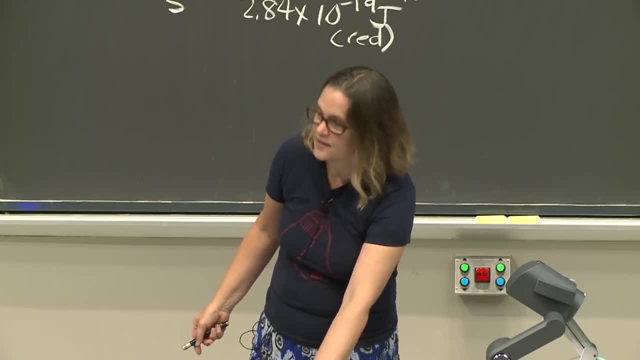 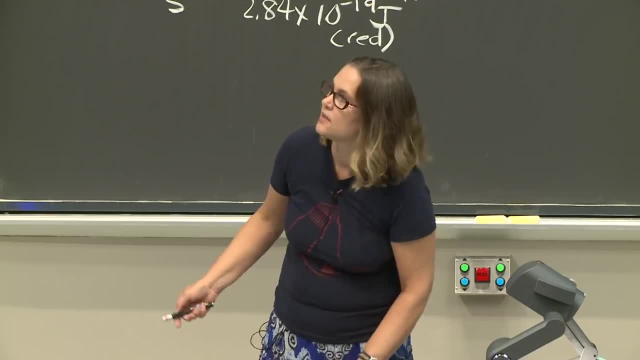 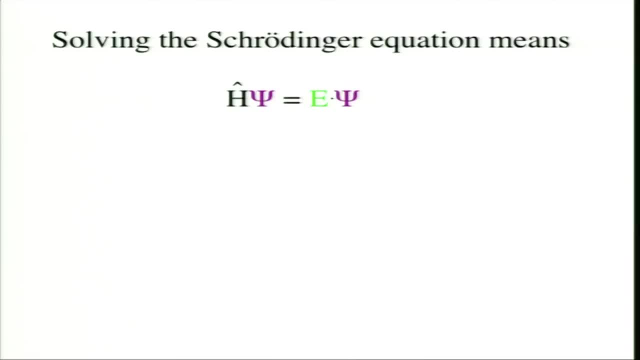 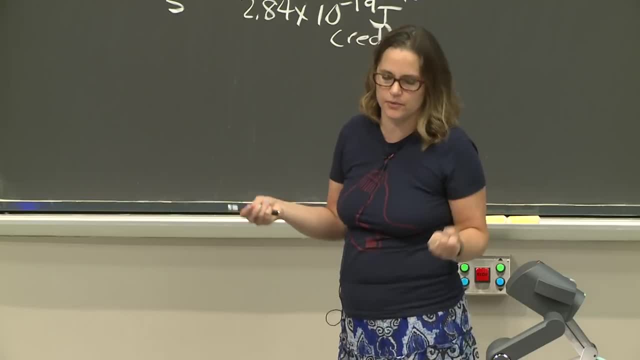 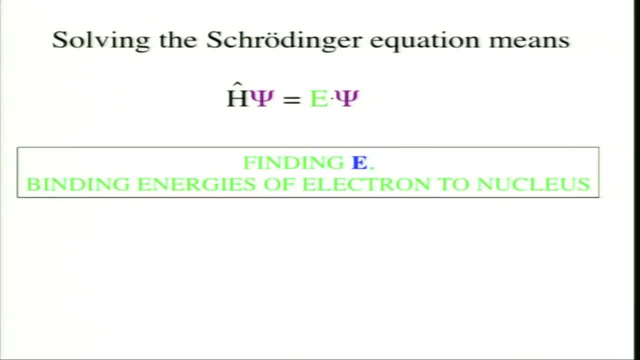 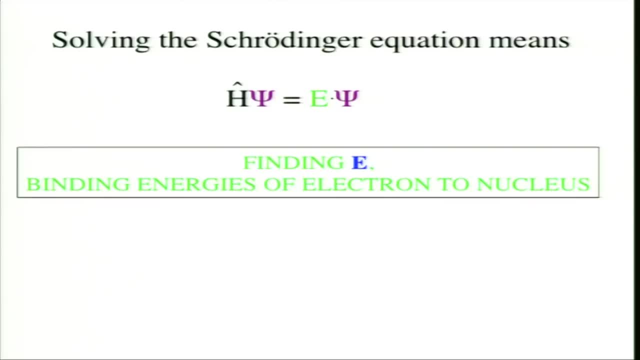 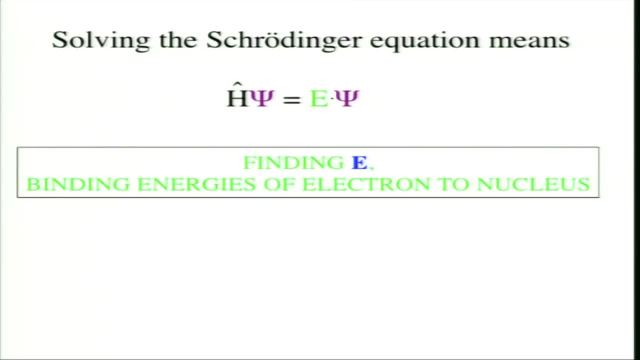 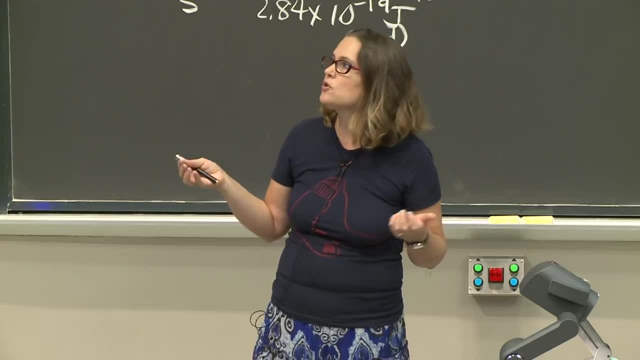 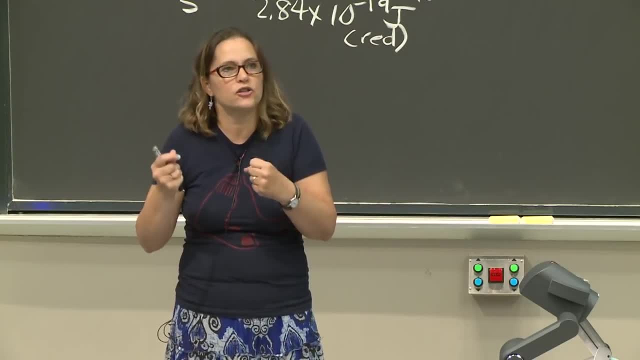 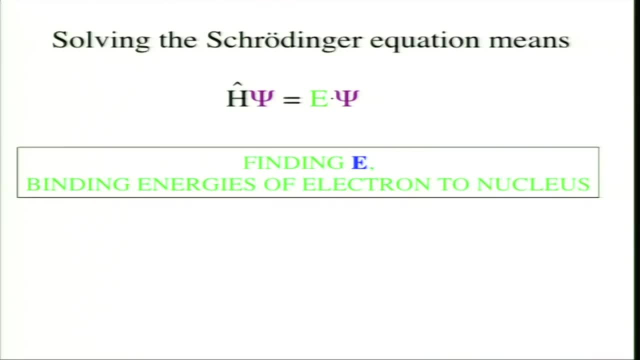 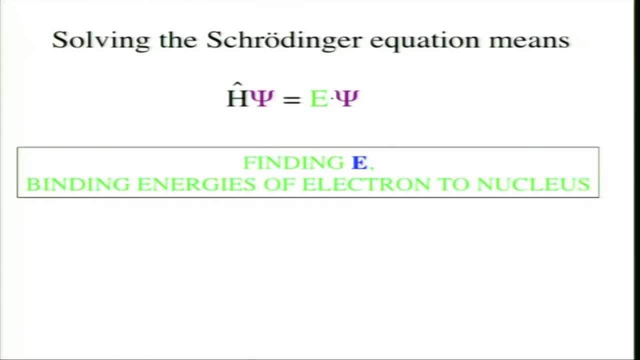 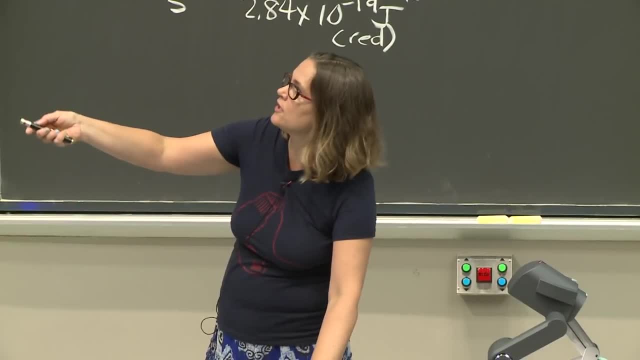 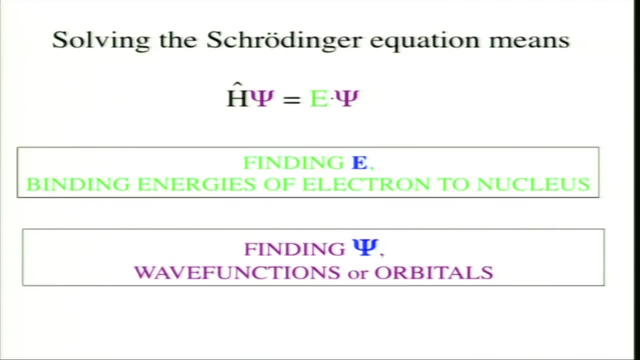 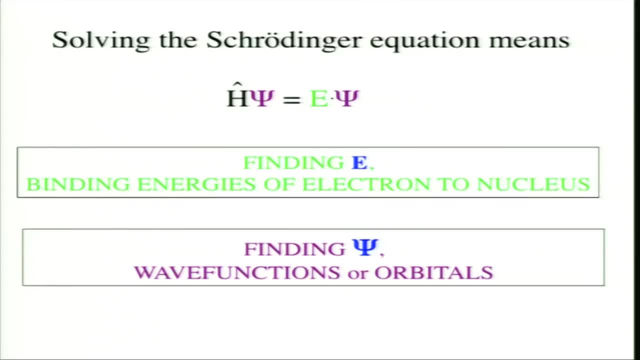 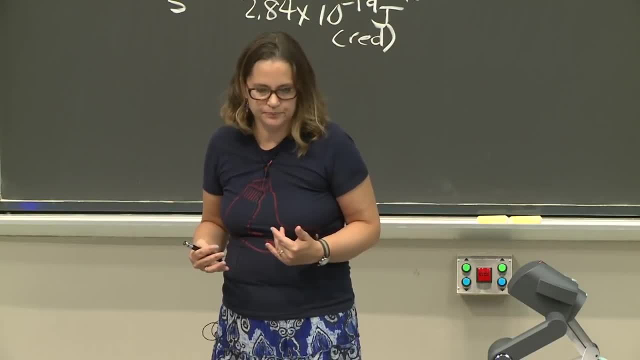 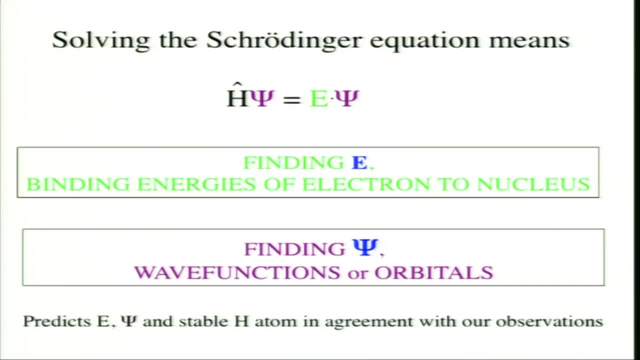 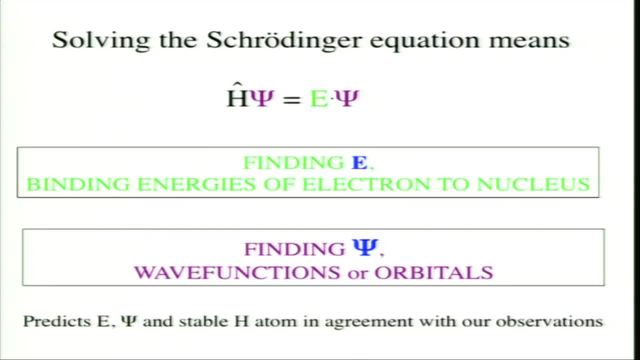 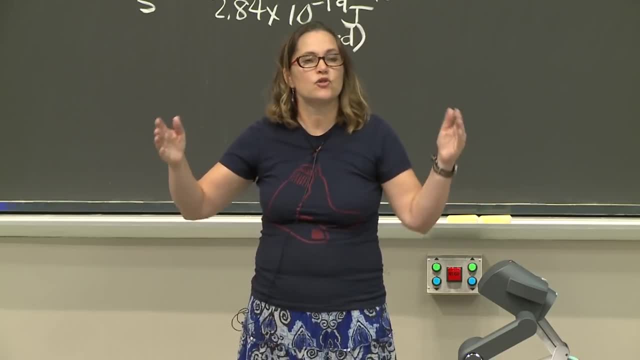 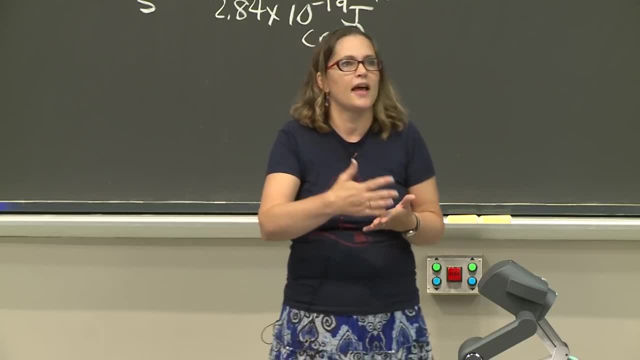 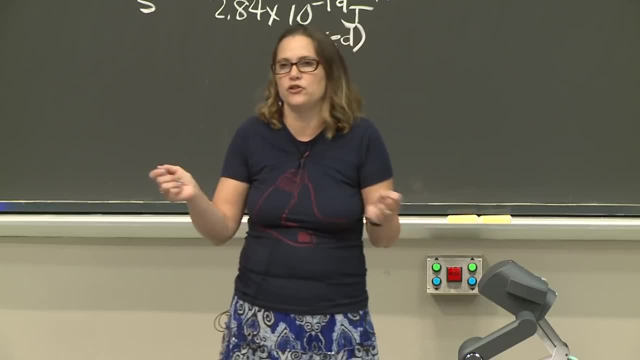 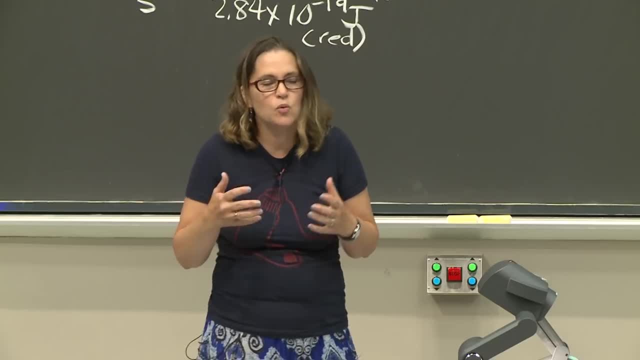 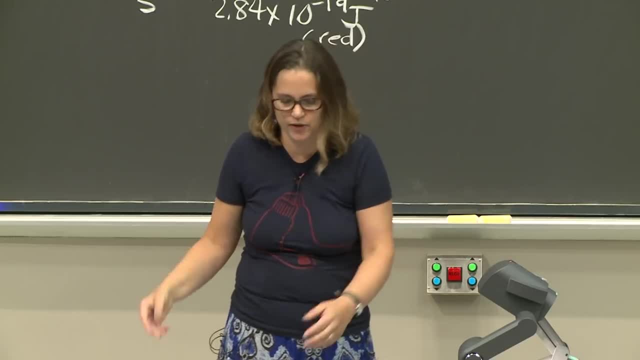 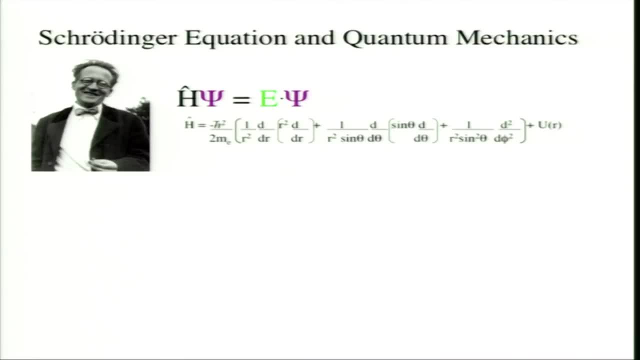 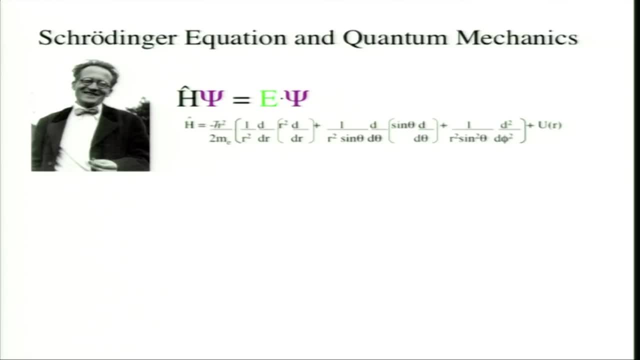 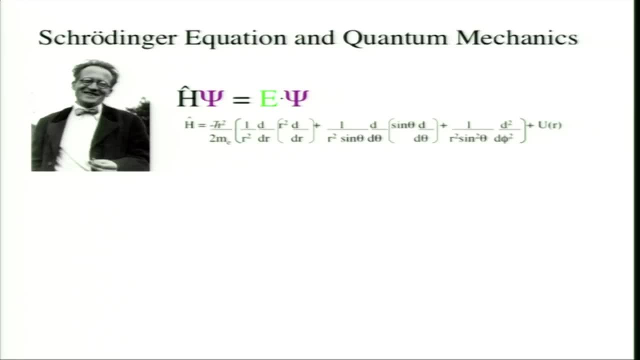 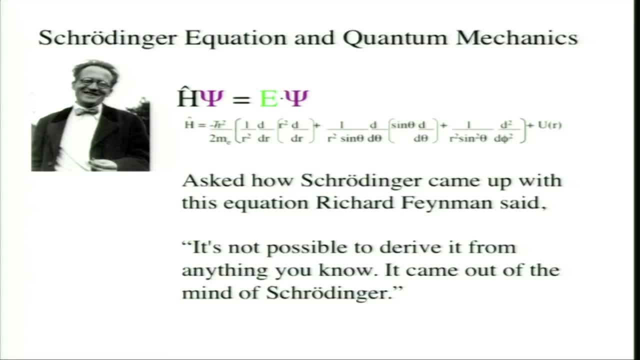 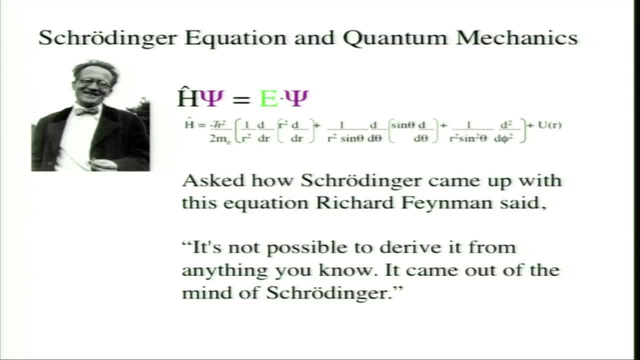 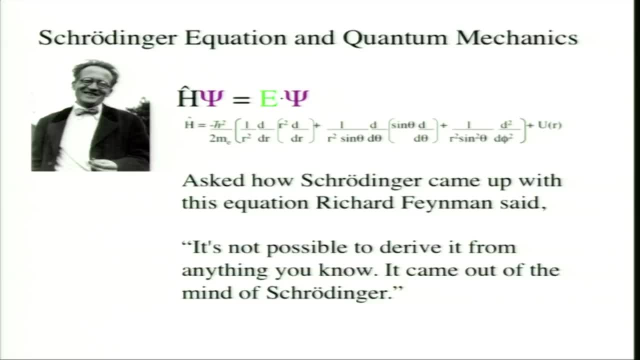 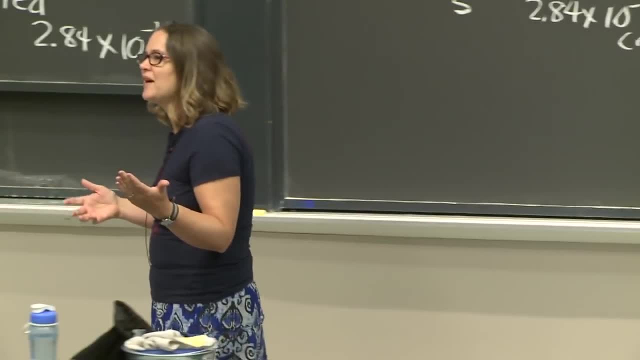 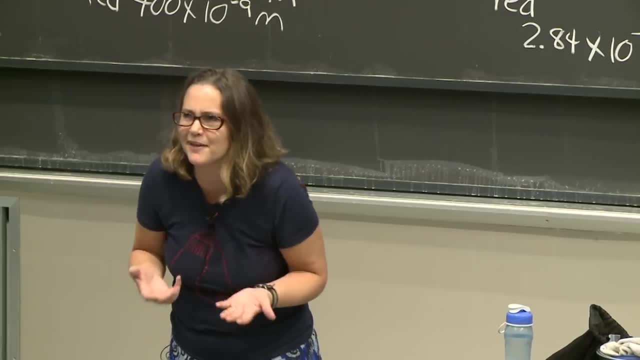 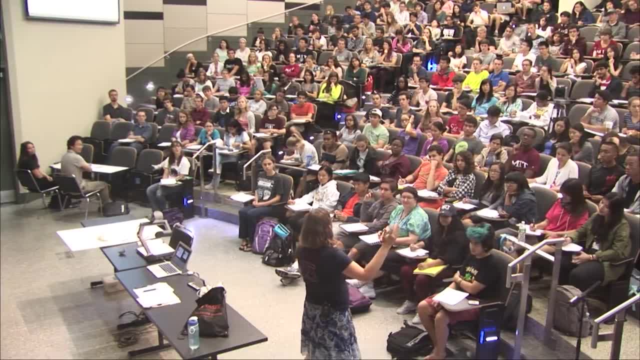 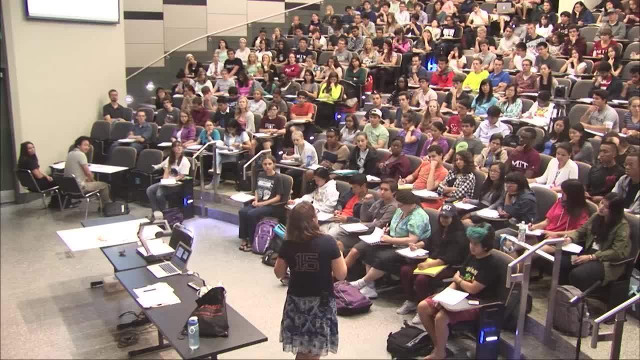 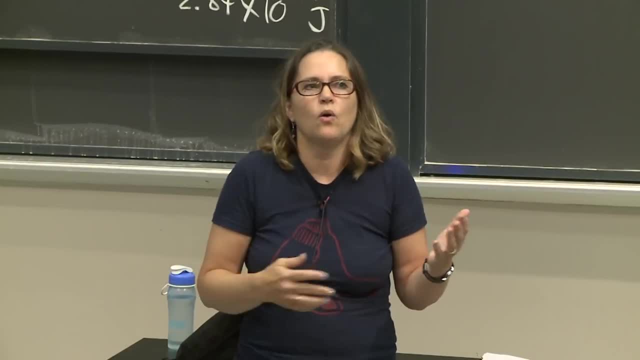 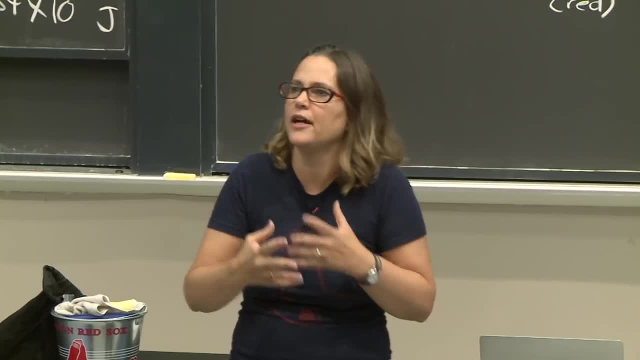 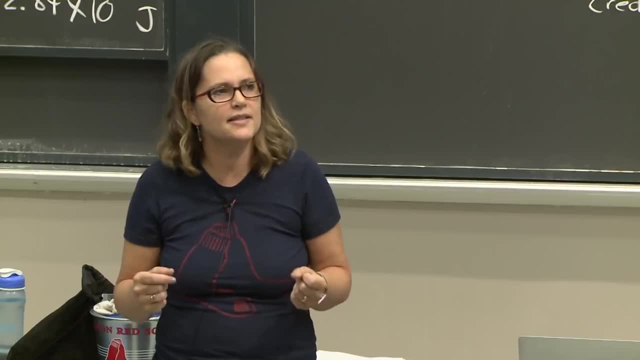 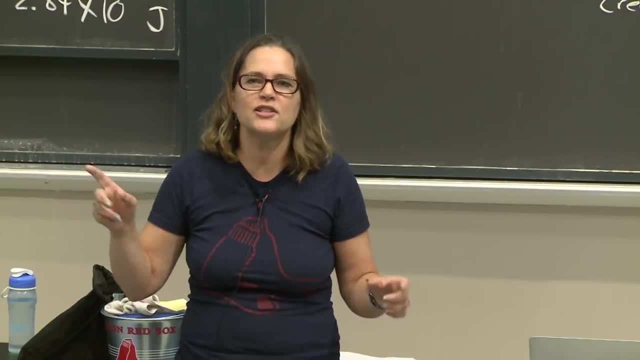 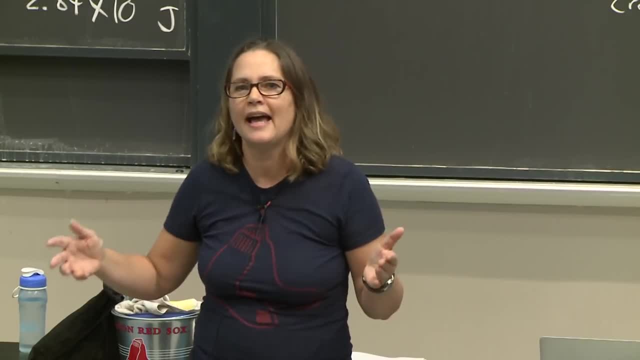 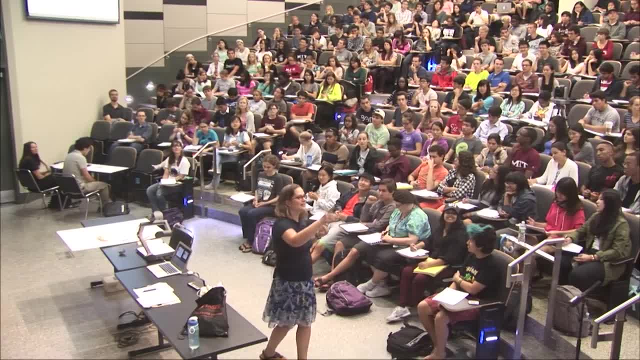 All right, let's see if we have any questions. All right, let's see if we have any questions. Okay, let's have a look at this. She asked the question to me And I've never. really that's the best explanation I have. 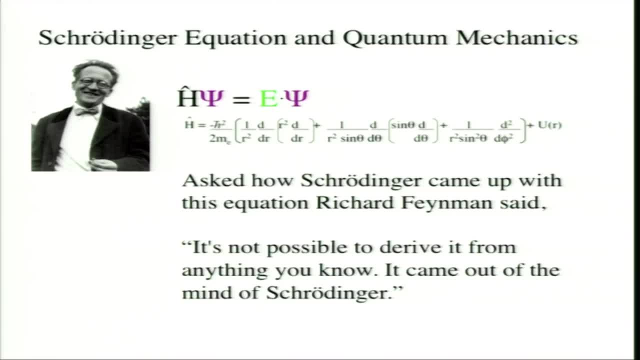 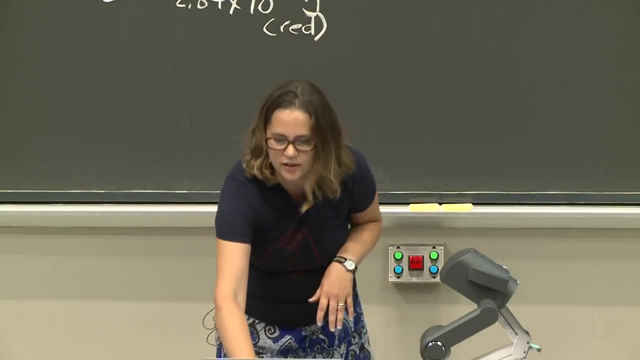 It just came out of his mind. Okay, so we're many years later. We've had the Schrodinger equation for a while, So this is, you know, an old story. Well, maybe for the hydrogen atom, But this is still actually a very active area of research. 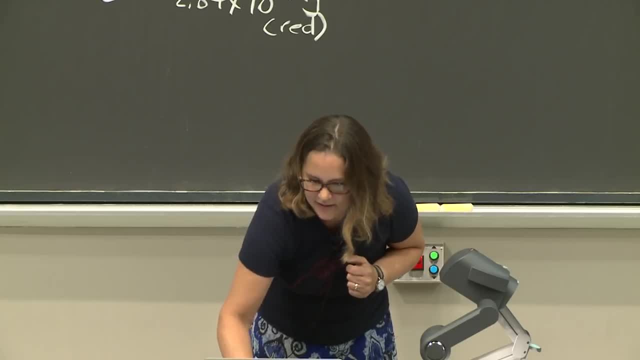 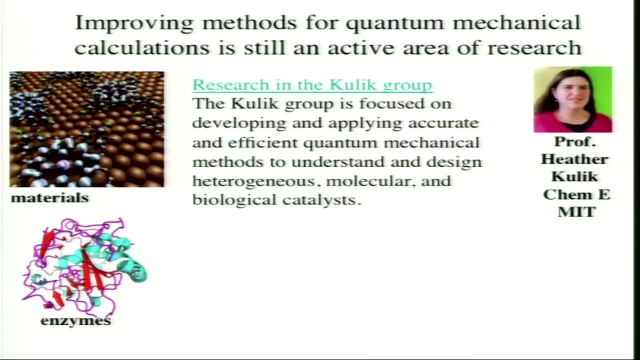 Oh, my startup disk is full, Thank you, Let's go back to that, All right. So I just thought I always like to give you examples of kind of current research on these areas, And so I know a number of you are. 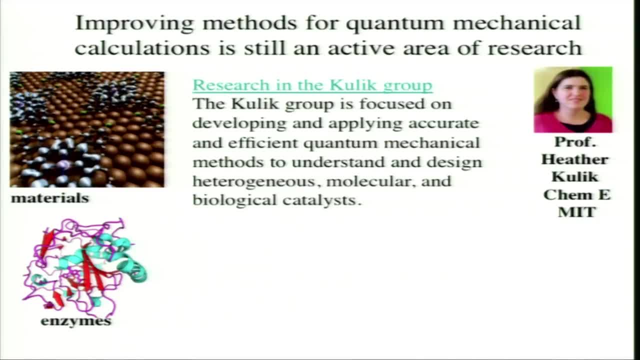 interested in potential being chemical engineering majors, undergrads. and I'll tell you about a new professor who started about a year ago: Heather Kulig, And her research group is really interested in using a quantum mechanical approach to study materials and to study proteins. 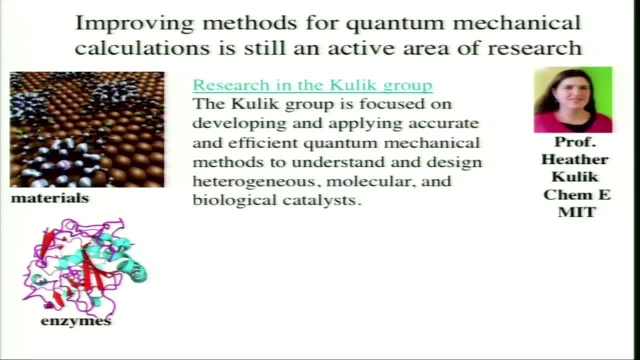 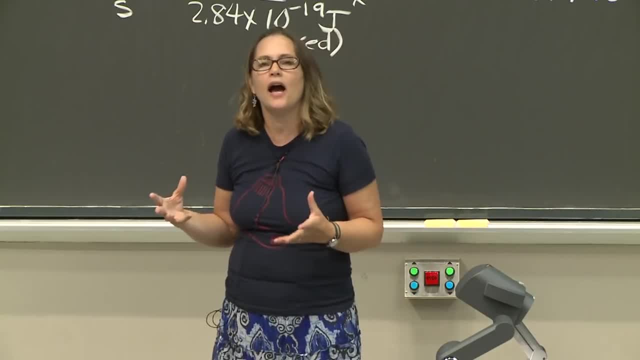 But when you get to things like proteins, there's thousands and thousands of atoms around. Forget multiple electrons. We're talking about multiple atoms with multiple electrons, huge complexes. How can you give a quantum mechanical analysis of things that are so large? And this is really important. 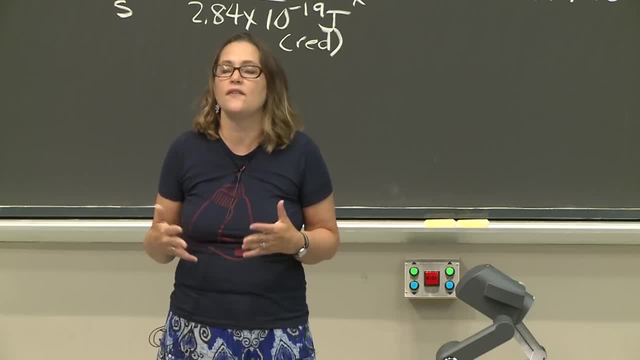 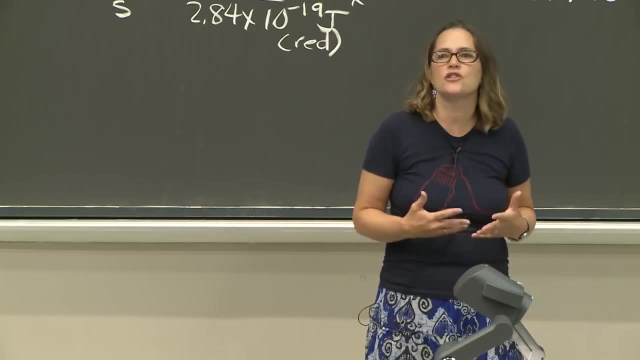 I mean, I think that one of the big problems moving forward is solving the energy problem and doing it in a way that doesn't destroy our environment. So new batteries, new electrodes, new materials. We need to understand the properties of different metals to understand what will make those good electrodes. 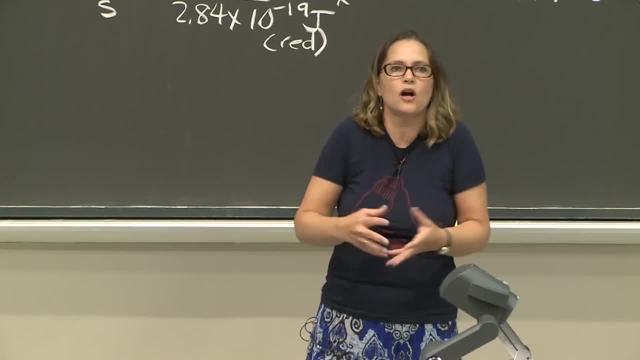 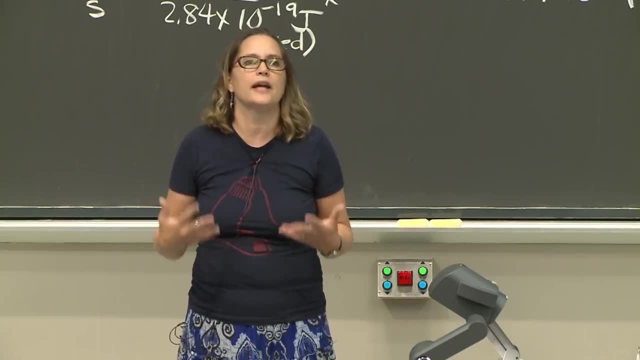 And to really understand them we need a quantum mechanical approach. But these are big problems, These are big areas. There's a lot of things to consider here. So Heather is interested in coming up with improving algorithms and improving the computation to really give a quantum mechanical analysis. 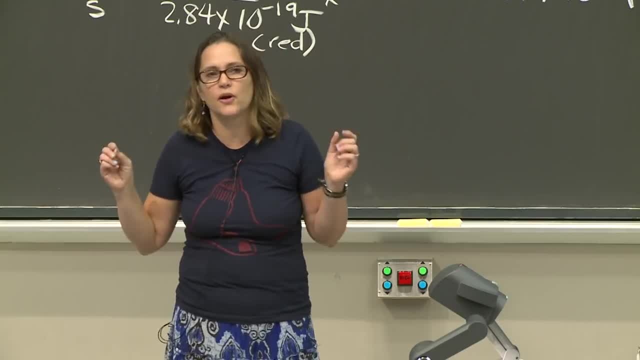 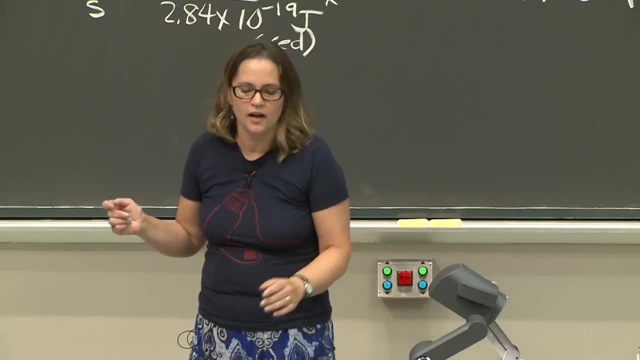 to systems that have a lot of atoms in them. So if you're interested in this area, you're not too late. You don't have to go back to the early 1900s. There's still a lot to do in this area. 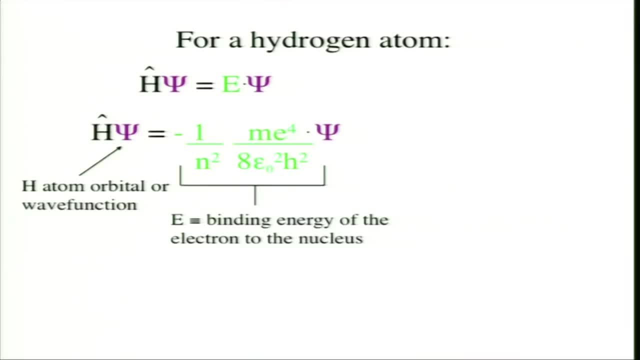 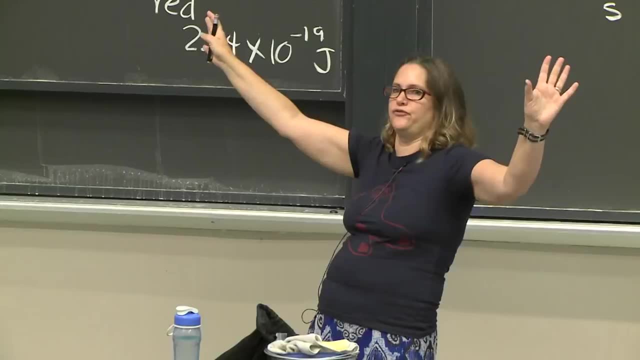 So, very briefly now, let's just look at the structure. We have the Schrodinger equation solved from the hydrogen atom, So we'll go back to understanding quantum mechanical analysis of photosynthesis. Amazing, Don't understand how it works. That would be great if we did. 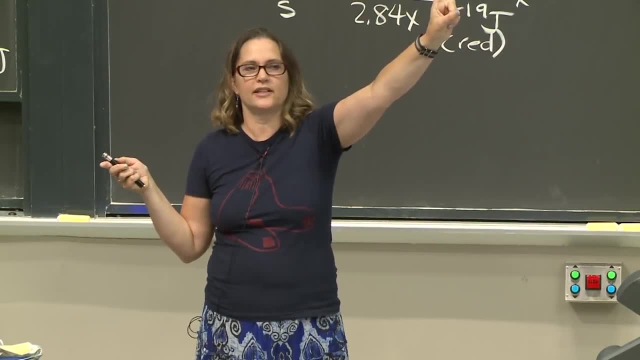 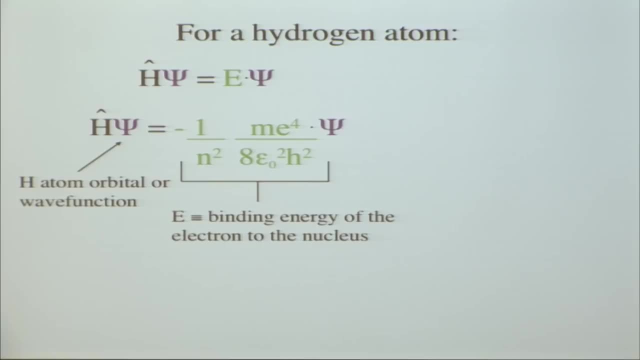 That would really solve a lot of energy problems. But we'll just go to hydrogen atom, one electron back. So if you solve the Schrodinger equation for this- and I think I did this in college, not in freshman chemistry but somewhere along the line- 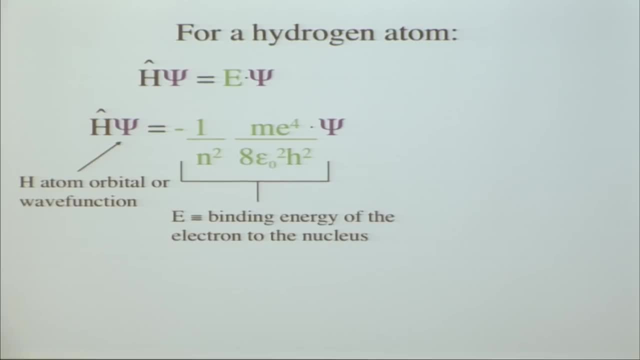 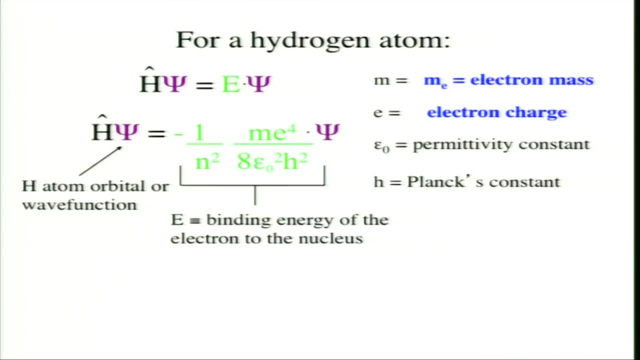 you'll come up with this term. So again, this is the binding energy. We just want to know about how we're going to solve this. So the electron is being held by the nucleus And there are some terms in here. We have the electron's mass. 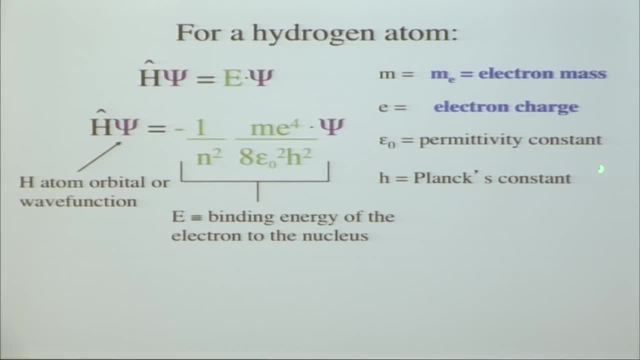 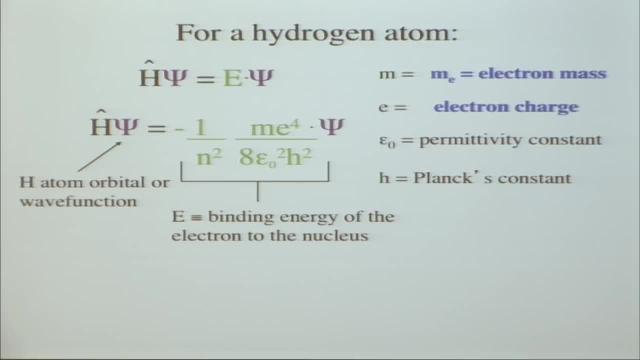 That's a constant. We can simplify that And we will. And that is the Ryeburg's constant: 2.18 times 10 to the minus 18th joules. So now it doesn't look quite as scary. We can just substitute this by Rh. 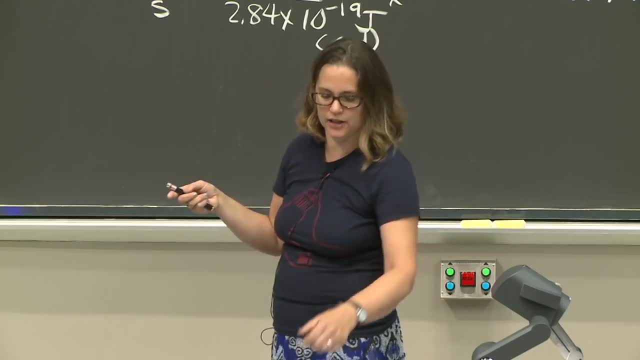 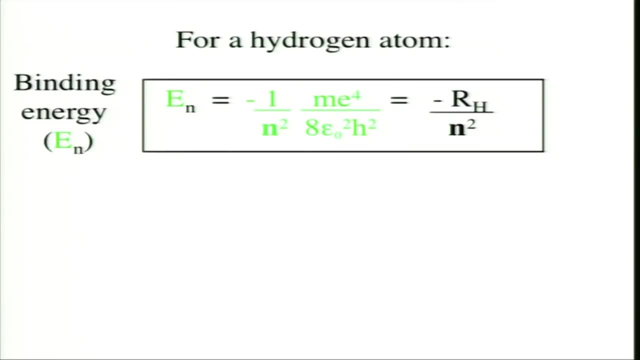 That makes us feel a lot better. It's one number that will be given on the equation sheet, so we don't even have to remember it. And now we can rewrite this in terms of the binding energy. So again, the binding energy. this is a constant. 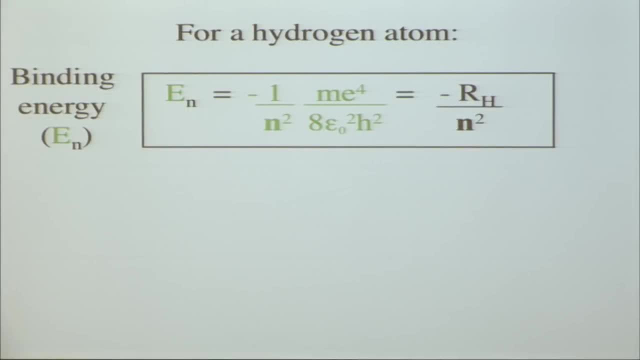 So now this turns into minus Rh over n. That's a constant, That's a constant, That's a constant. So that's n squared And n. what is n? n is a positive integer: 1,, 2,, 3, up to affinity. 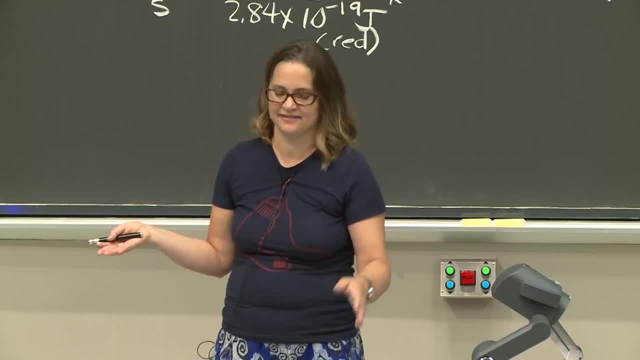 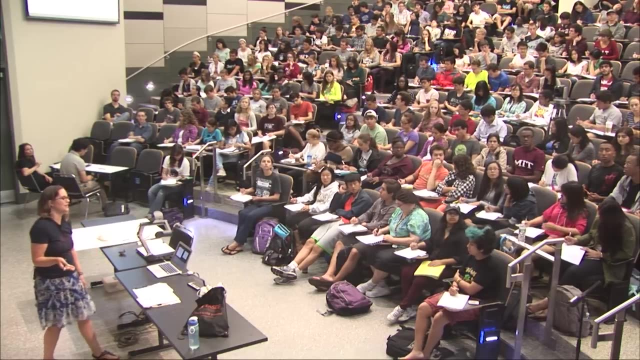 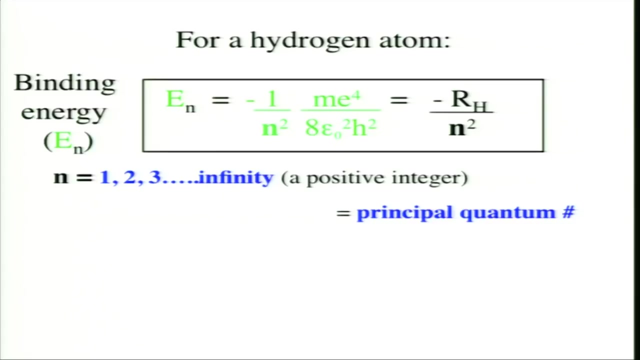 And what's its name? What is n? Can you yell it out? Some of you know, Yeah, principal quantum number. That's right. So the principal quantum number comes out of the Schrodinger equation, and that's how we can think about it. 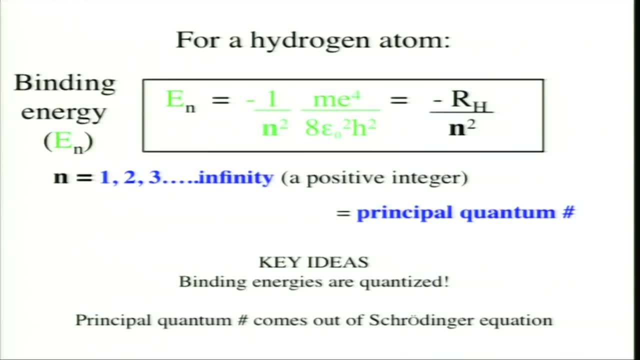 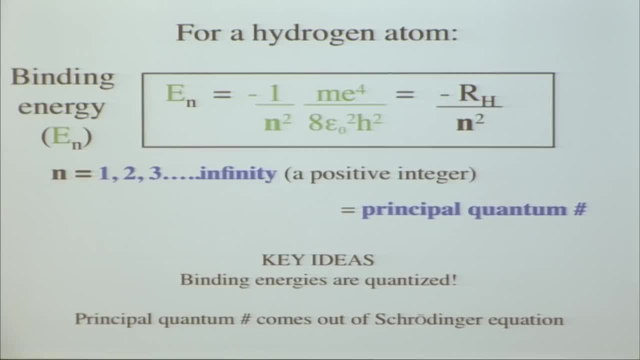 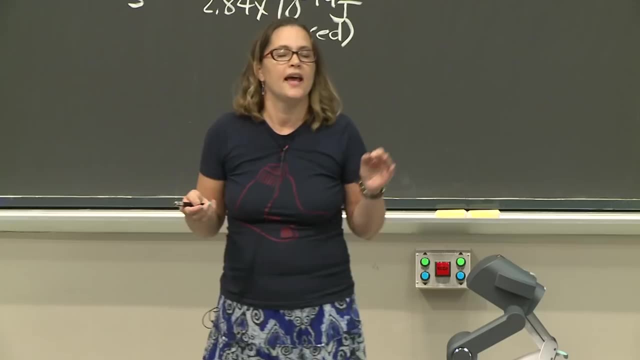 And again, here are these ideas. The binding energies are quantized. This is a constant over here. So the principal quantum number comes out of the Schrodinger equation. So now, next time, we're going to think more about the Riber constant and we're 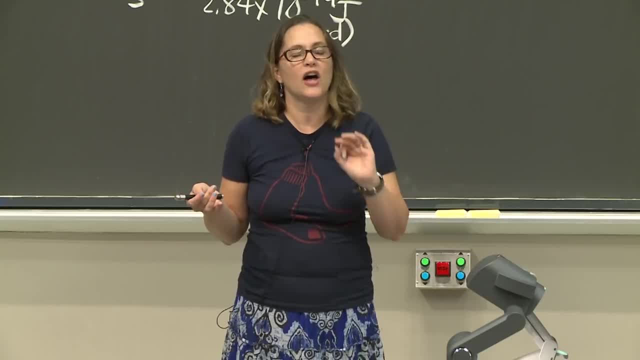 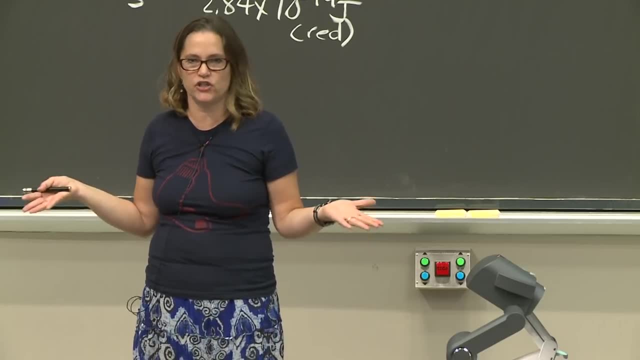 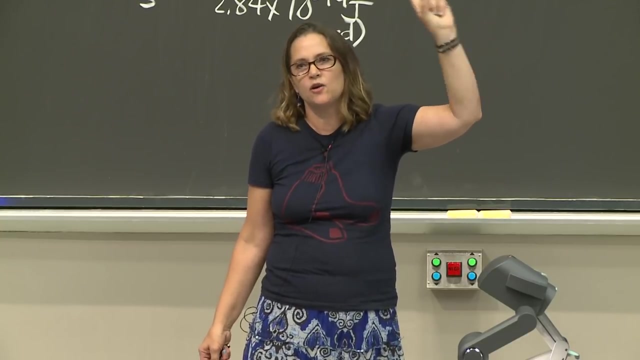 going to do a demonstration next Friday of the hydrogen atom spectrum to show that the Schrodinger equation, in fact, can explain binding energies. So that's on Friday and that's our first clicker competition. So come, be ready with your clickers.